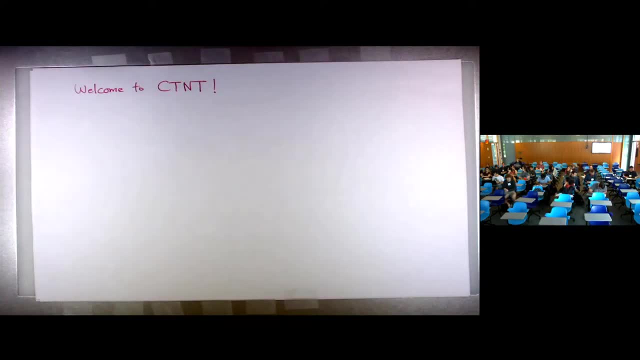 Okay, good, Good morning everyone. Welcome to Kaneka's summer school in number theory. My name is Liang Xiao. I'll be giving a series of lectures on algebraic number theory, which is kind of a if you've learned it before. it's going to be kind of a review of what 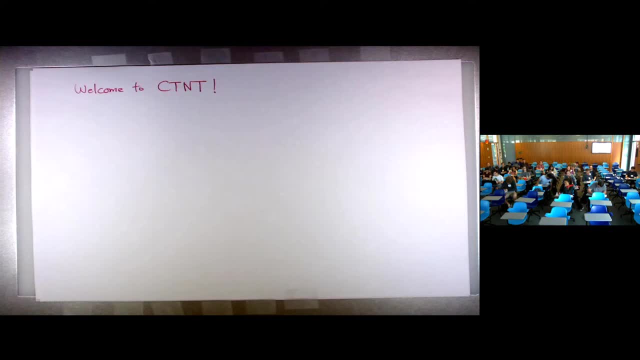 we have learned. If you haven't seen it before, well, you can, I guess, I hope, to give you some sort of a sketch of what's going to happen. So the idea is somehow to summarize probably a semester-long course into a four-hour-long course. We'll see how that goes. Well, if 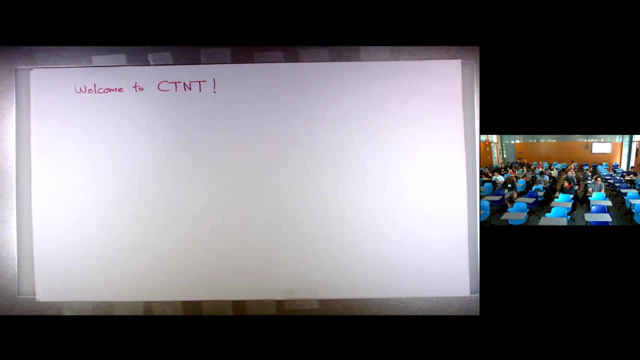 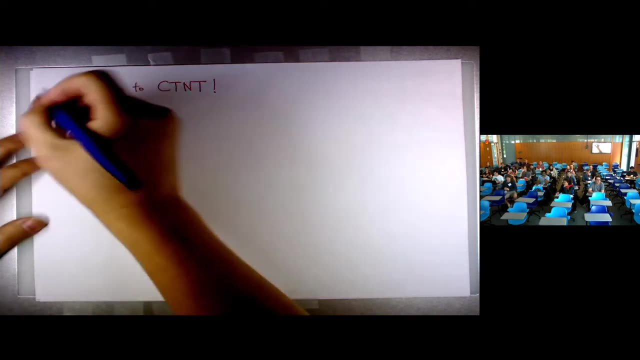 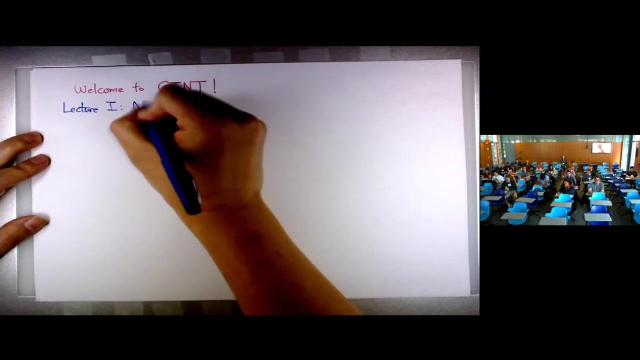 you have any questions at any time, just raise your hand or just say it out. I won't be able to kind of see you very well. So yeah, and feel free to ask me questions. So the first lecture, we're going to just somehow talk about the very basic number field By 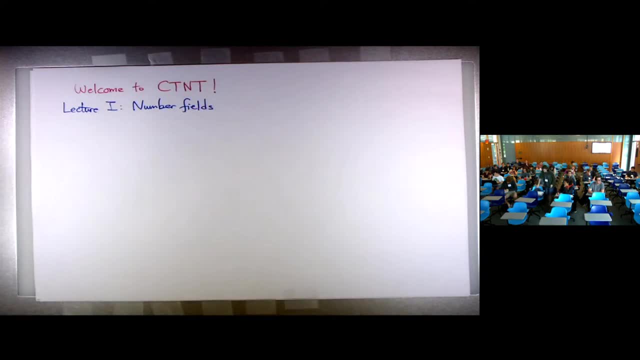 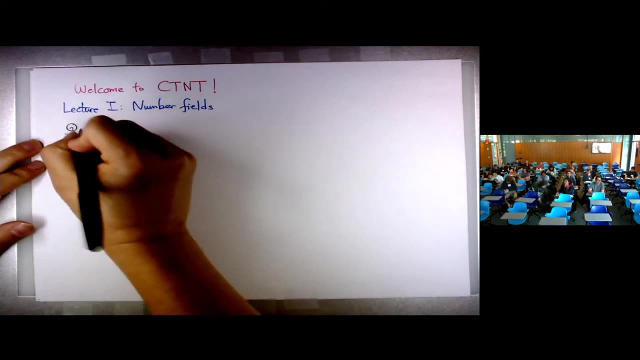 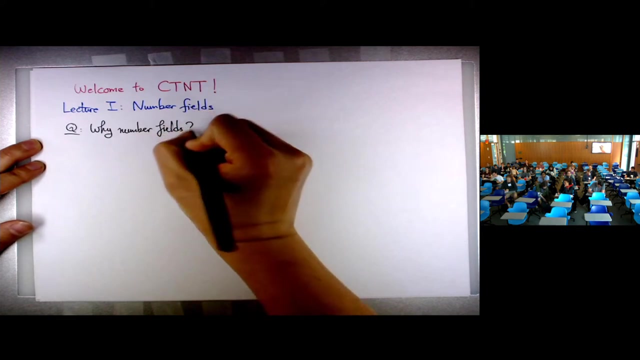 number field. I I mean, I find that an extension of the rational field. So let me, before anything, let me sort of explain why we want to look at number fields. Why do we care? I mean for a lot of people like I mean, somehow, at the end of the day, we care about rational numbers. 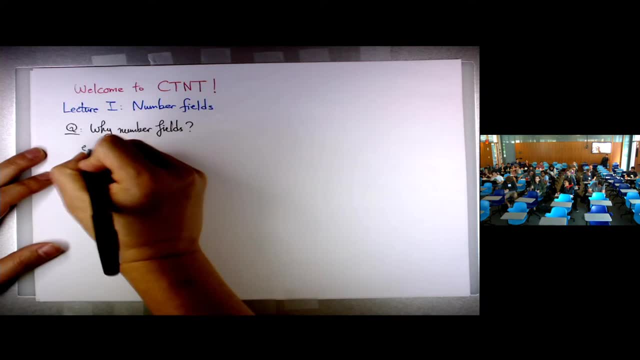 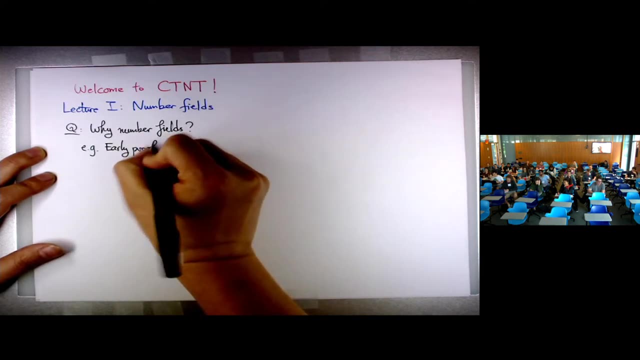 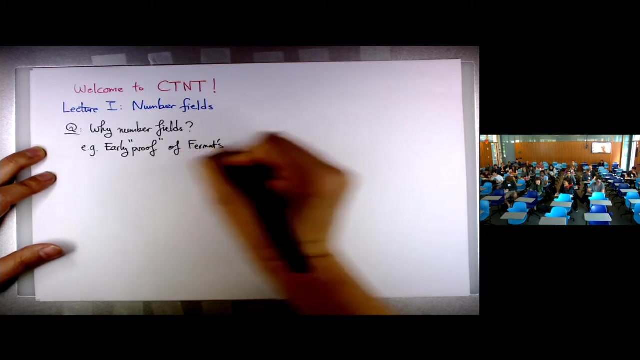 you know integers. So here I'll give you one reason. I have many reasons, but here's maybe one reason I think that this comes from. I'll explain that. it comes from an early proof- Well proof, not quite a proof- of Fermat's last name. So what that is is you want to show that. 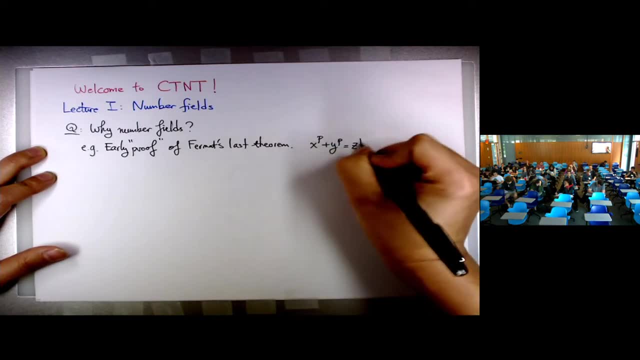 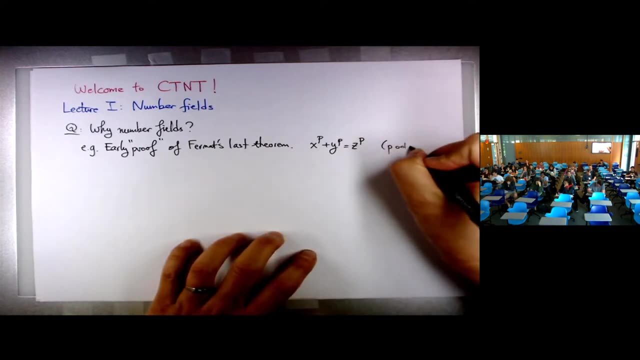 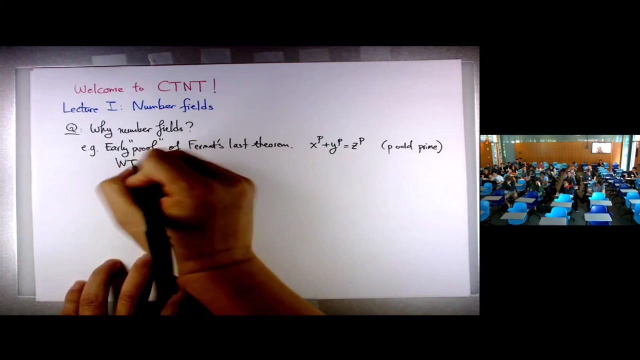 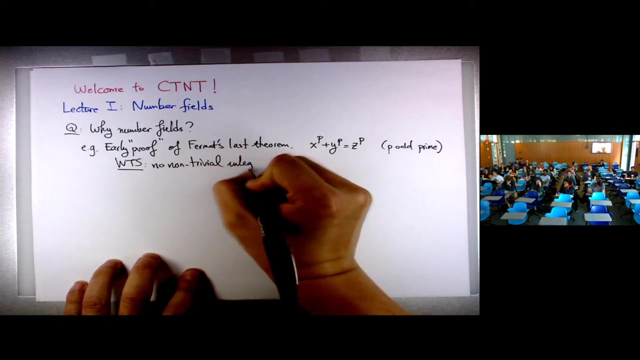 you have this Fermat's equation: x to the p, y plus y to the p equals b to the p, where p is the odd prime. You want to show that. you want to show no non-trivial integer assumptions. So that was. 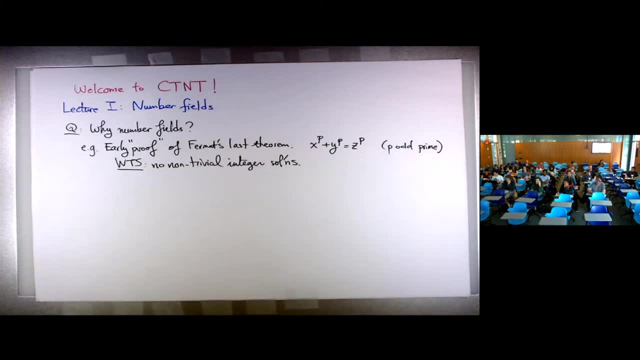 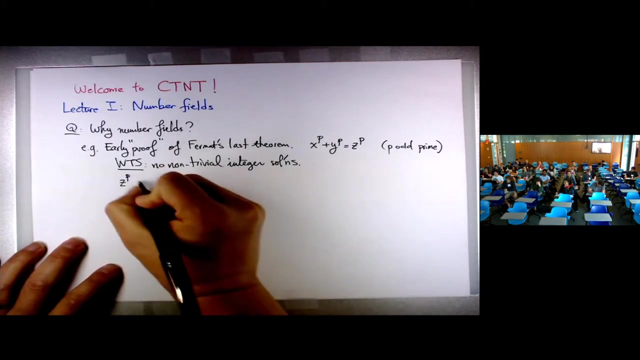 Fermat's last theorem, And of course this was proven by a very, extremely difficult method, a very highly technical method, But there's something that was known like over a hundred years ago. You can do the following: You have z to the p. Let's write this, because p is an odd number, so you can write x to. 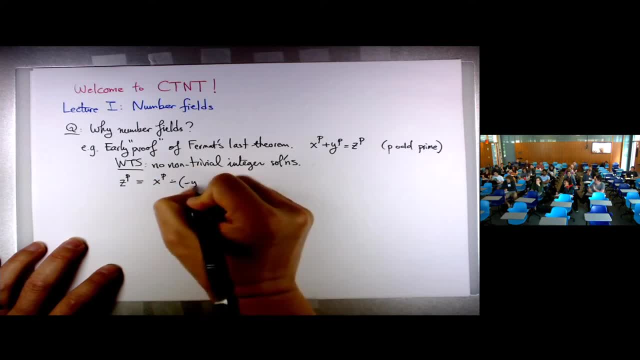 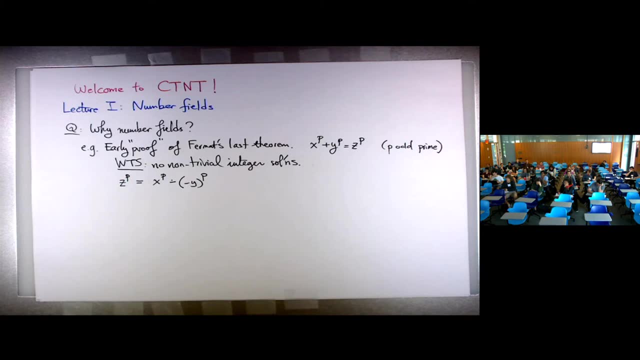 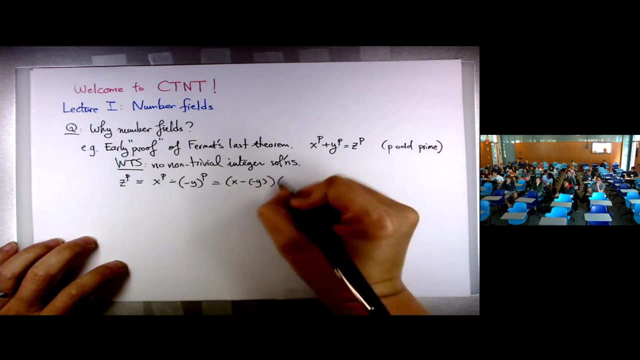 the p plus y to the p, as x minus negative y to the p. And then, just like you factor x squared minus y squared, you have x to the p minus something to the pth power. You can write it as x minus negative y times, x minus p through unity minus y and so on, to x minus. 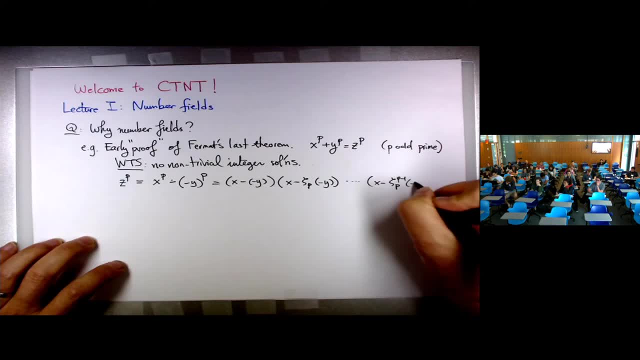 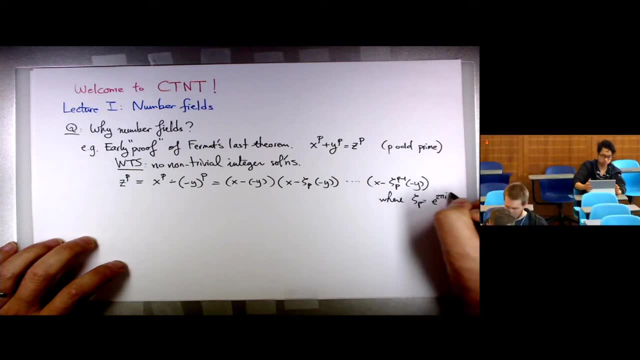 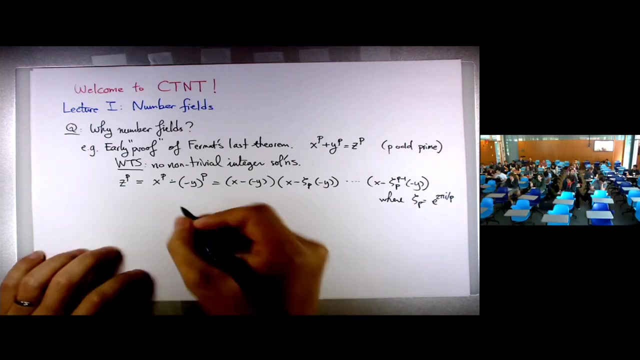 z to the p, To the p minus 1, where theta v is e to the 2, pi i over p. Just like you factor x squared minus y squared, you have x plus y, x minus y. You have this factorization And let's 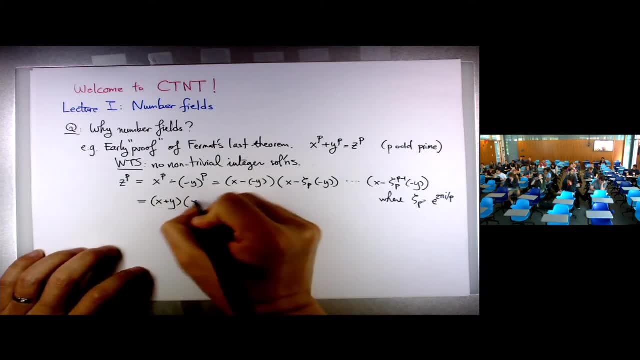 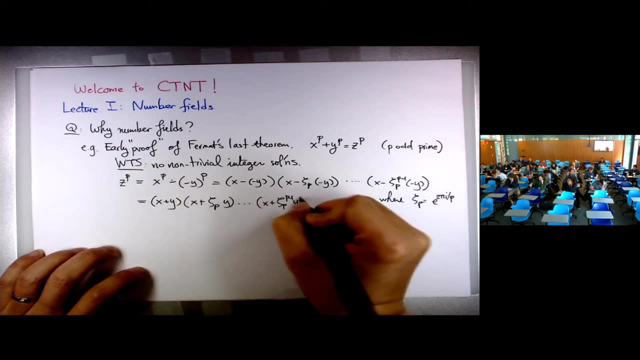 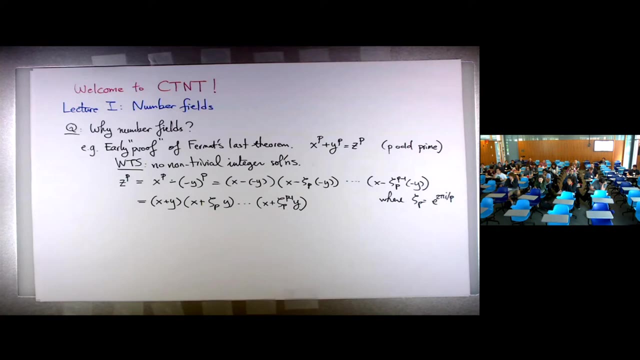 rewrite this. I guess it's traditional and people like to write it as this. Okay, So now we're going to solve this equation with x, y, z in the integers. So here's some sort of relatively- let's make some sort of naive observation to see why this helps. So 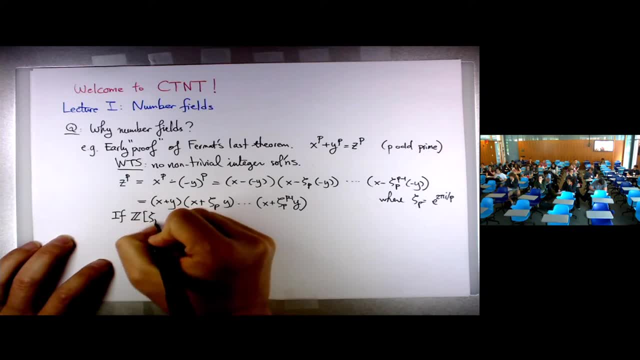 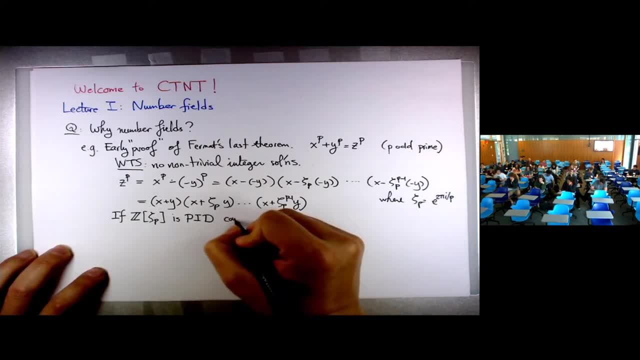 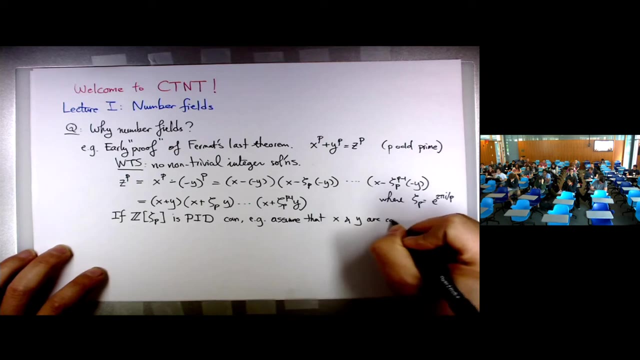 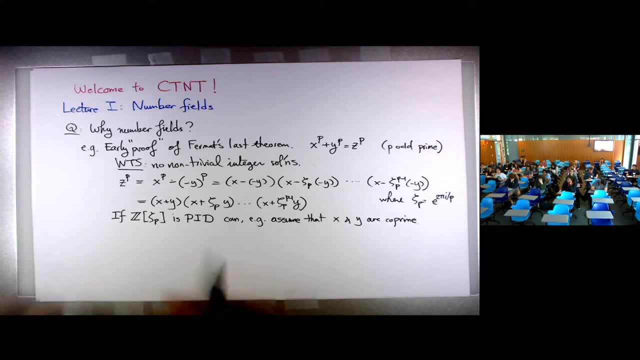 prime factor And after that you see that this x plus y and this x plus z to the p y, they're very close. If you take the difference, like z to the p y, z to the p? y and z to the p, you can just write this And then, if you listed this as a greater 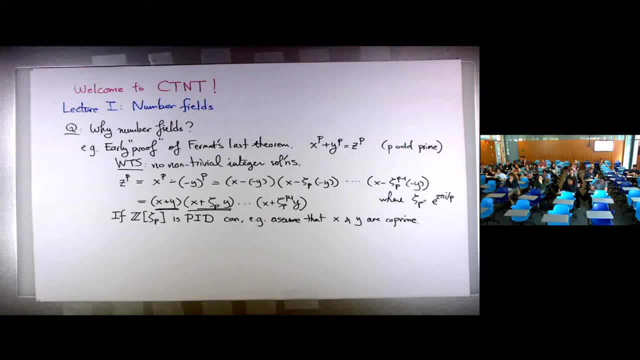 simple property, you're not going to be able to do it. That's why we'll do this faster. minus 1 times y, Because x and y are co-prime, you would expect that this x plus t and x plus theta, p, y are. let me say: 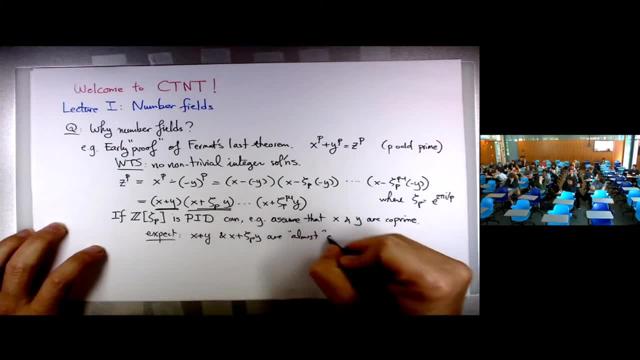 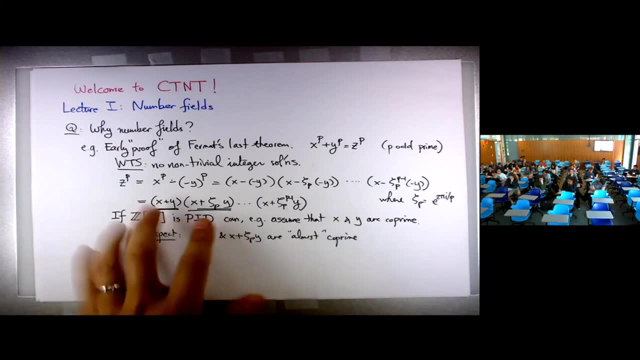 almost co-prime. They're not quite co-prime right away because they remind me of a small factor of theta p minus 1. But except that factor they're almost co-prime And therefore you have p factors of things. 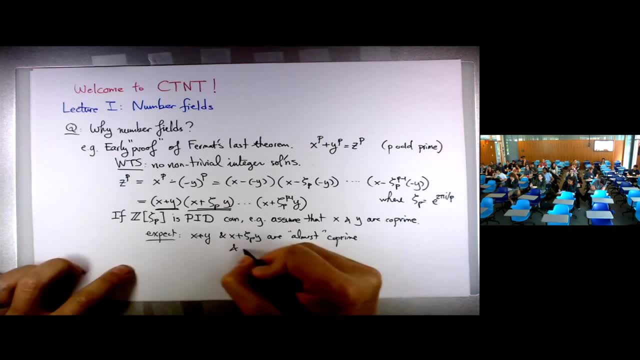 which are co-prime to each other And hence are sometimes almost p power, p power or something. So that's something somewhat very rare to happen. If you have two numbers, their sum is a p power and then their x plus theta p, y is also a p power. 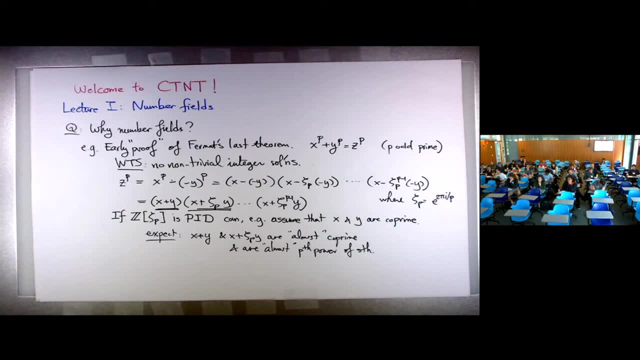 That rarely happens, And so you can explore that fact To show that there's no solution to this. So of course, there's a lot of work to be done after that, But then of course, this gives you a way to approach this problem. 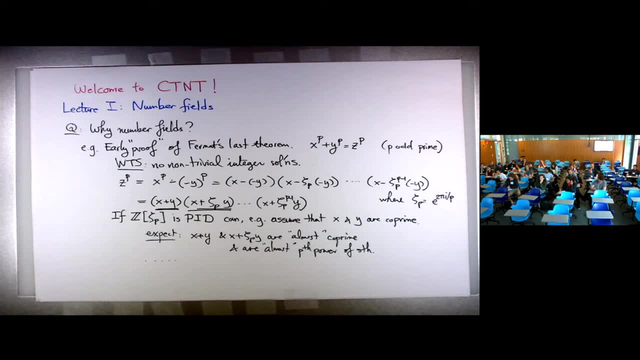 So the upshot I want to say, oh, maybe I should say this: So, Coomer, using this kind of method- Coomer, that's centuries ago- shows that this proof works. Not only this. z-adjoint theta p is p-id. 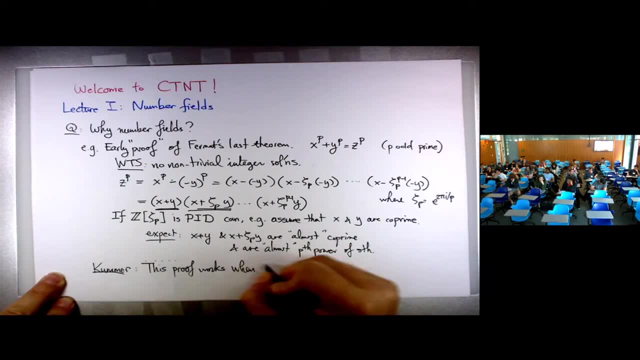 but also when this ring is, let me say, almost a p-id. I'll come back to this later to talk about what really condition is. So that's why, I guess, triggered the study of the algebraic number theory and algebraic number theory. 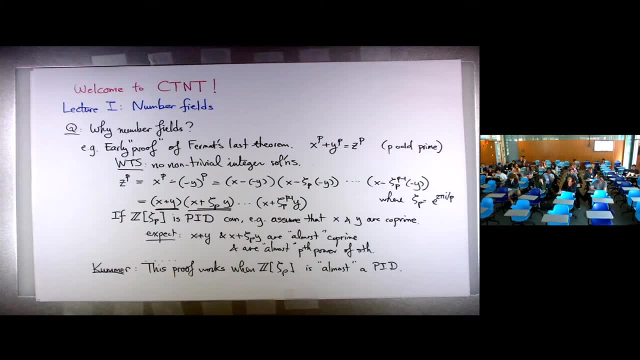 And I want to say that also. I want to make a remark that Coomer used this method to prove this for all all prime p Less than 100, except for three primes. So he proved a lot of this for my theorem actually. 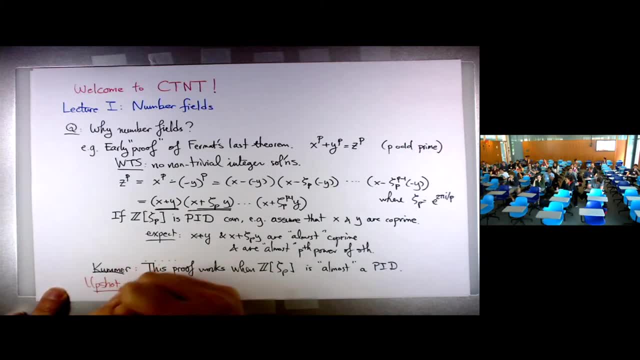 So here's the upshot on a conclude by conclude at the end of this example, which is that studying bigger fields help understand how to solve this Delphi-Tang equation over either z or q. So even if the original equation, like this one x to the p. 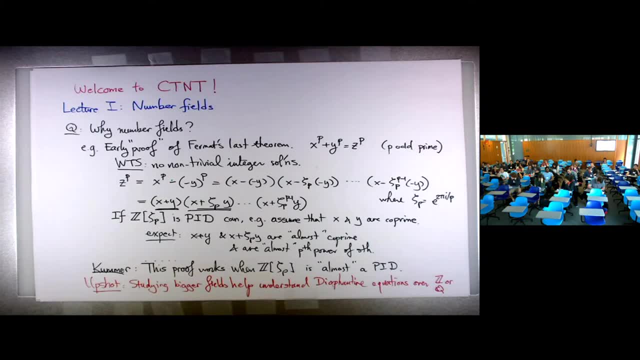 plus y to the p, because z to the p is written. you're asking about real, excuse me. I'm asking about integer solutions or rational solutions, But the solution somehow sometimes involves understanding this in a bigger field, And it really helps if you go to a bigger field. 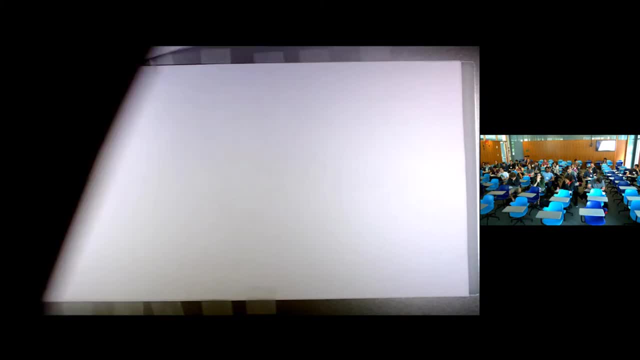 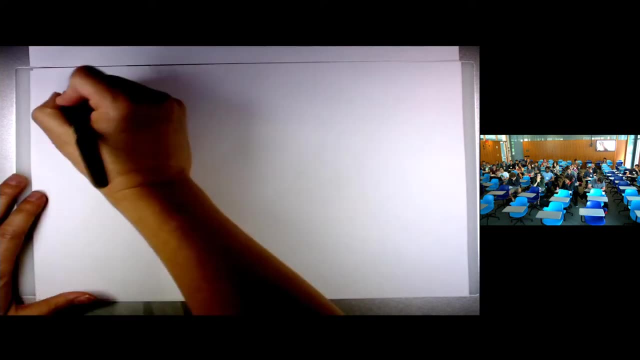 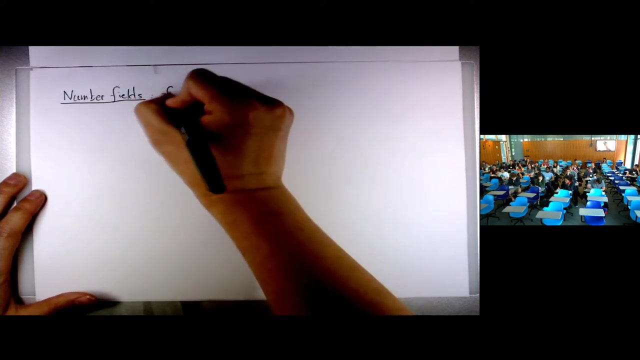 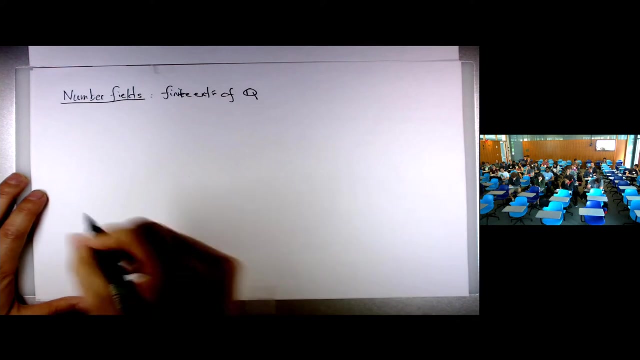 So that's why we want to talk about number fields. So let's get down to study number fields. This, by definition, is just a finite extension. So this is f of q, So usually people write this as f over q. 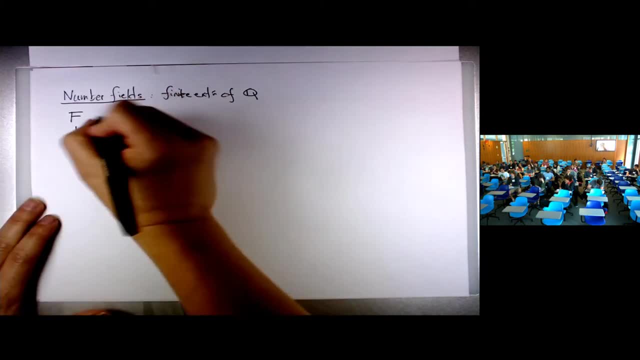 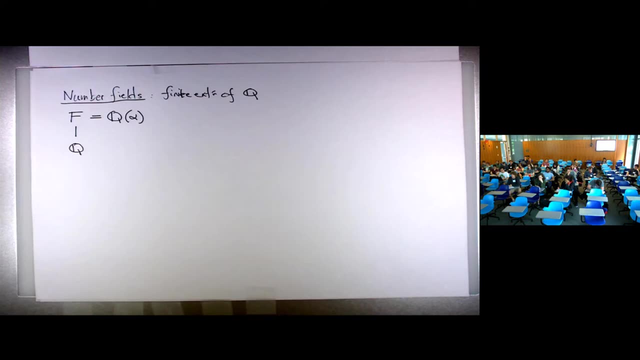 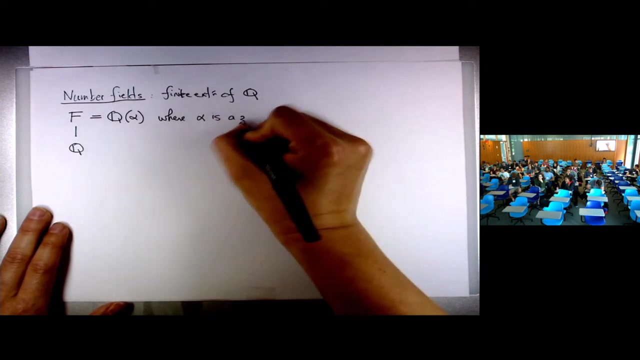 That's the standard way of writing this By the. there's a primitive element theorem that if you have a finite extension of a field of 0, it's always generated by one element. So this: where alpha is a 0 of an irreducible 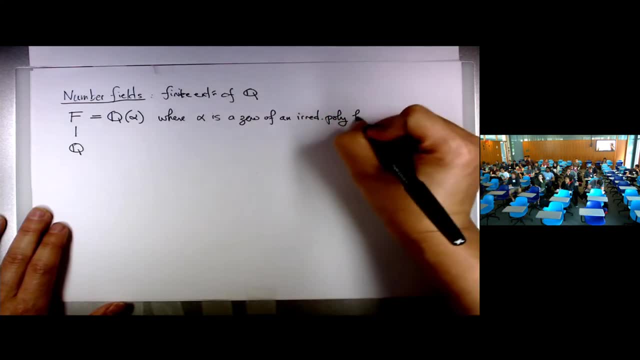 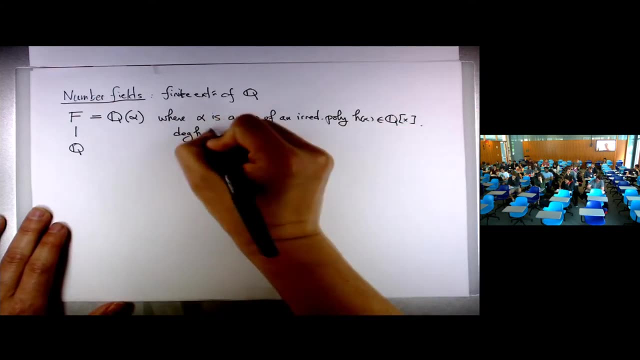 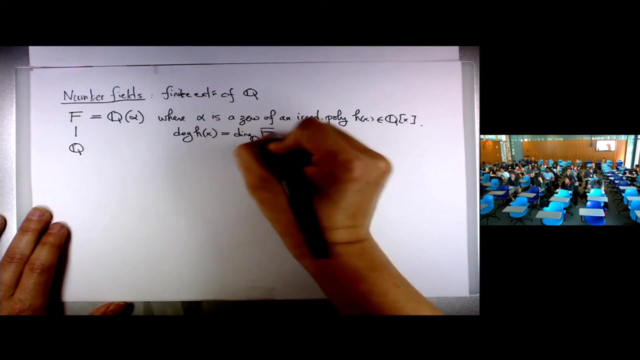 And here's the final. I call it hx And q will join x. So the degree of hx is well the same as the dimension of this f as a q vector space. Sometimes I write this: I write this as f called q. 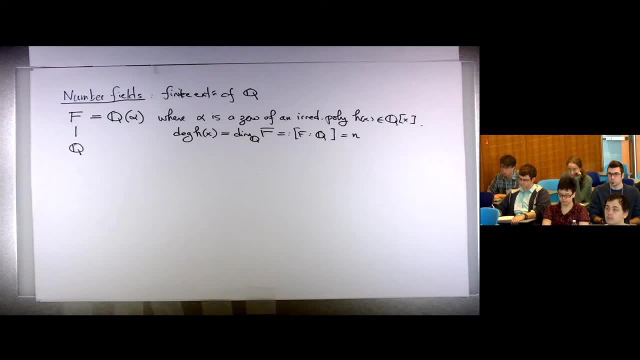 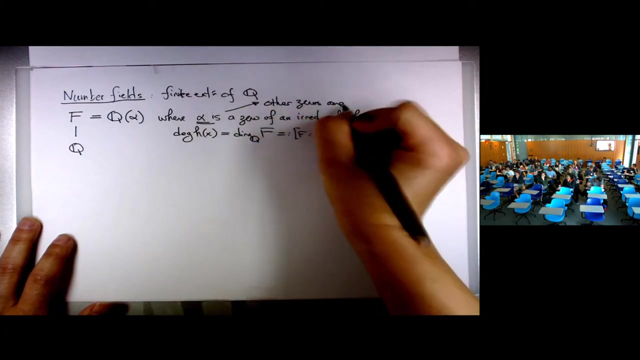 That's. we're going to use n to denote that degree of extension And I have this alpha to be the 0 of this irreducible polynomials. Let me write other 0's as All right, All those 0's maybe. 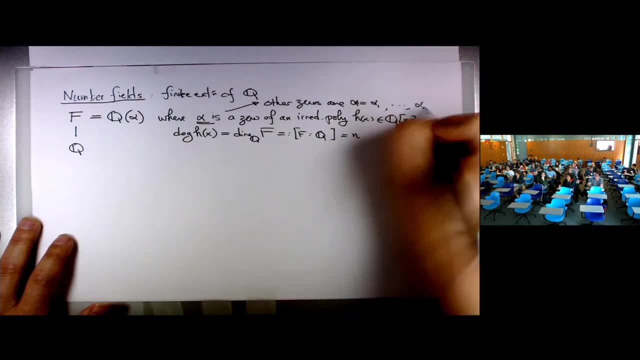 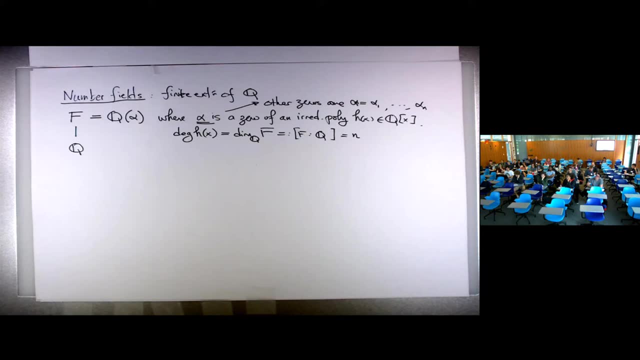 Maybe I include alpha here. It'll be alpha 1 through alpha n. OK, So now I'm going to think of this. So the idea is I don't want to think of alpha as a actual complex number. So I'm saying I want to think of it. 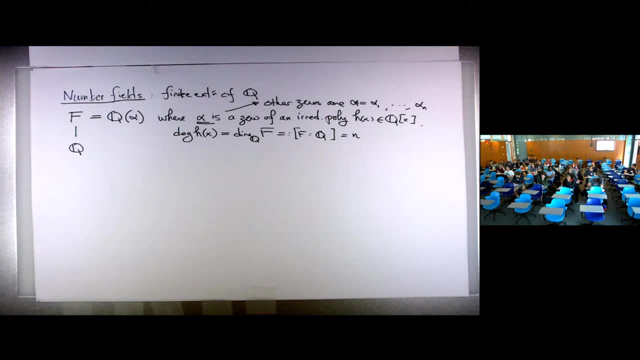 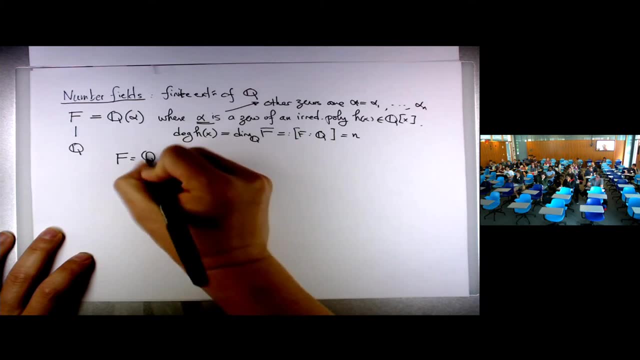 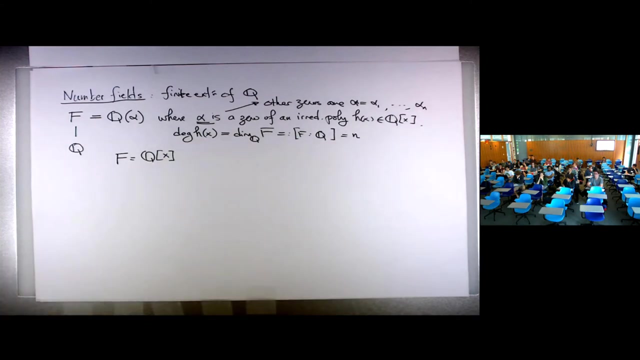 as alpha, as just the 0 of this polynomial. In some sense, I want to think of my f. Instead of joining some concrete number alpha, I want to just join a abstract variable, x, except that I set h of x to be 0.. 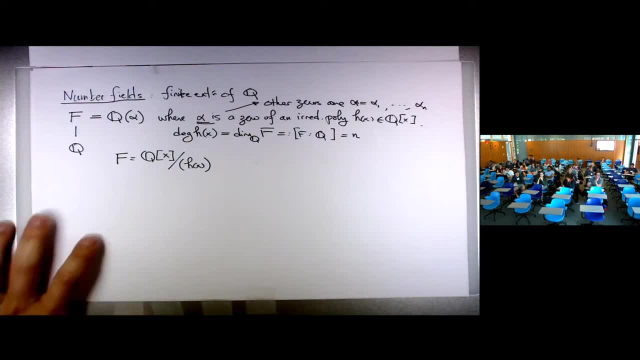 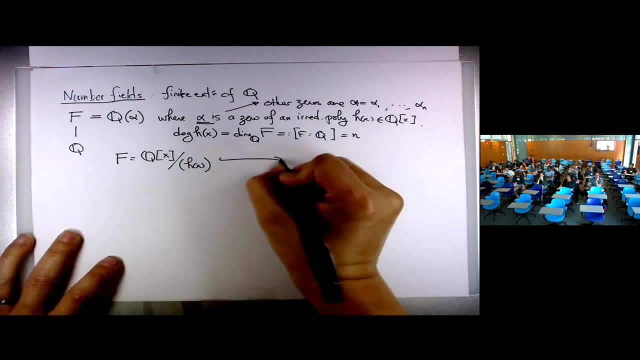 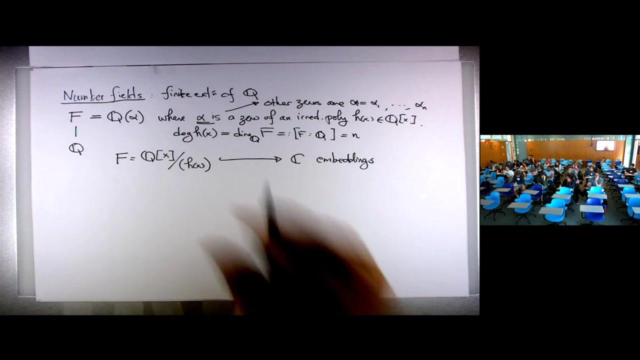 So this is some sort of abstract number here. But whenever we want to talk about, you know, we want to relate to the reals of a complex, we talk about something called embeddings. So when we choose a way to embed this into C, 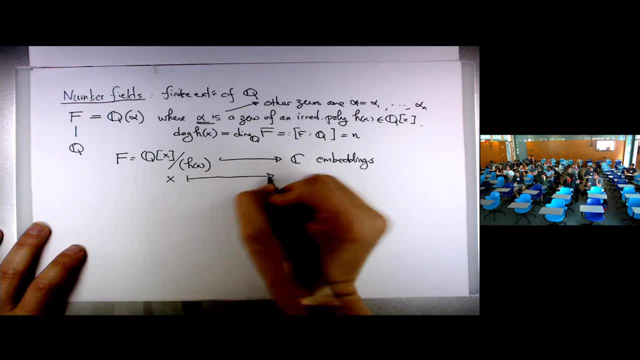 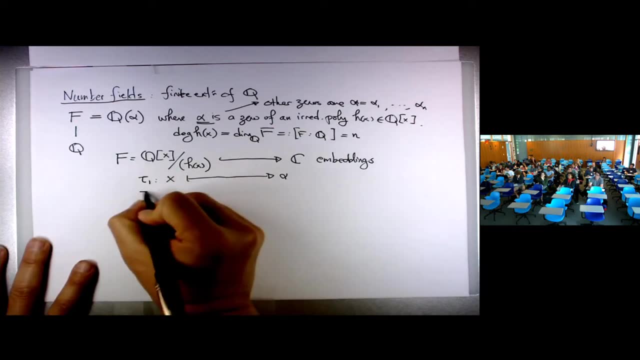 where I'm allowed to send this x to. somehow in the natural in our mind, I can send it to the alpha 0. So this is called, let me call it tau 1.. I can also send it to other 0's of the same polynomial. 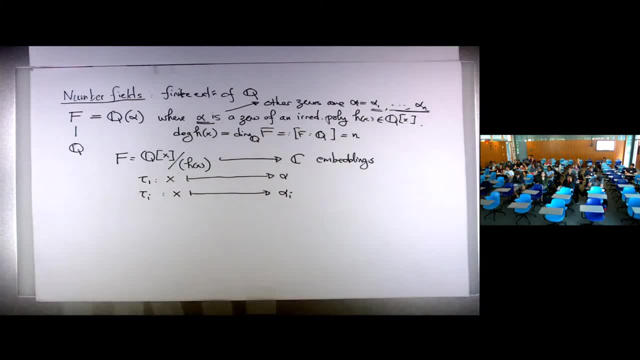 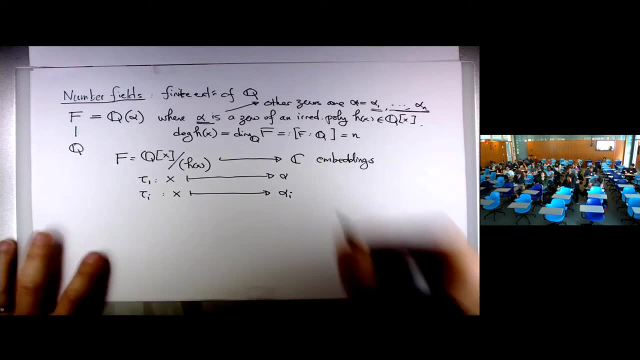 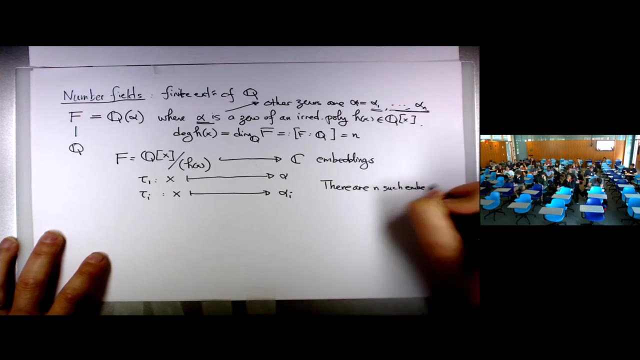 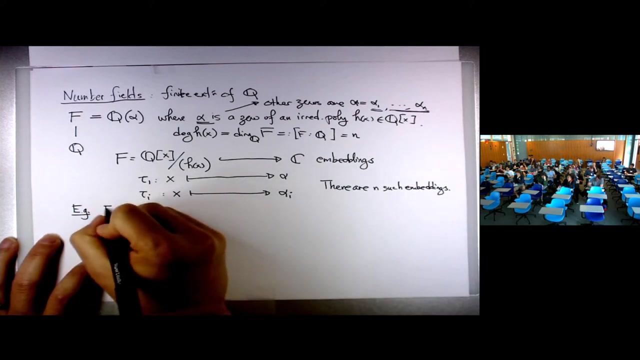 Alpha 1 and all the alpha i's, So they all form different embeddings of f in C, And there are precisely n such embeddings. Let me give you an example. So let's say f. I want to take it to be q of a joint. 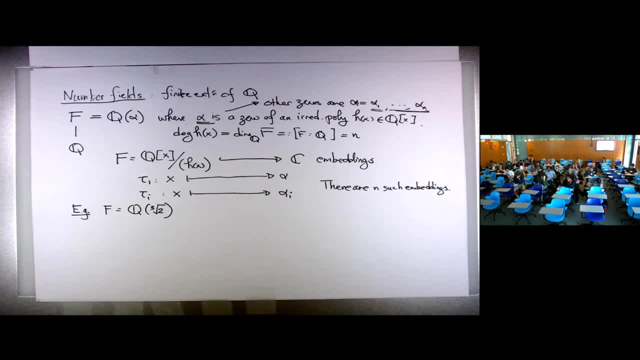 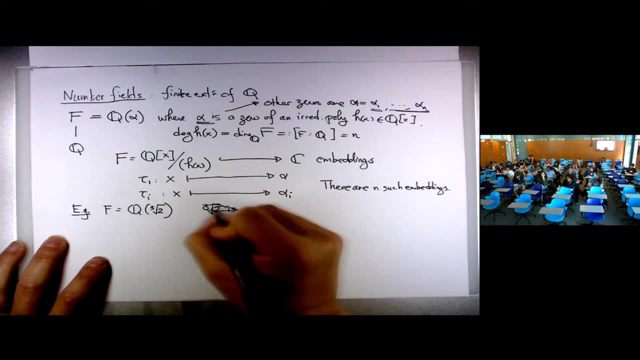 cube root of 2.. So this, of course, this is a 0.. I don't know. This is a 0 of x, cubed minus 2 equals 0, of course, Let me write real embedding. I'll explain what that means. 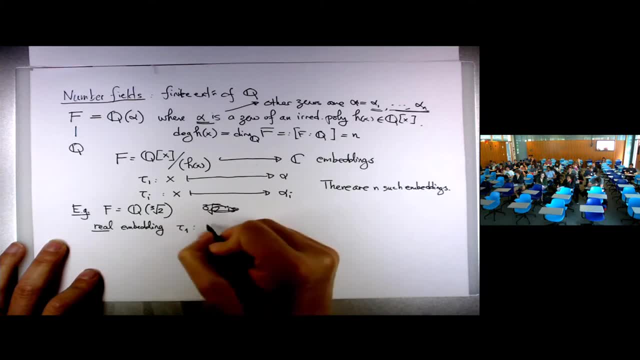 Real meaning. it's going to embed into the real number. So I'm going to write tau 1 of f into into C, But somehow the image will land in the reals. The way you want to send this is that I want to think of this again as qx over x cubed minus 2.. 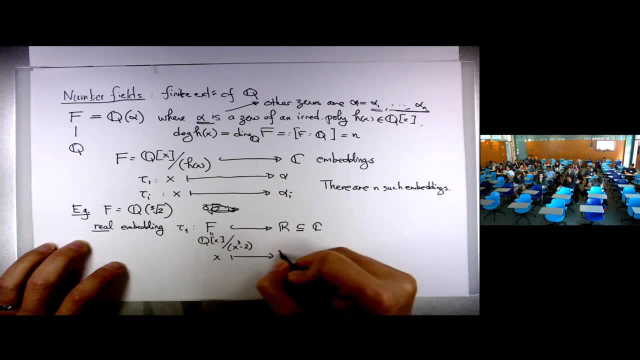 You want to send the x to the actual cube root of 2.. Right, You see that if you send x to cube root of 2, then the equality here- x cubed minus 2, will be automatically 0.. So, therefore, you have a map from this quotient. 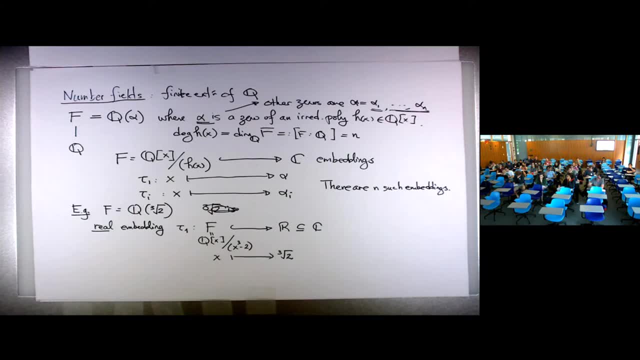 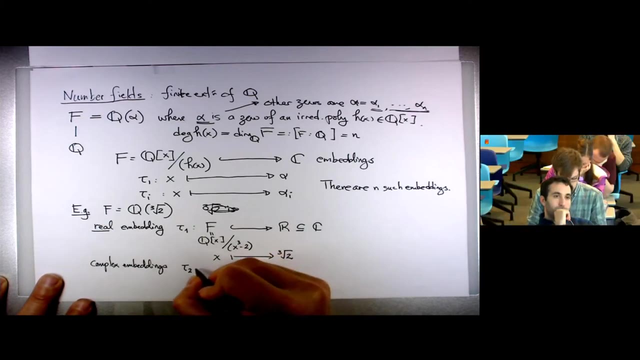 This quotient to R. That makes sense. Similarly, you have other embeddings. There are complex embeddings. Let me write tau 2.. OK, Tau 2, tau 3.. That's fine. Go from f to C And you think of this as q, right? 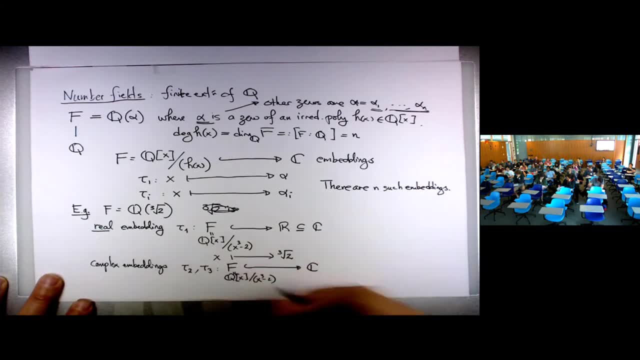 x over And then you think of this as q right x And then you want to send x to tau 1.. We'll send it to cube root of 2, times the third root of unity. You see, x cubed of 2 has three roots. 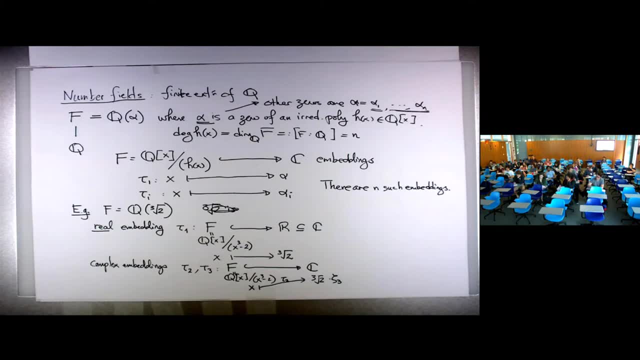 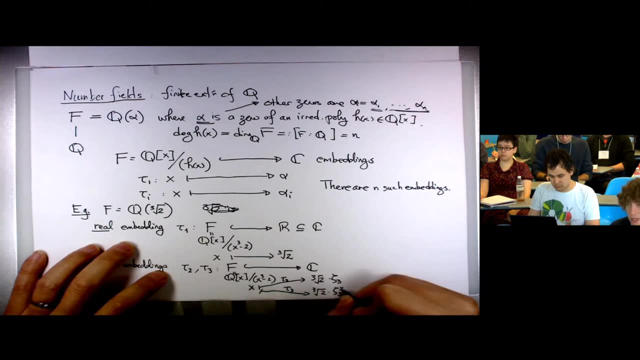 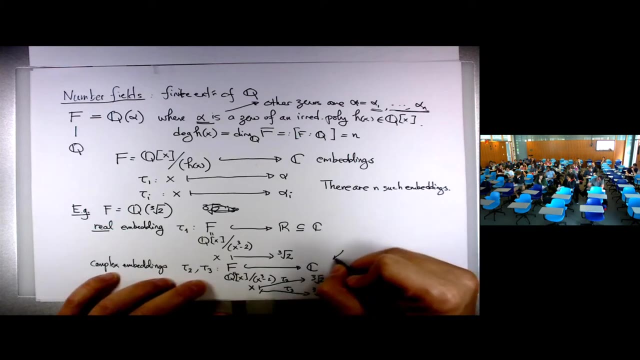 cube root of 2 and cube root of 2 times third root of unity, and then the other one. So, in other words, what I'm implicitly saying here is that if you join cube root of 2, and that's just the same as q. 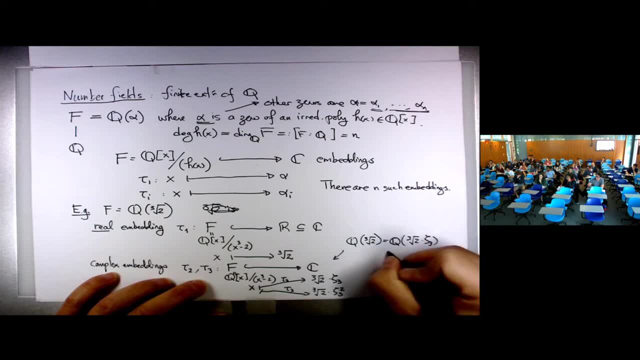 a joint, this times this, Or that's also the same as q a joint. the other roots, They're just different. They're somehow abstractly the same thing. That's how you're increasing different embeddings and realizing this field as tau 2 to C. 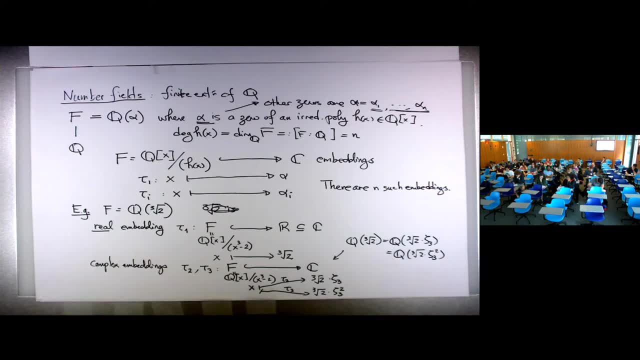 Right. And also I want to point out that, uh, because this theta 3 is negative, uh, minus 1, plus root of negative 3 over 2.. And uh, theta 3 squared is exactly the complex conjugate of that. 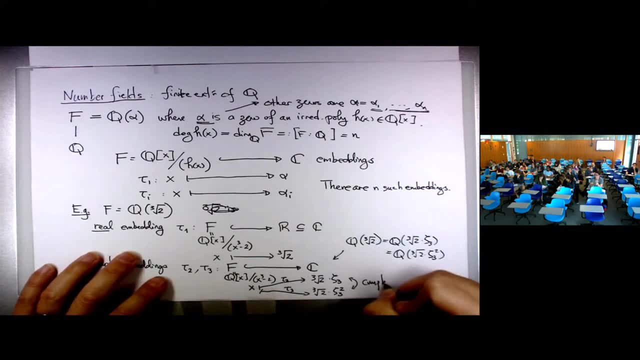 So these two are complex conjugate of each other. I want to point out- this is some sort of reflection of a general fact- that, given an arbitrary number field, you have some number of real embeddings and you have some complex embeddings, But the complex embeddings always come in pairs. 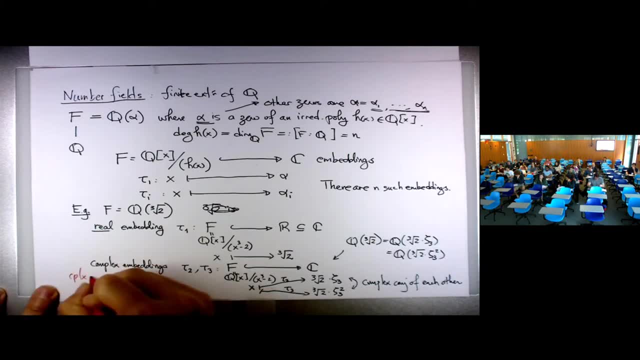 Let me just say that Complex embeddings always come in pairs, Because when you have a complex embedding you can further apply a complex conjugation. you have a different embedding, Okay, But altogether there are altogether n embeddings if the degree of f over q is n. 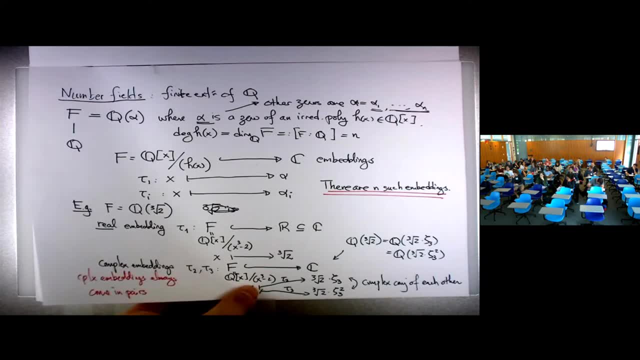 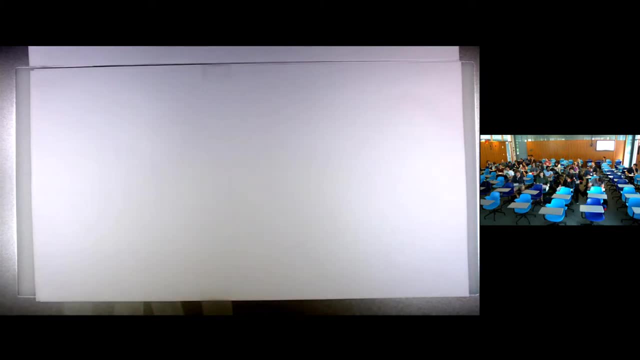 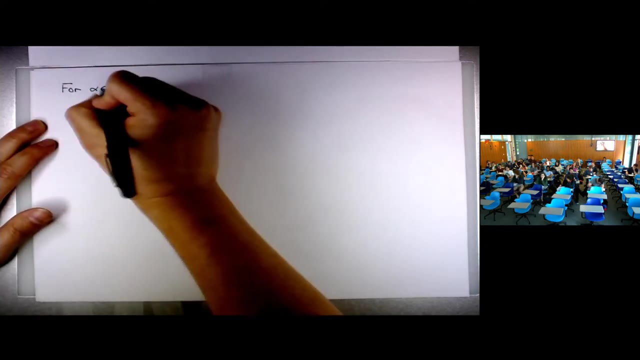 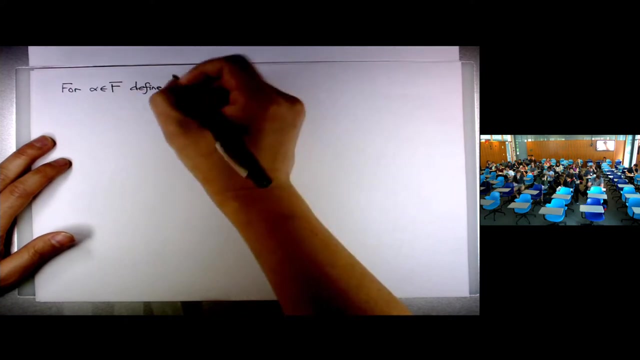 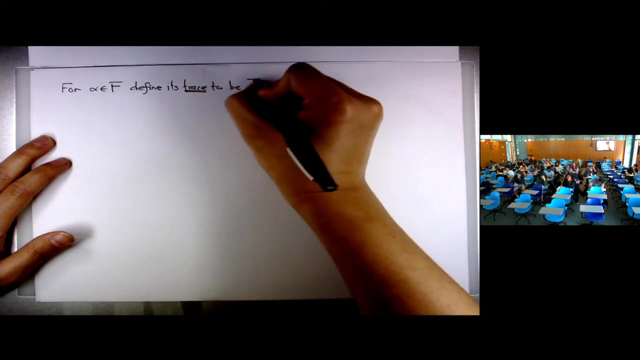 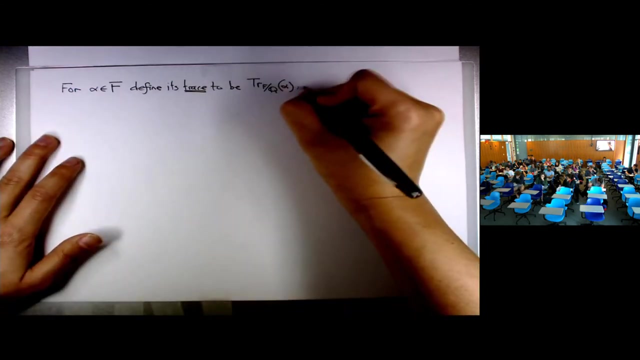 Are there any questions? So I'll talk about a very technical thing. I want to. for arpa in f, I want to define its choice to be. I'm going to write this choice of f over q of arpa to be the sum. 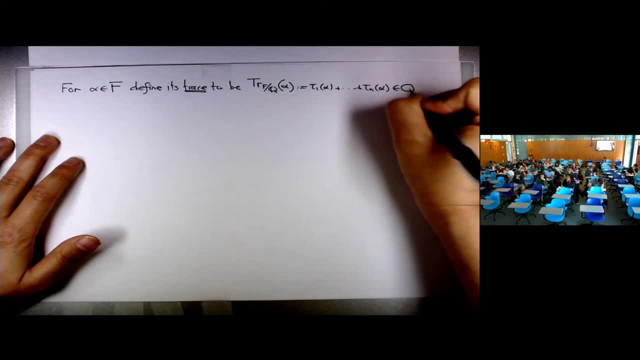 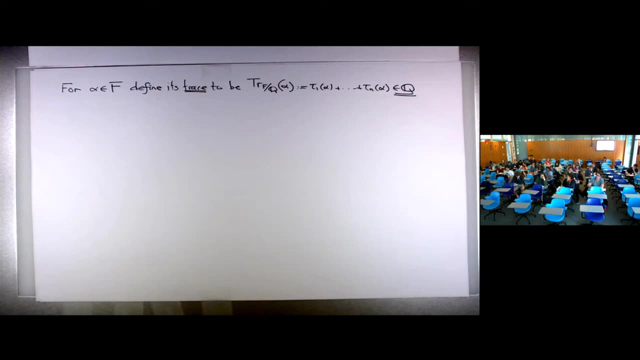 of all the embeddings, And it's not a trivial fact that if you sum all the embeddings of an element, you get actually get back to in q. So I have some exercise here. Oh, I should just tell you this: 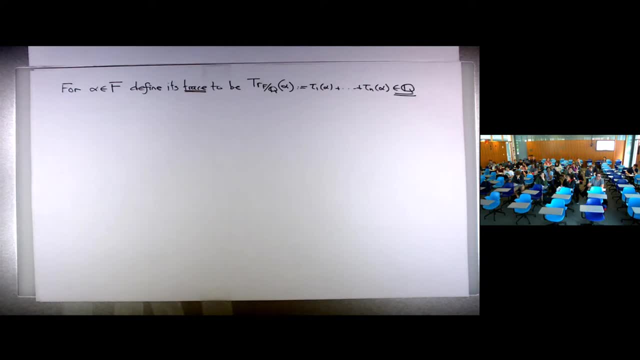 So I have some exercise printed out here. You can also find it online if you want to get it. later In that exercise I will tell you how to prove that the traces are actually in q. Similarly, I can define this norm to be: 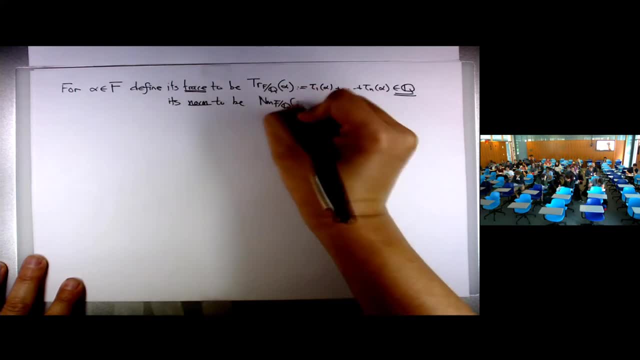 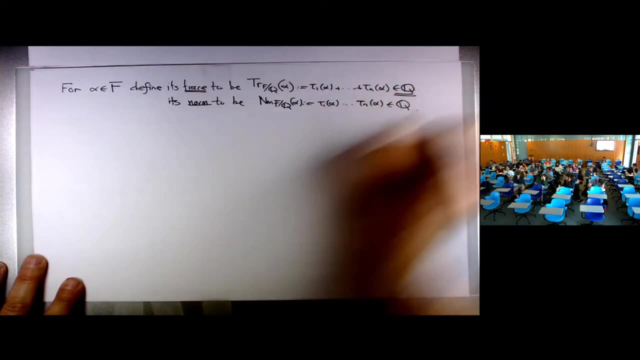 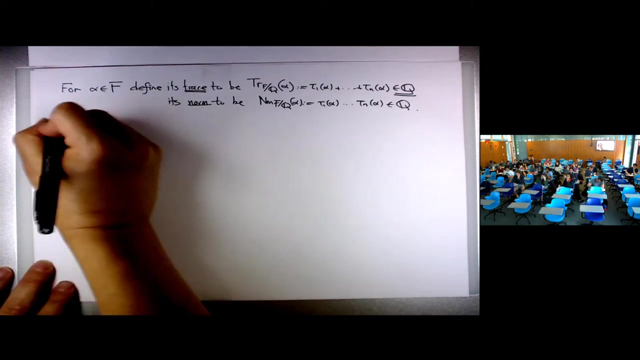 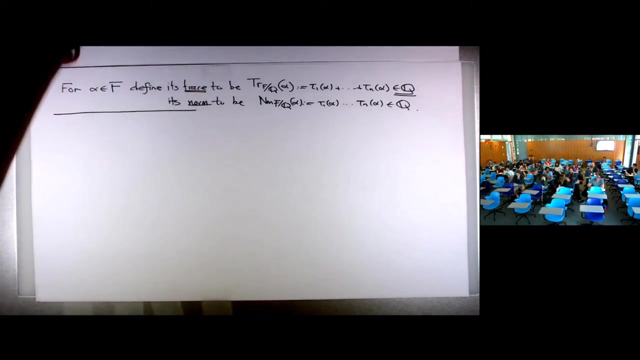 this: Instead of taking the sum, you take the product. Once again, this will be in q. Okay, So now this is all about the field. If you recall earlier, let me turn back this page a little bit, So. 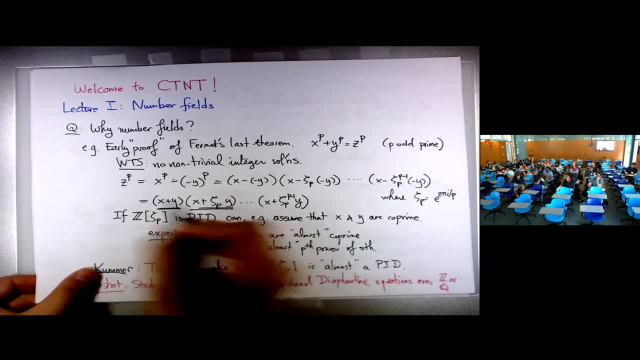 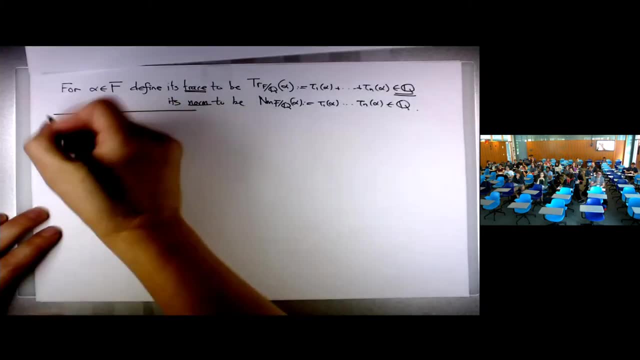 when we talk about this application in the last class. I'm really interested in this z-adjoint data p. It's not a field. This is somehow the ring associated to that, So this is something we call the ring domain here. 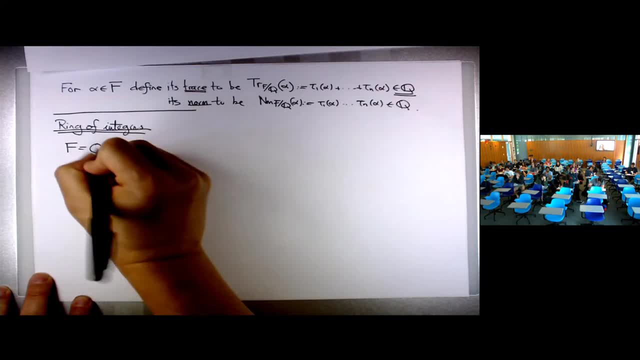 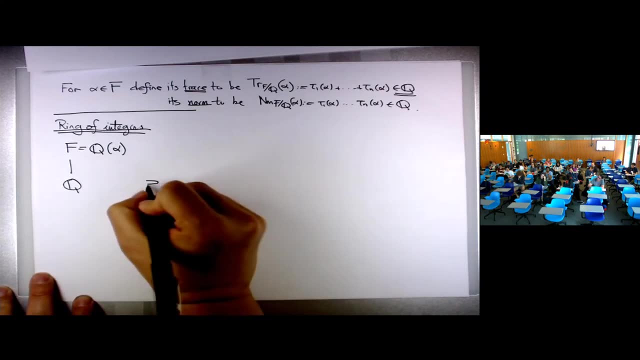 So basically, the idea is that now I have my field, f equals q, joint alpha as an extent of q. Okay, We know that inside of q are the integers. That's something we work with And now we want to understand. 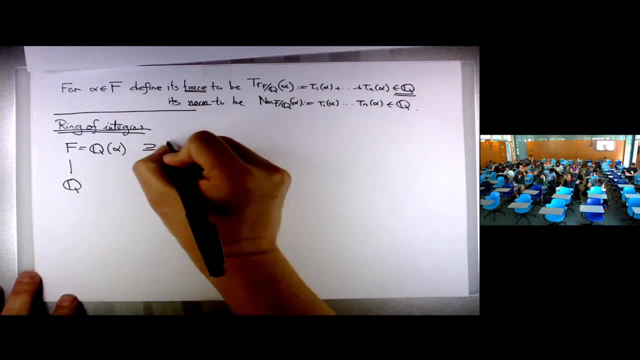 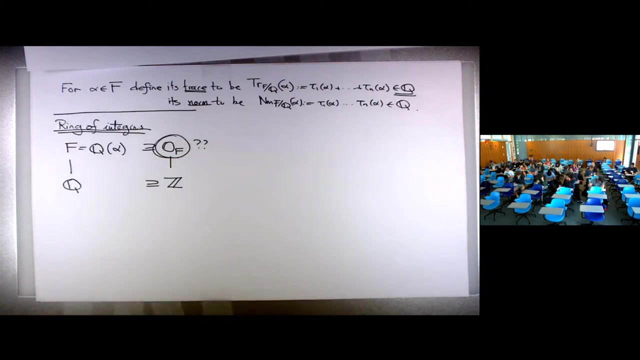 how to define this thing here, which is sort of the sort of ring of integers for a number of fields. Okay, That's what something I want to explain right now. So let me even say so, here's maybe a naive guess. 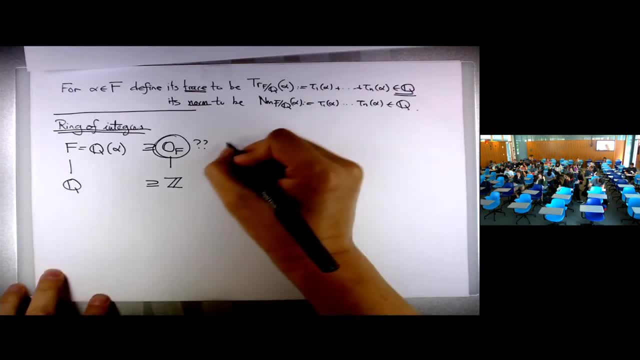 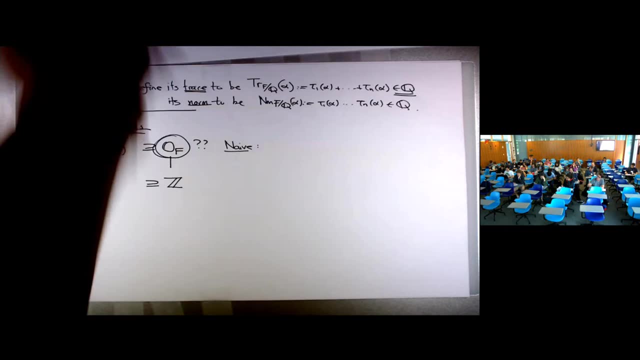 So you can, I mean you can start with this, So you can start with this. So this is an alpha, It's obvious. I mean I can just maybe look at the from my last term example, right, 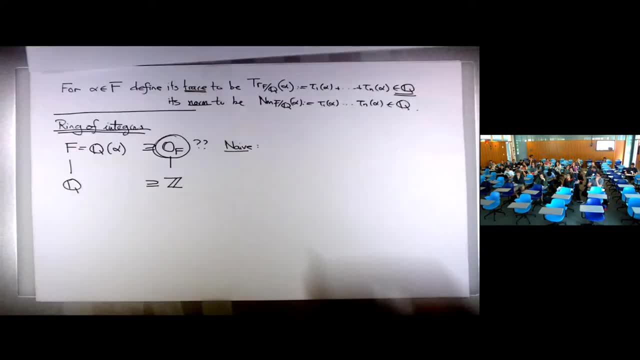 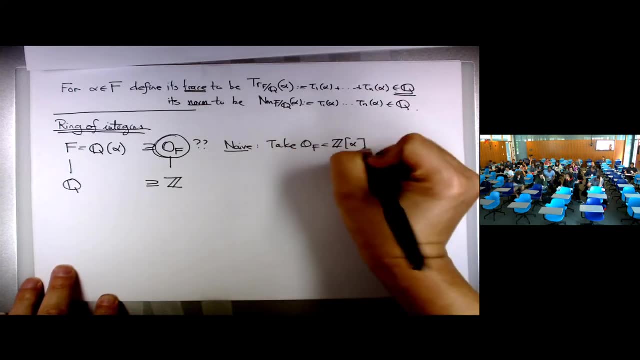 I mean, I start with a sort of adjoining, some zeta p. right, We can do this. Maybe I can just say: just take of equals z adjoined alpha, Well, well, there's a bit of a problem with this. 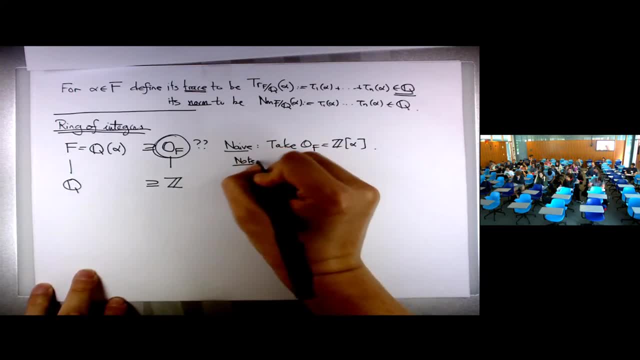 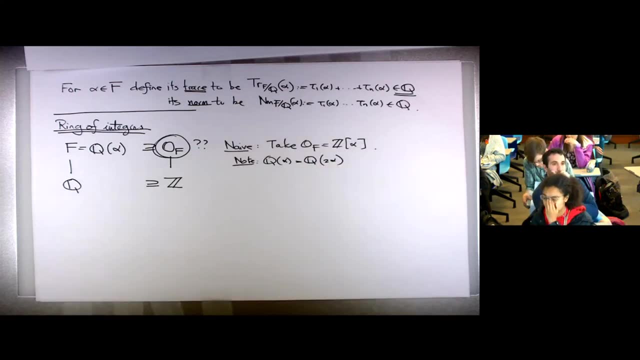 What's the problem? Well, you can say: okay, note that q alpha is the same as q 2 alpha. You can either join alpha or 2 alpha to the same q And you're gonna get the same. you're gonna get the same. 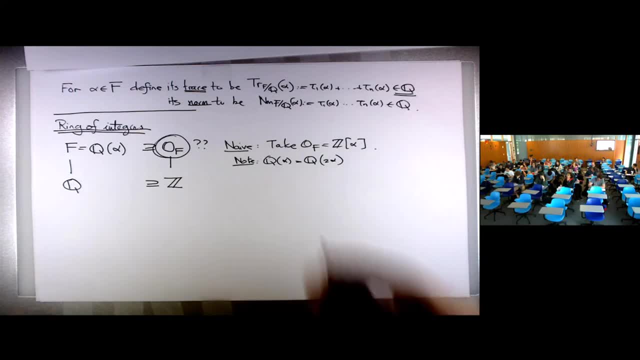 like adjoin them to q, then you're gonna get the same same thing. But of course definitely z alpha is gonna be different from z 2 alpha And sometimes the denominator would depend if you, if you were to define it. 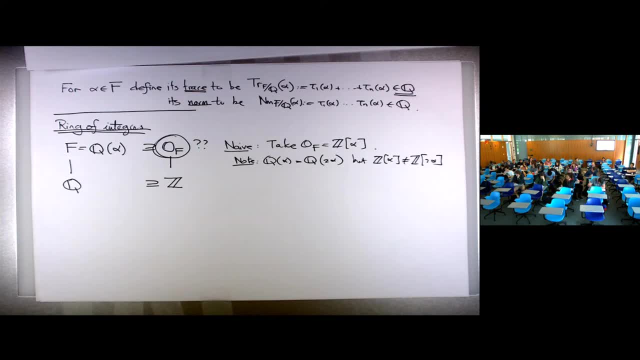 this way, it would depend on the choice of the generator alpha. That's not very ideal. You can also argue: maybe there's some way to q, some sort of denominator, some sort of coefficient too. But later on we're gonna see some examples. 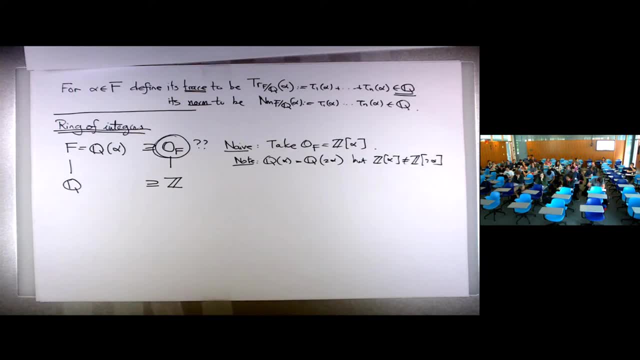 where it's. you know this alpha. you can choose other things which doesn't quite look like 2 alpha, For example. you can choose. most of the time you can choose, for example, for many cases, for example, you can choose. 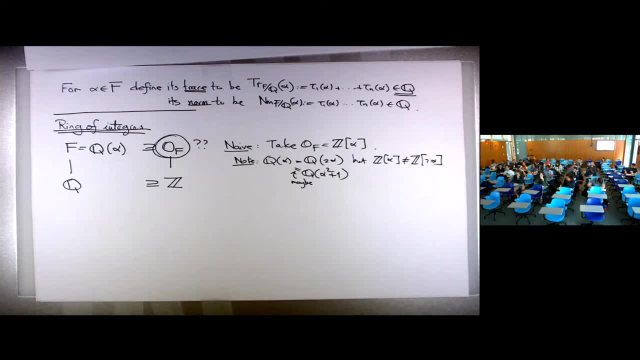 x alpha squared plus 1.. It might be the same thing, maybe, but this is not a good way. That's what I want to say. There's no good way of choice of r, But instead we're gonna do the following: 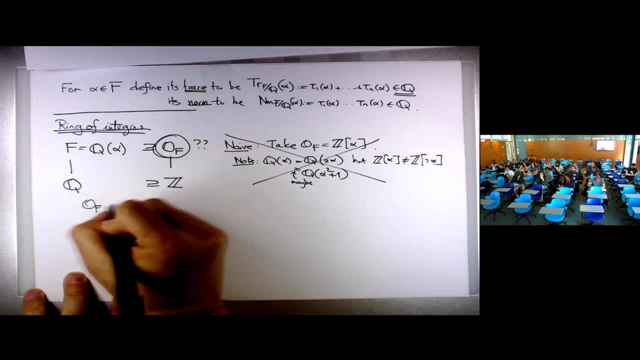 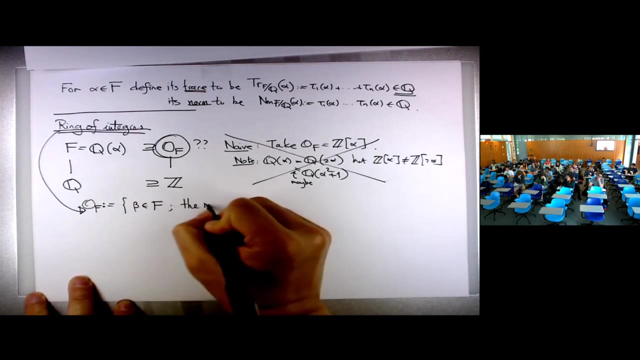 We're gonna define it in a very some sort of abstract way. So I want to define it to be: this is a ring of integer called f, So this will be all the elements beta in f, such that the minimum polynomial okay. 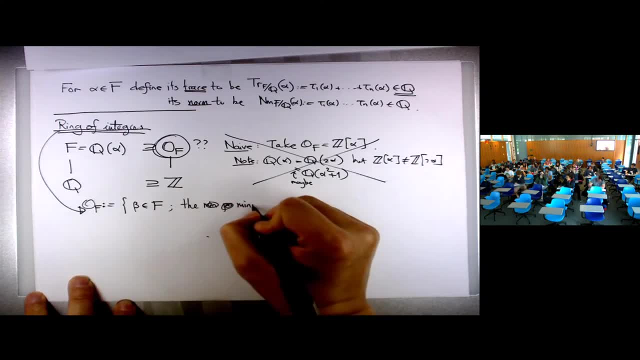 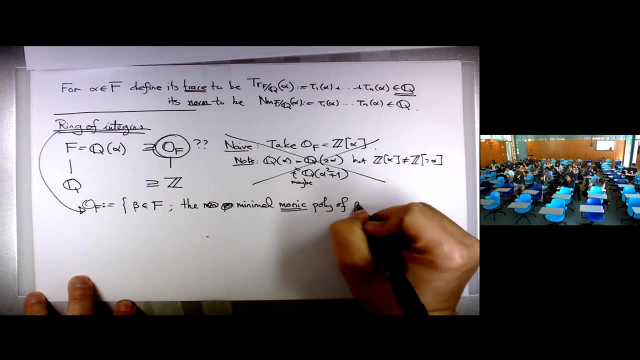 the minimum. let me write it down: minimum monic polynomial of beta in qx as coefficient in z. So by an element beta in f with a certain element, you can always find a common element in f. You can always find a common element in f. 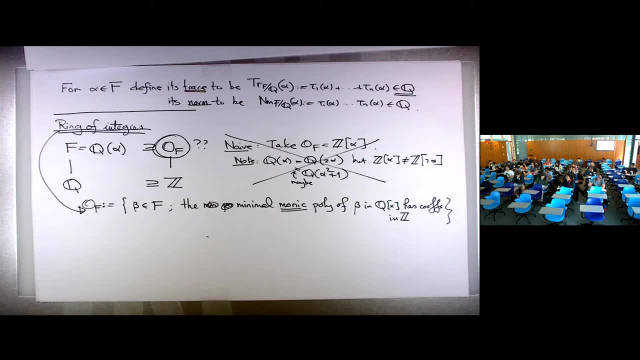 with a minimum degree, such that f beta is a zero of that polynomial. And you can always normalize the polynomial so that the leading coefficient is one. I want to do that so that at the end of the day, all the coefficients like if beta is. 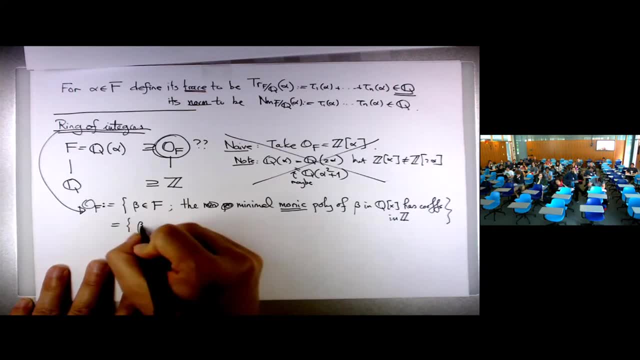 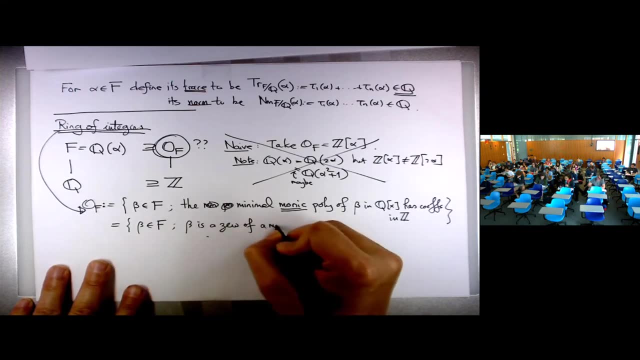 an integer, then the minimum polynomial of that has coefficient in z. It turns out this is the same of a monic polynomial in zx, Namely, this polynomial does not have to be irreducible. You prove this by factoring the polynomial in zx. 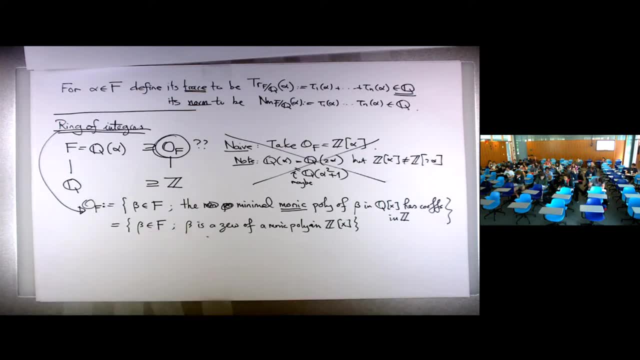 and you show that the factor that beta is zero of also has a coefficient in z. That boils down to zx is a unique parasitic domain. Okay, so here's maybe the example. It's rather abstract. I guess It's better to give an example. 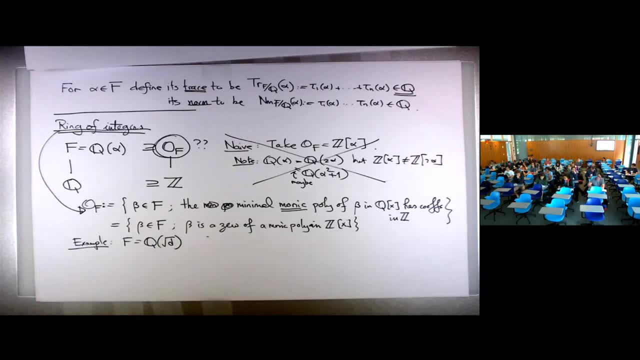 So the, I guess, very first example many people use when talking about number fields is the quadratic field q, joint root of d. For well, for d, a square-free integer. You can actually read that into the water: Square-free means. 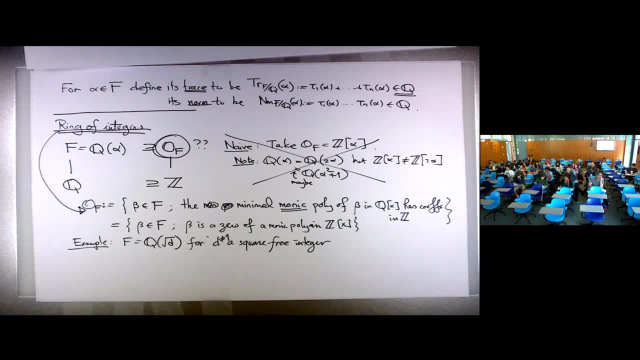 that when you factor the integer of d in your product, there's no p squared in the factors I mean. otherwise you can just take it out from there, Anyways. So then the ring of integer in this case is for most of the cases. 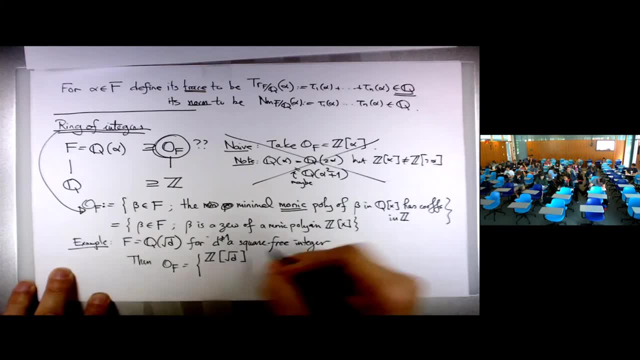 z joint root of d, where d is common to two or three mod four. The other case where d is common to one mod four. So you can, you have a something that doesn't quite look like an integral One root of d over two. 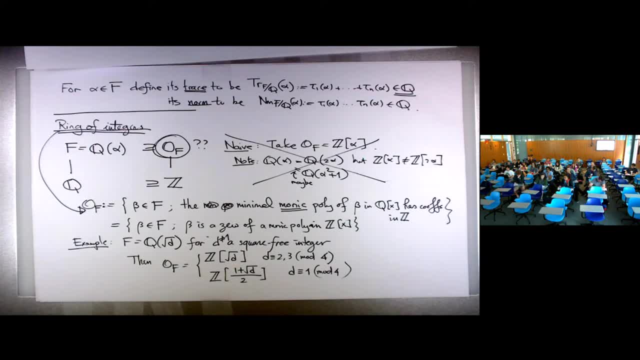 That turns out to be in the ring of integers. Here I didn't have the case where d is divided by three, because if you divide by three that won't be square-free. You can take out the factor four from the square-root, Okay. 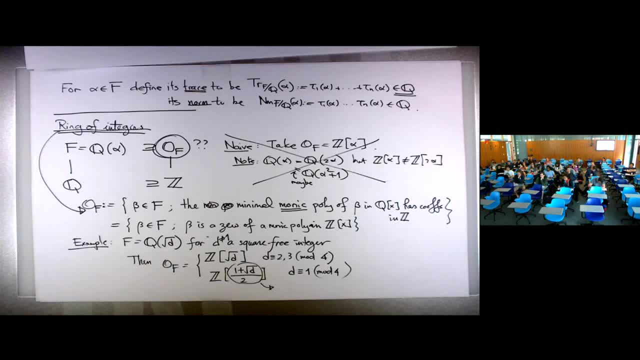 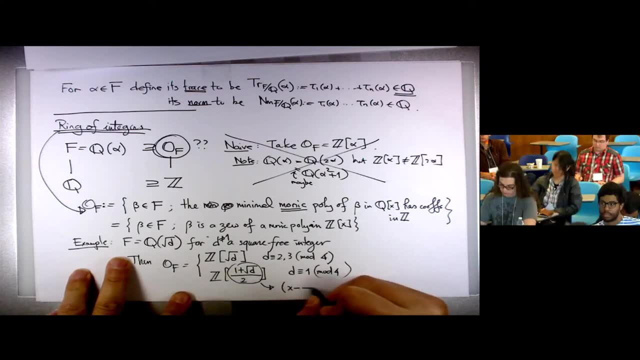 So I want to show that this is actually a zero of a modding component with coefficient z. So why is that? Well, let's try to build one So I can do this. Right, But this is not of course. 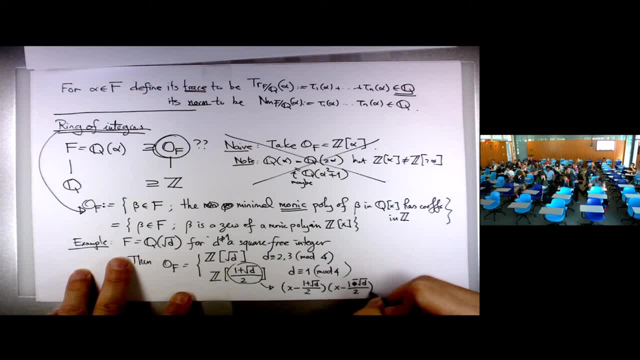 the coefficient is not in z. What I want to do is I want to. this is really complex congregation, But if d is positive it still makes sense to talk about the kind of conjugation in some sense In the real contract you just 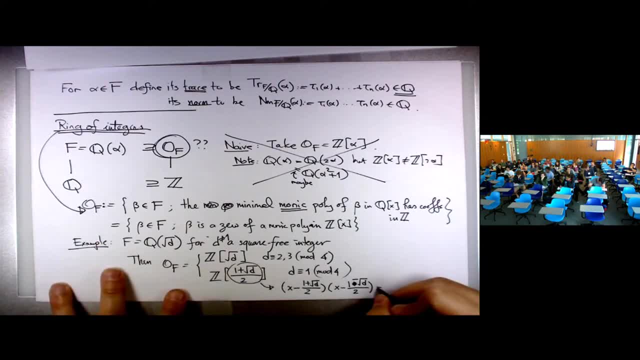 turn the root of d into negative root of d. Okay, Now let's multiply these two out. So what do I get? I get x-square. I'm just going to concise calculations. So I get this: 1 plus root of d. 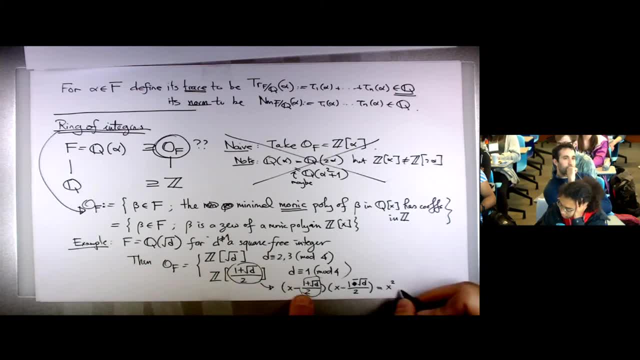 over 2 and 1 minus root of d. Sum them. So I end up getting negative 1, negative x for next term And for the last term it's going to be plus, excuse me, 4 plus 1 minus. 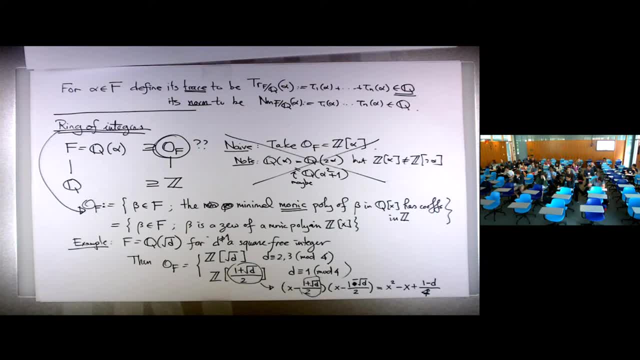 d, 4 in the denominator and 1 minus in the numerator. Think a little bit Now you see that if d is congruent with z, it's going to be the same way in z. So therefore, although this 1 plus, 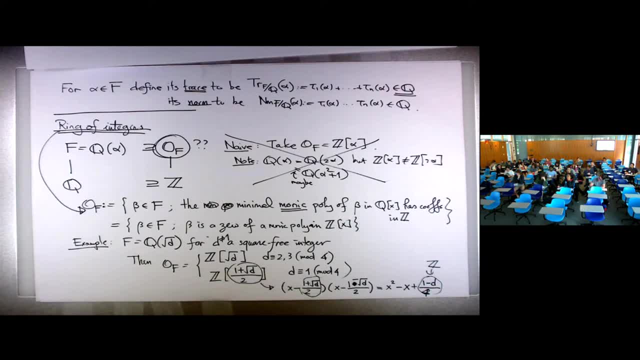 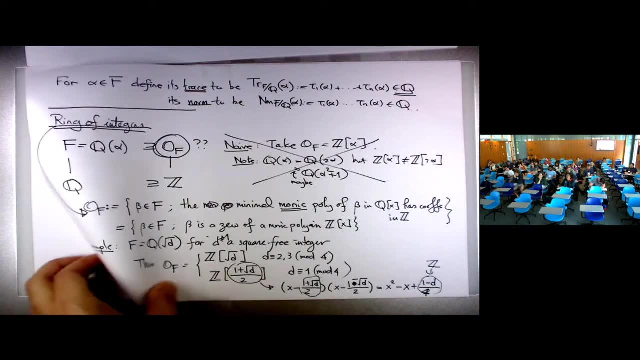 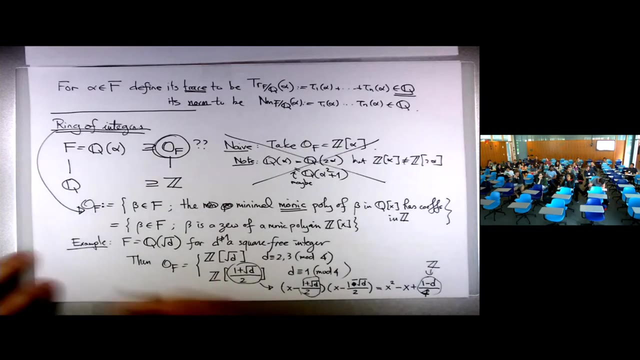 root of d over 2 doesn't look like very integral, but it is a zero of integral coefficient polynomial Okay, Good. So this is one of the examples. honestly, Oh you know what, Let me stick here. I want to. 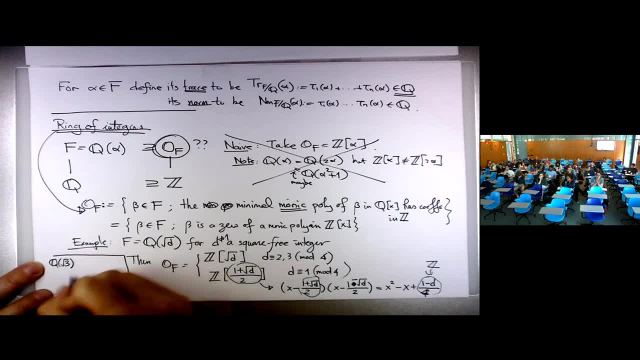 I want to give you concrete examples. If you do q adjoint root of 3.. Let me try q adjoint root of 3, that's just z adjoint root of 3.. However, if you do q adjoint negative, 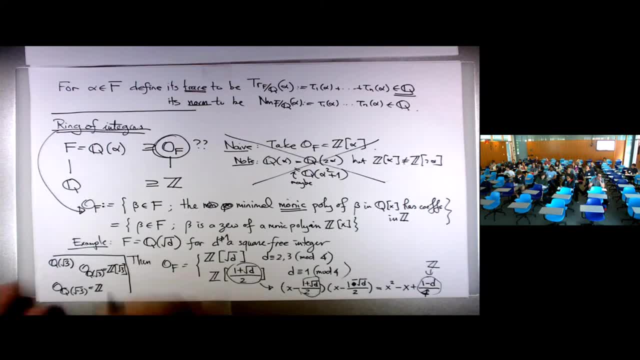 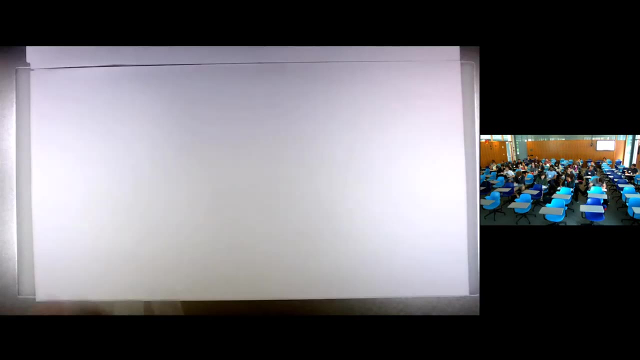 root of 3, now that negative 3 is congruent to 1 plus 1.. So you have z adjoint that, All right. So for example, just an example. Let's see more examples, If I. 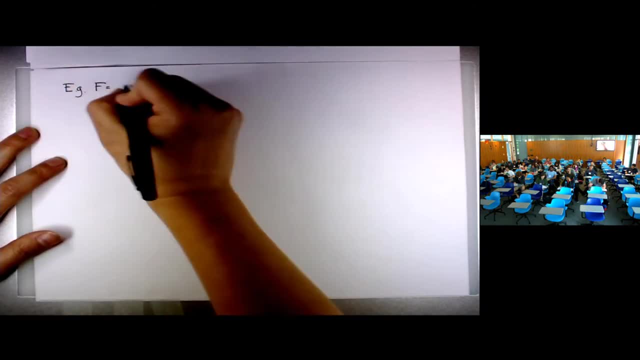 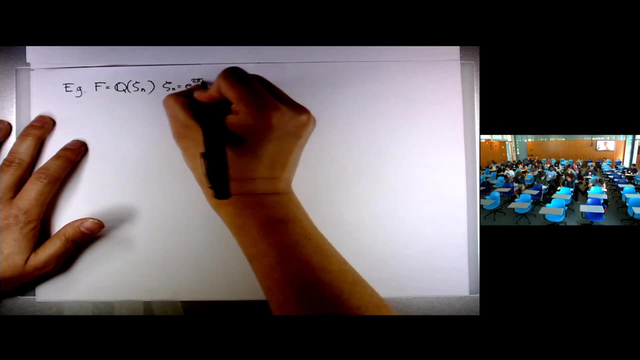 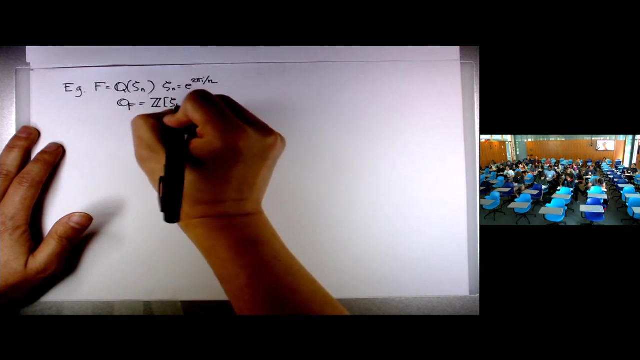 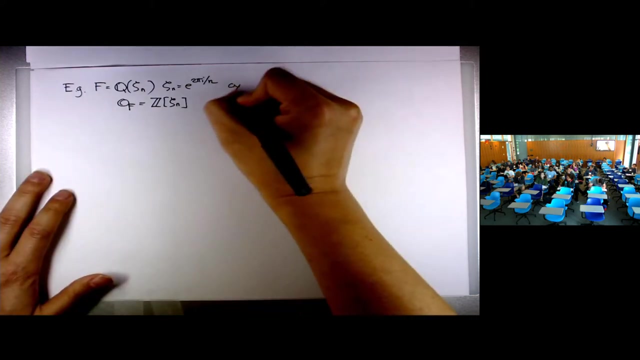 take f to be q adjoint theta n. theta n is the answer to mu. Okay, In this case O f is actually just v adjoint z a. So this is called the cyclotomic field, I should say. If your, 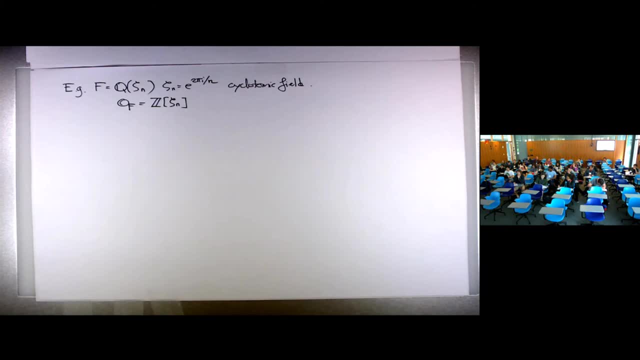 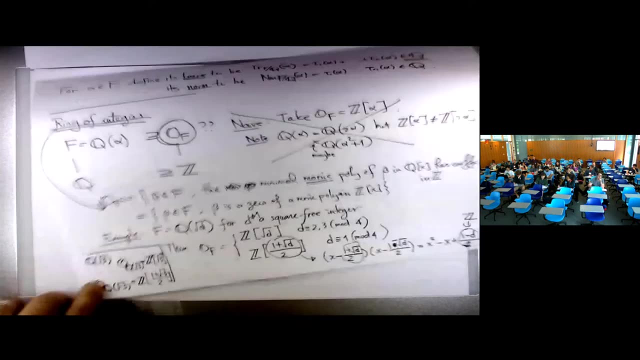 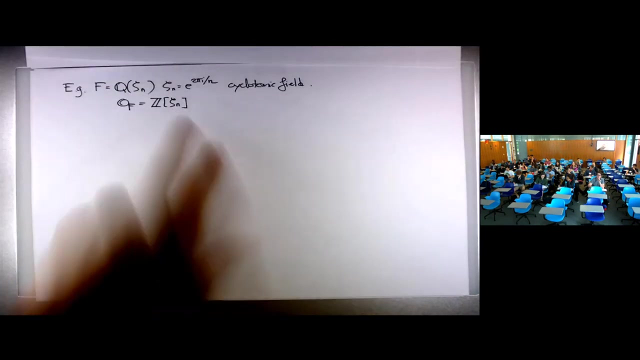 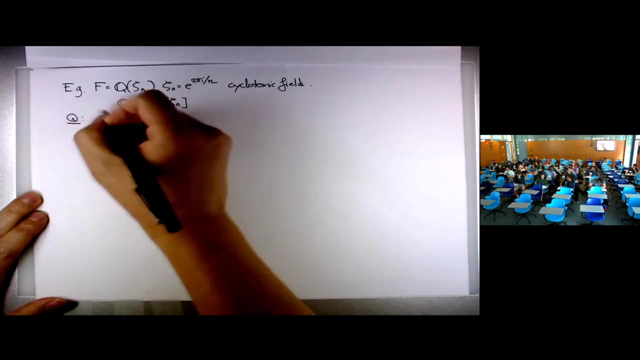 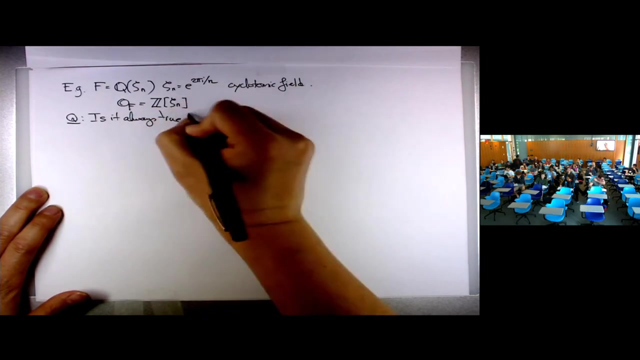 joint ends in the. Then it looks like all the examples we saw, I mean like in the quadratic case. of course. that's what the ring of energy looks like. And then this cyclotomic field. is it always true that? 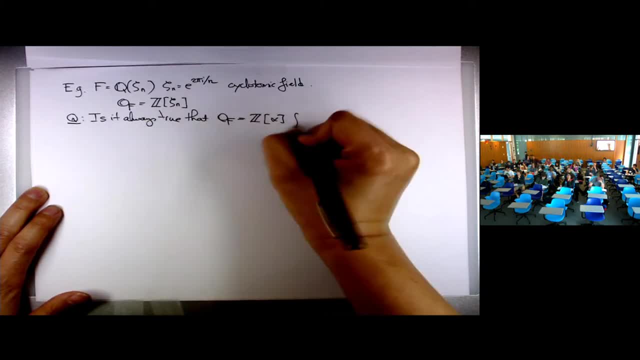 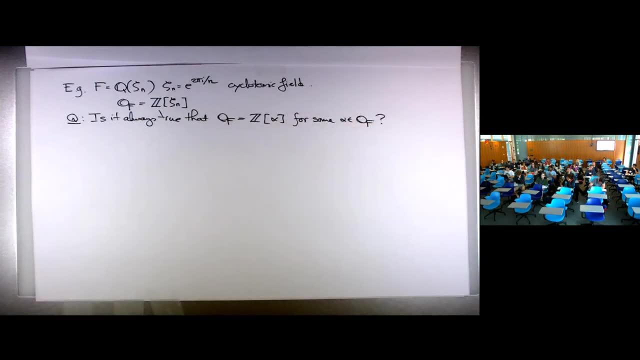 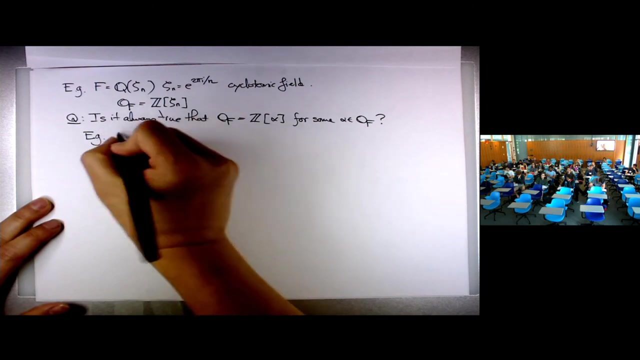 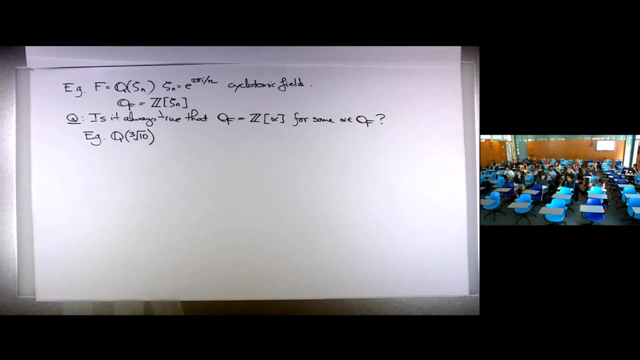 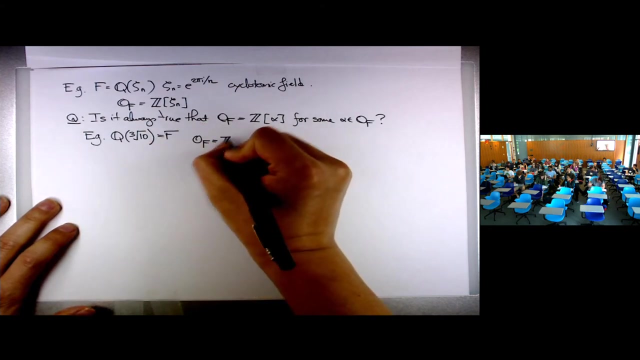 my O f is always v, adjoint alpha for some r. Let's maybe look at another example. Let's see. Let's start talking about cubic fields, Degree three, Adjoint cubit of 10.. This is my r f. 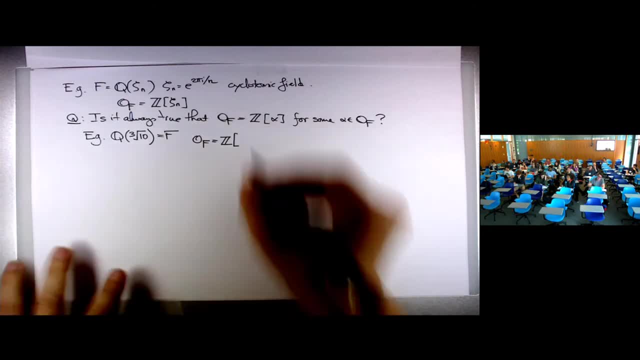 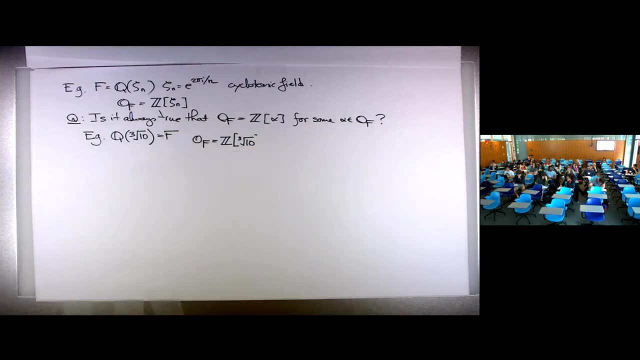 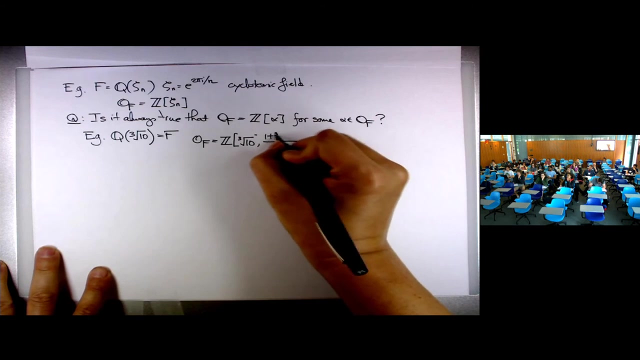 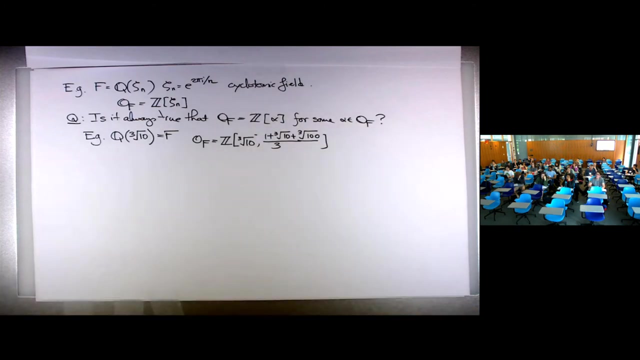 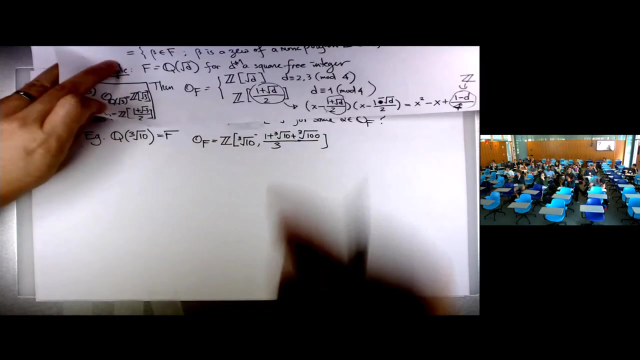 It turns out if you go around and write, let's see, okay, It turns out that O f is a little bit bigger than that, Like this Kind of a sharp. You can see that It's not that in some sense. 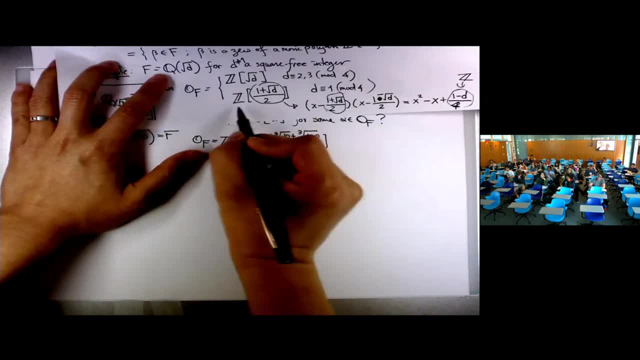 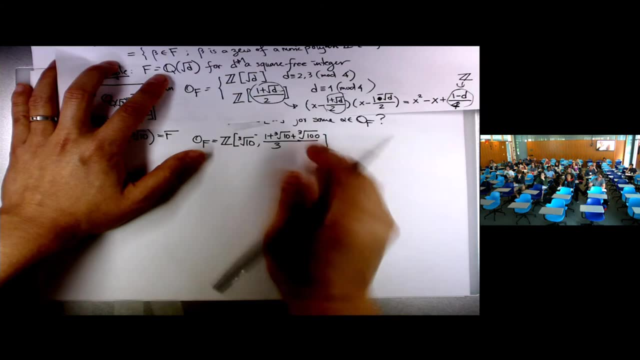 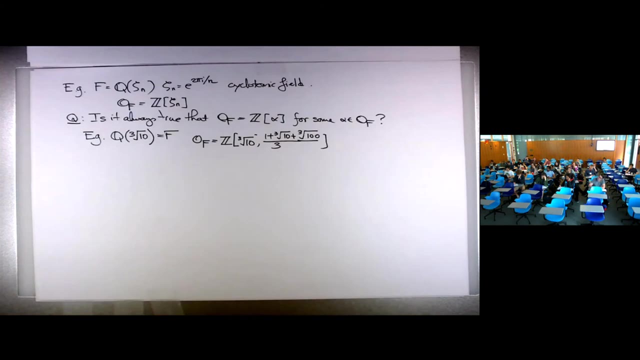 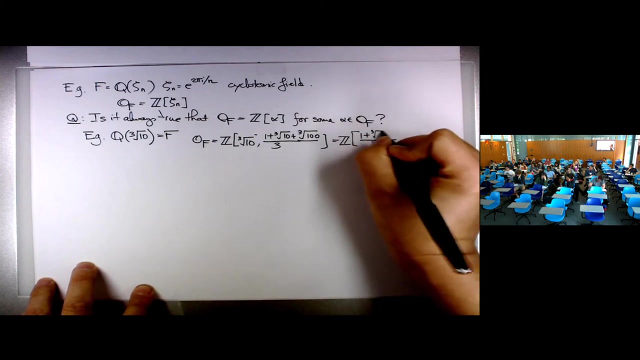 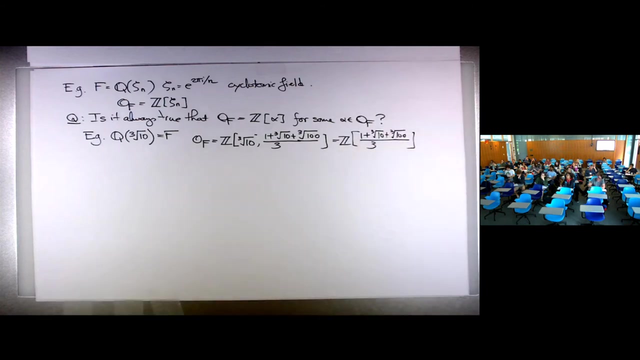 And these two kind of share some similarity if you think about it. But it turns out. this is not quite a counter example, But it's an interesting example in the sense that it turns out that the letter guy looks like 1 plus r plus r. 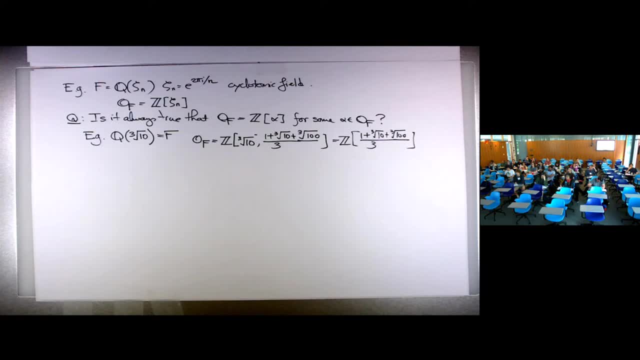 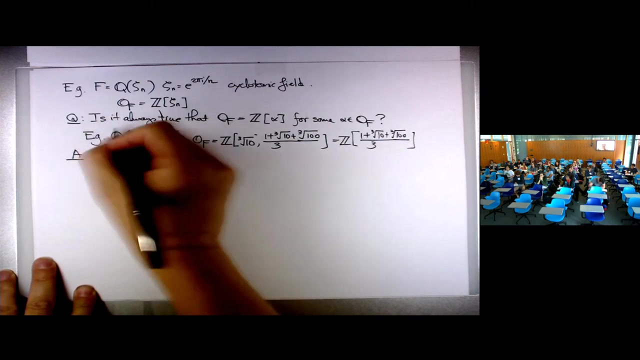 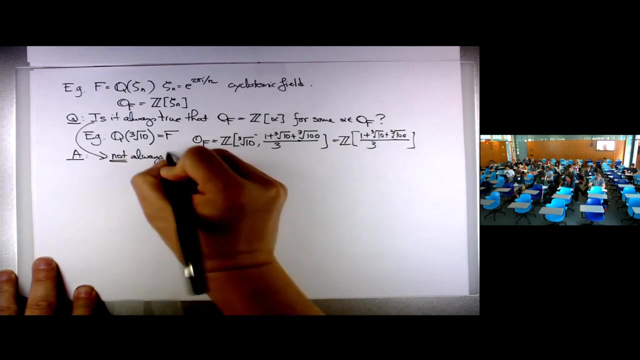 plus square over 3. This can generate cubits of this. So this seems to be also supporting the case that. First of all, I want to say that even in some cases, O f equals z alpha. the alpha might not be something you would think. 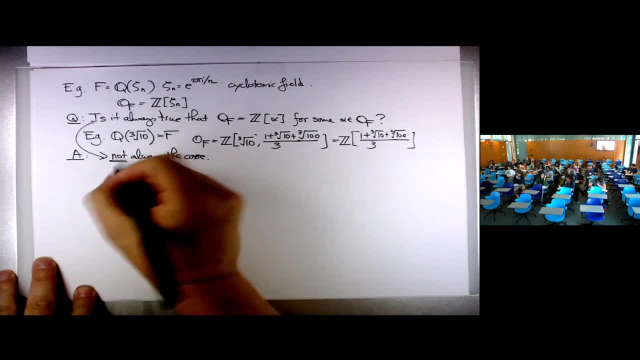 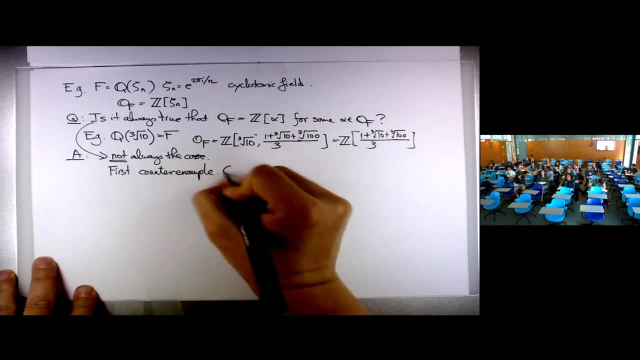 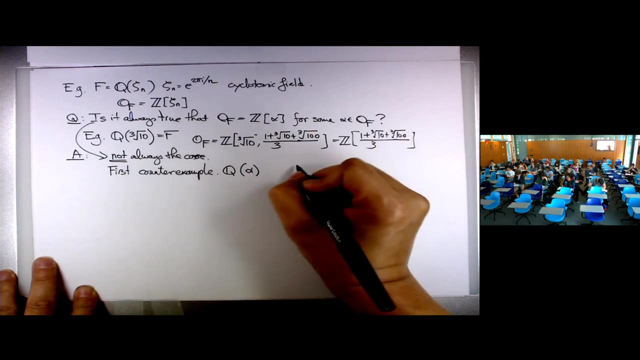 The example. So first a counter example Starts in qubit. All correctly, of course, is that there can never be one element, So hopefully I got it right. Oh shoot, Square minus two alpha, I think this is minus eight. 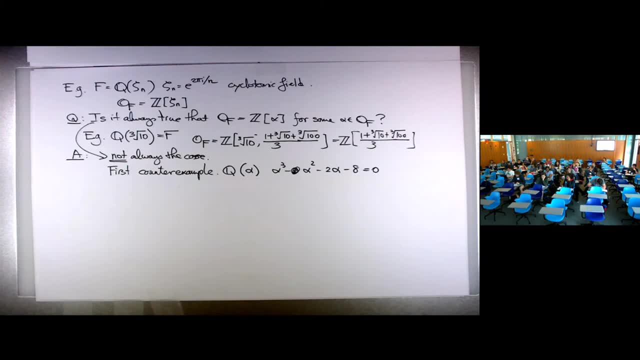 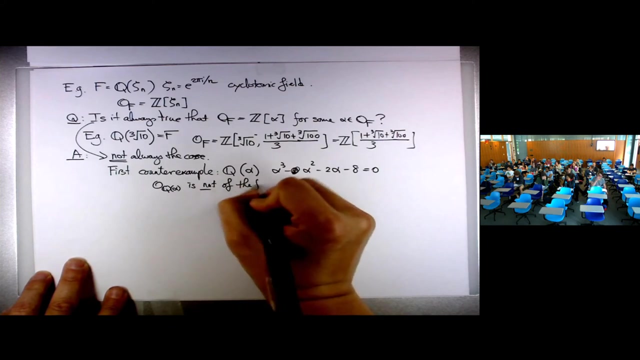 So play with the coefficient. One of them is: I think this is so you can check. this is irreducible, unless I get a sign wrong, And as it turns out that this one, there's no, so let me call it it's not of the form z beta. 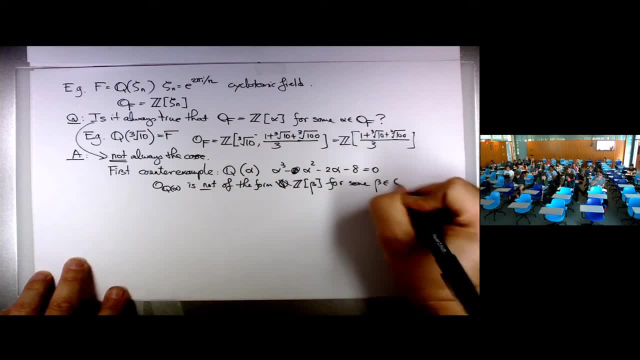 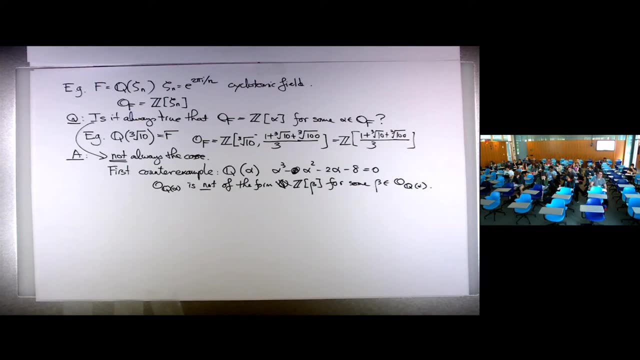 For example, beta In this vector, In the next, in the exercise, maybe for the next lecture or the after. I'll give you a way somehow. I'll explain a way. why this? why this is not generated by one element. 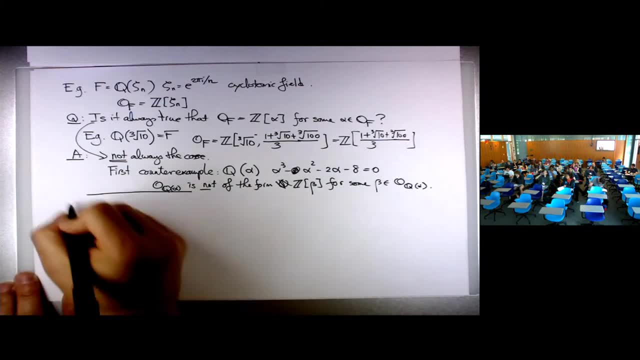 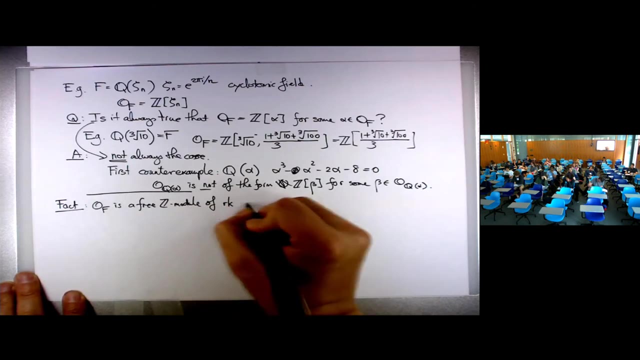 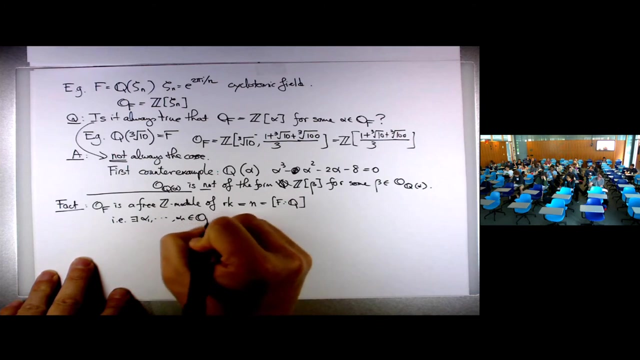 Okay, So that's not quite true. But what are true is that there's a basic fact about OF. OF is a free z-module of rank equal to n, which is the degree of the extension. By that I mean that you can find alpha one to alpha n in the random integers, such that 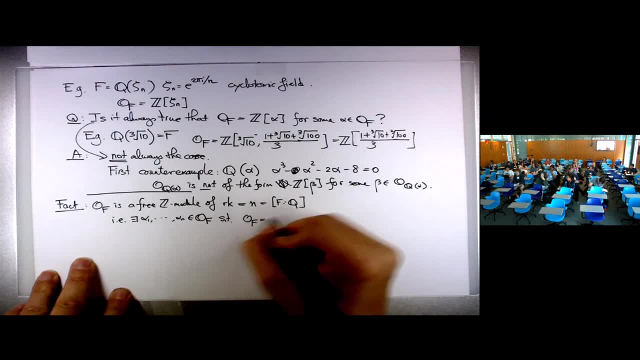 I guess maybe I'll just write it this way. So OF is equal to a1, r1.. a, a, n, r, n, Where a1 and a n's are n, z. All right, And also there's another fact that if beta is in the random integers, 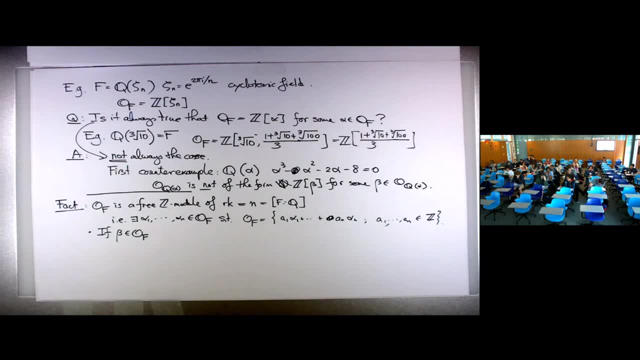 Earlier on we said that the choice of the norm of an element is a. the choice of the norm of an element in the number field belongs to q. Now if beta is in the random integers, then the choice of beta is in z. 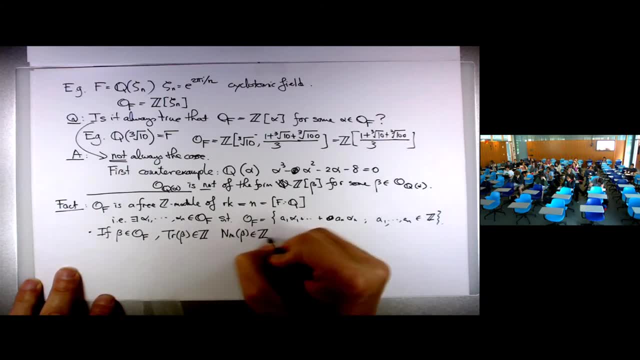 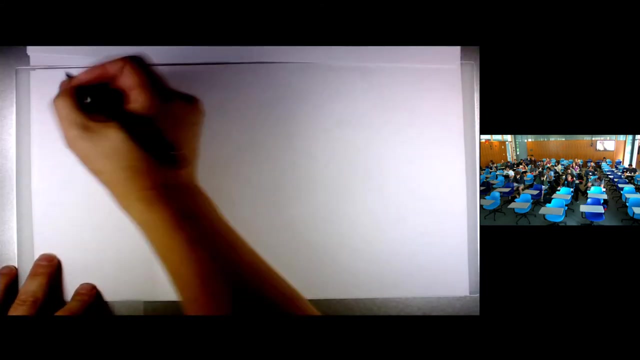 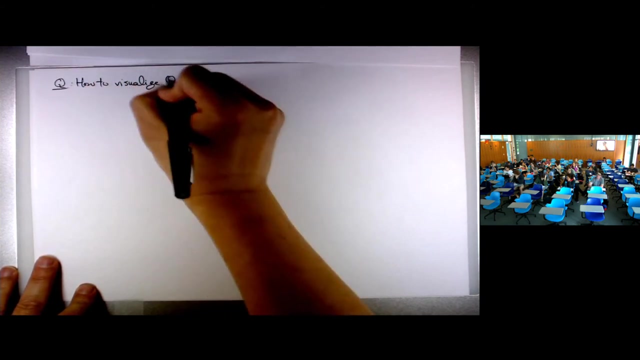 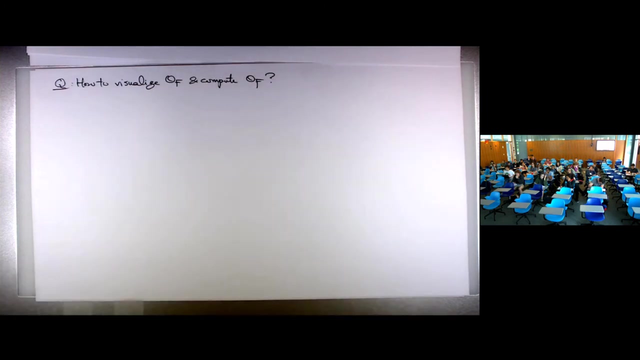 And the norm of beta is also in z. Okay, So are there any questions? Before I move on to the next one, we'll talk about how to visualize these OFs. So how to visualize OF and compute OF in some sense, In some cases, not all the cases. 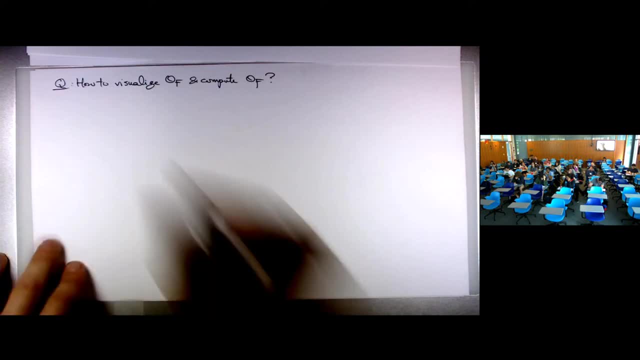 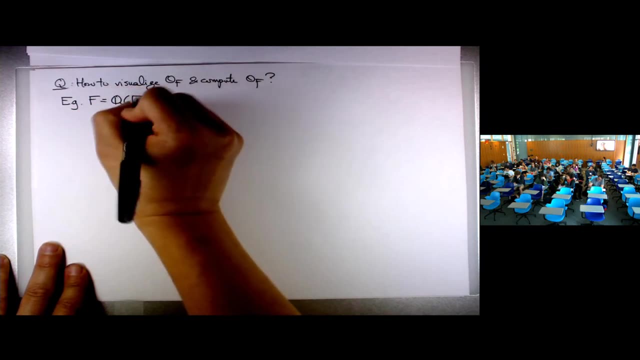 I'll just give you some sense of how this works. So let me start with talking about this by an example. So I want to use f equals q joined with a five- What we talked about earlier there- for every number of fields. 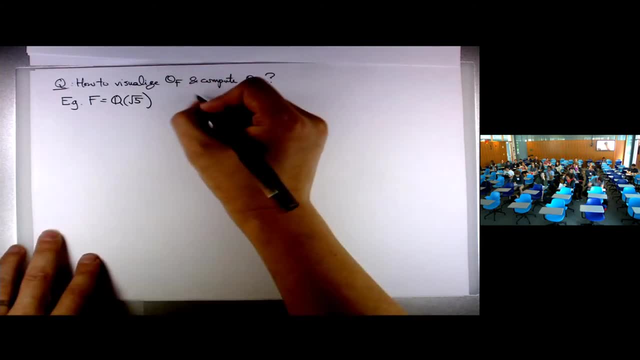 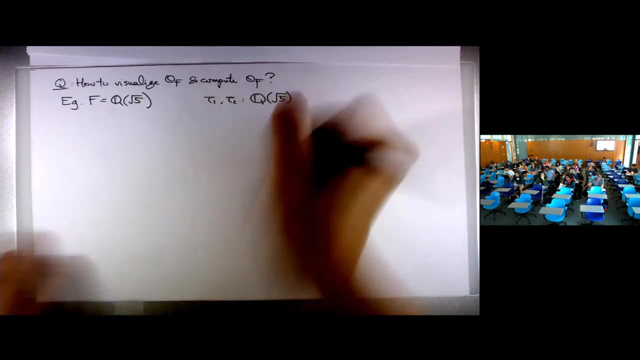 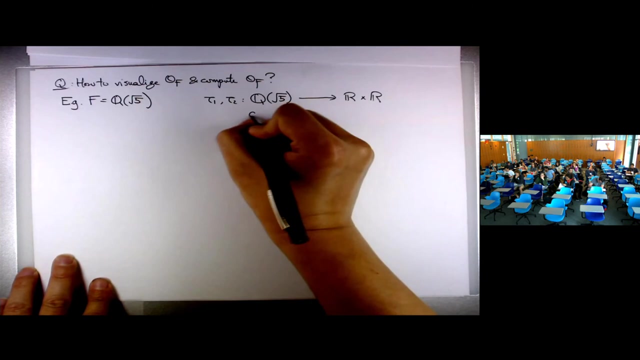 there are the same number of embeddings at the degree of the extension. So I have two embeddings. I've got tau 1 and tau 2.. I'm going to embed q to the two, But you know what? Let me, I'm going to send the explicit. 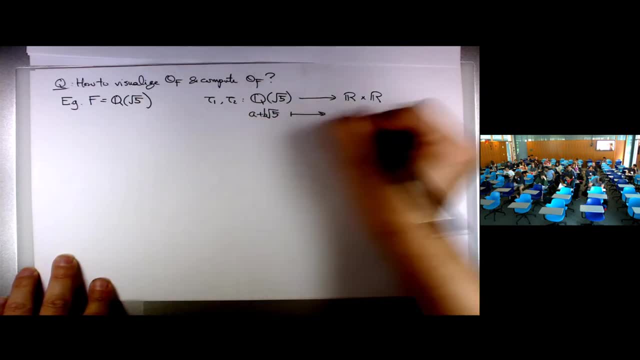 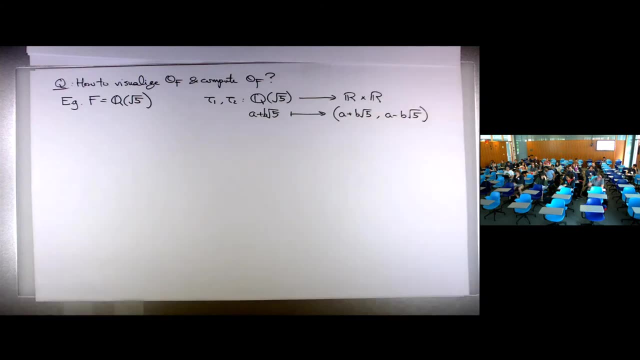 a plus beta to the five goes to a plus beta to the five or a minus beta to the five. Okay, Now I really want to visualize it by drawing a picture of this. See, we'll have two coordinates, Right, So let's see where the 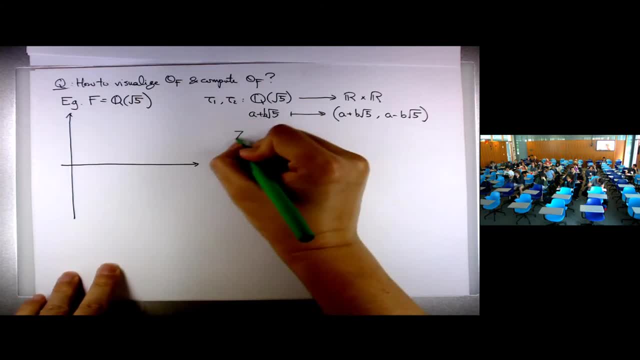 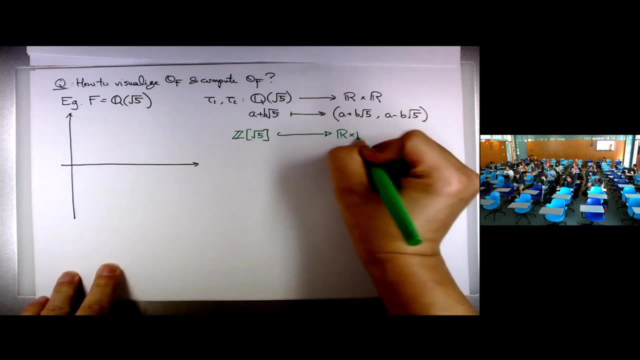 Excuse me. So let's see where, If I take z joined with a five- I mean using the same embedding, same embedding- into r, across r- this becomes- I want to say this becomes- a lattice. Let's see what it is. 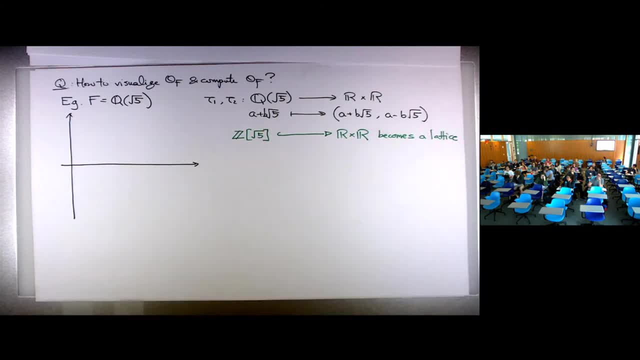 Let's see what I mean by this. Okay, what is z? I joined with a five, So let's see I have zero here. Let me use zero here. Okay, The number zero under the embedding, let's get into. 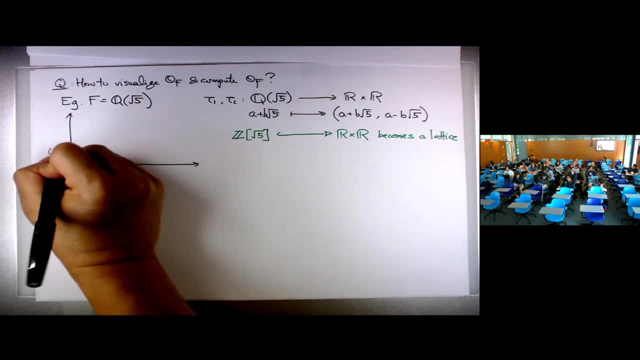 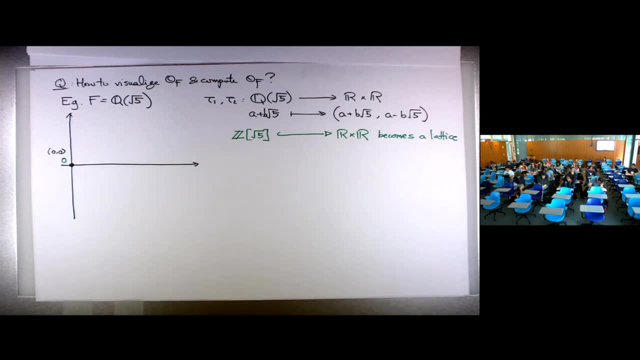 got embedded into the point zero zero, because zero will go to zero zero. So now, where does the number one go? Well, we have a one here. It's going to go to one and one, Right? So I should put a one here. 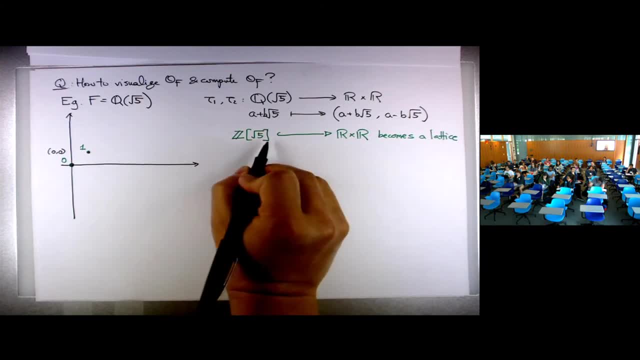 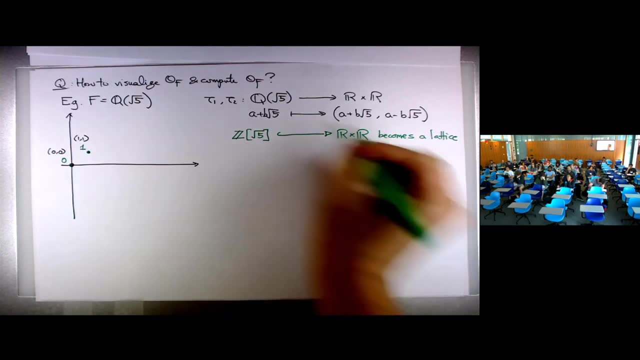 So this is the number one in z to the five. but the actual coordinate in this, under this embedding, is one and one And same for two. If you have two here, it's going to match two and two. So my number two is placed here. 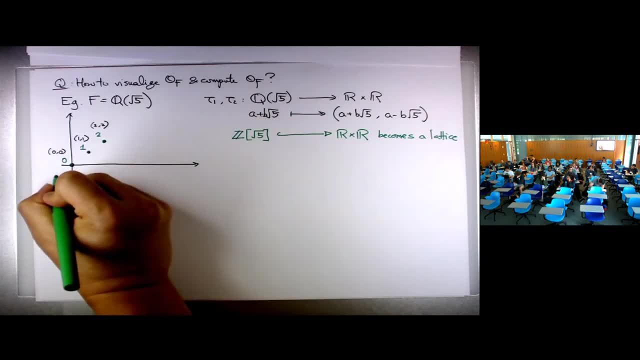 And so on. So you can imagine the negative ones here and all the others And so on and so forth. So all the integers are kind of in the diagonal line. That's because if you embed the integers into the rails the two embedding are the same. 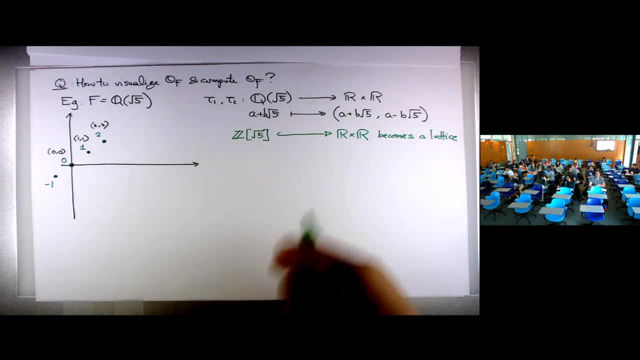 Right. So let's look at the other extreme. Like root of five, We'll embed root of five to r cross r. You get root of five on the first coordinate And the second coordinate. you have a negative sign here, Right? 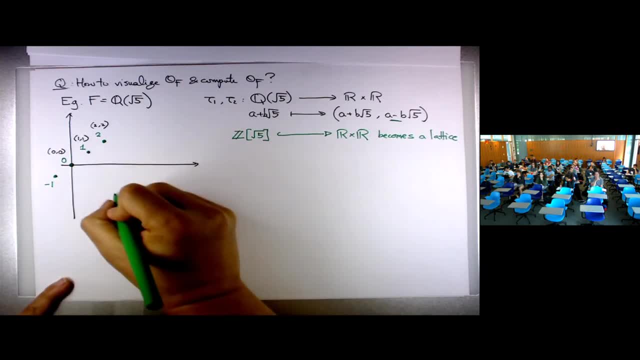 So you get negative root of five. So you get root of five in this way and negative root of five, So roughly here. This is where root of five is. The actual coordinate in the two-dimensional space is root of five. comma. negative root of five. 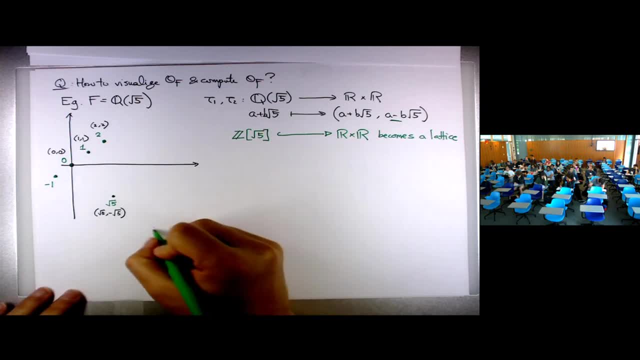 And if you do two times root of five you're going to get OK. So where does one plus root of five go? Well, you can think of it as kind of a vector space. Right, You have this vector zero to one. 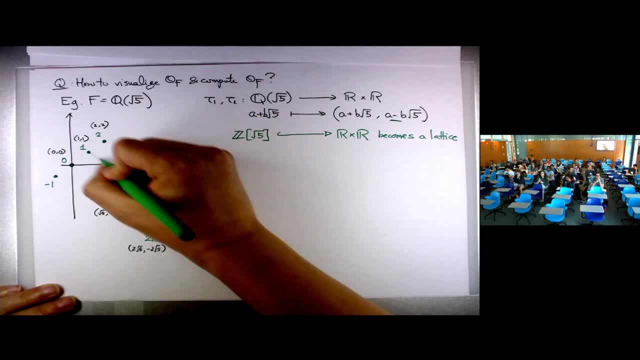 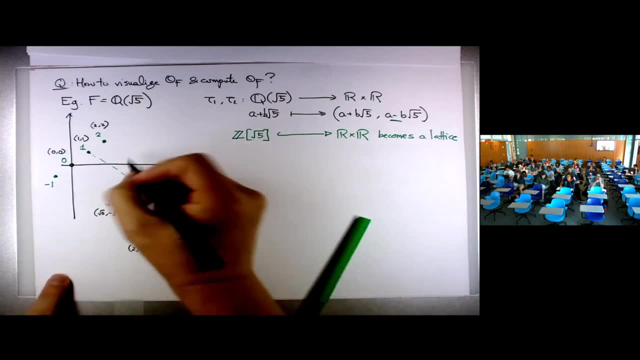 zero to. Then you can kind of start to link this together. That's where one plus root of five is And the actual coordinate is just one plus root of five, comma, one minus root of five. And then you see that if you embed this z-joint root of five. 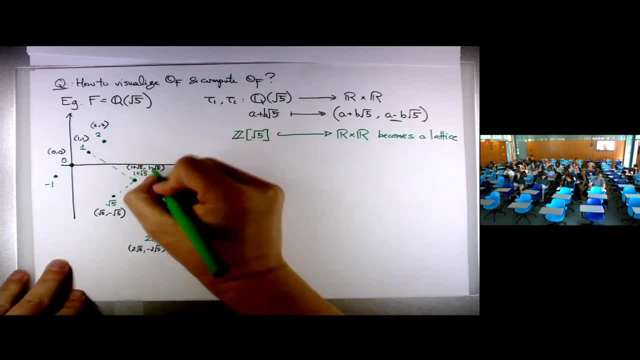 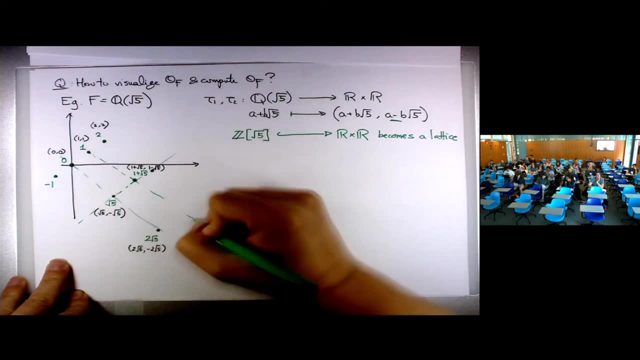 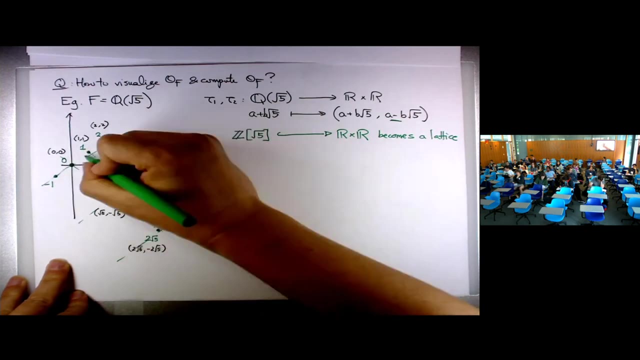 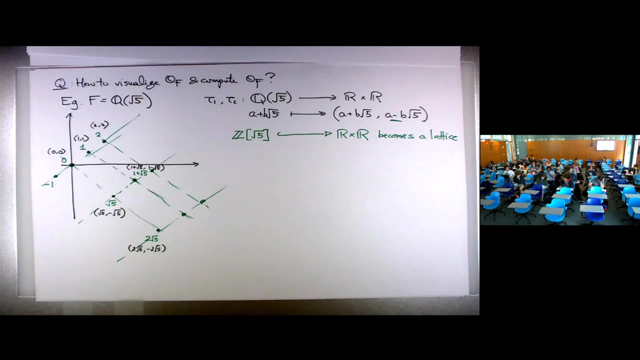 into the two-dimensional real space. you're going to get some sort of lattice- I don't know how to draw this Roughly- get some sort of lattice here, OK. OK, You get some sort of lattice And of course, for a lattice you can ask. 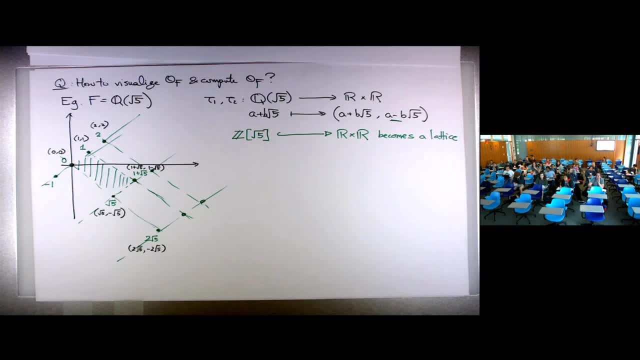 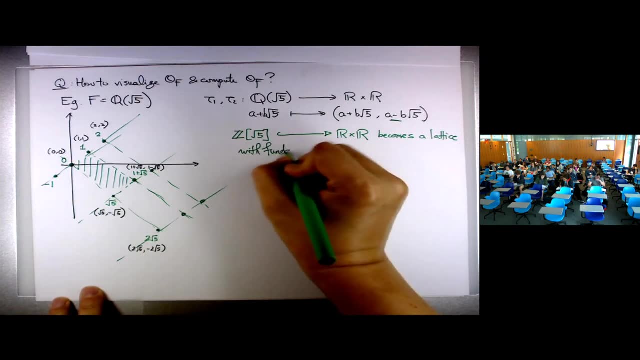 now, what's the area of each of the it's called fundamental area? What's fundamental area In this case? what is equal to? Well, I guess you can check. So this is like one one, So this is like root of. 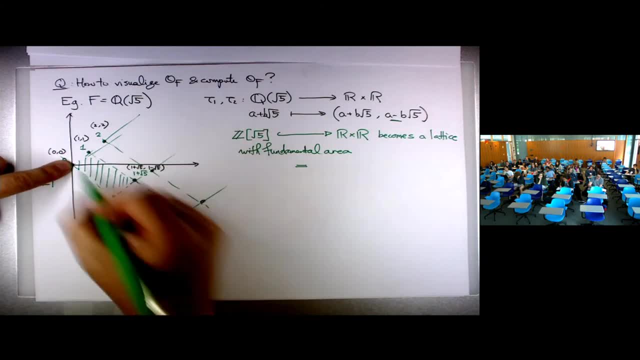 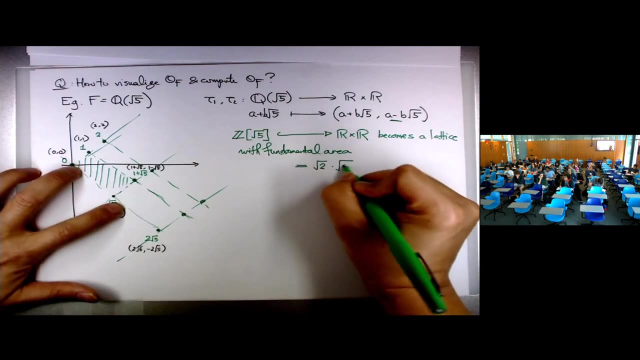 see, this is all 45 degrees up, Up. right, This is 45 degrees up, you know, right down. So it's like a rectangle right here in this particular case. So this side is root of two and this side is root of five times root of two. 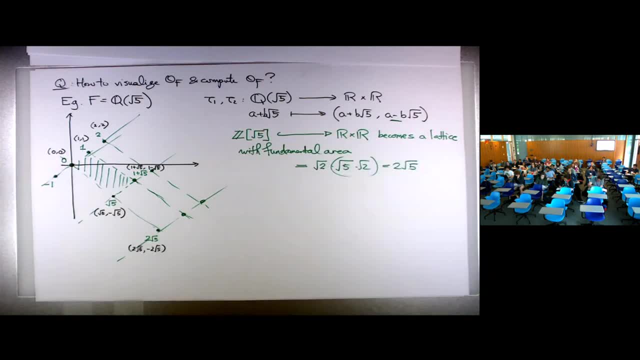 So I get two root of five. OK, Let's compute And like: this is like root of two, of course, And this is like this coordinate is root of five, But I want to for what I'm going to do later. 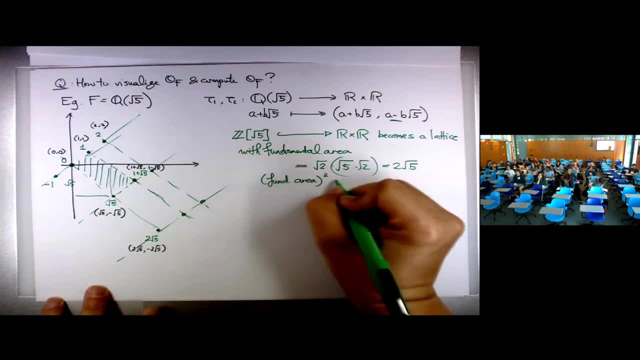 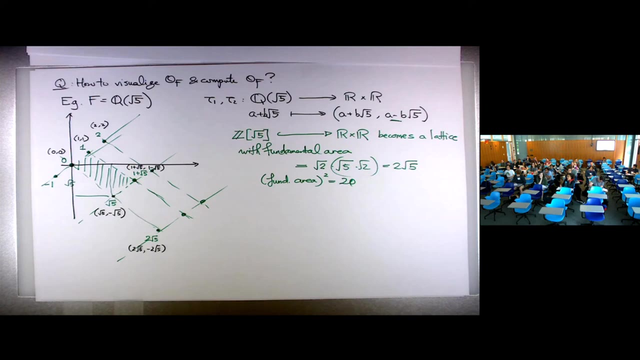 I'm going to do calculate this area squared for some reason, So this is 20.. OK, Now I want to remind you that for Q, Z to the root of five, Z to the root of five is not a ring of integers. 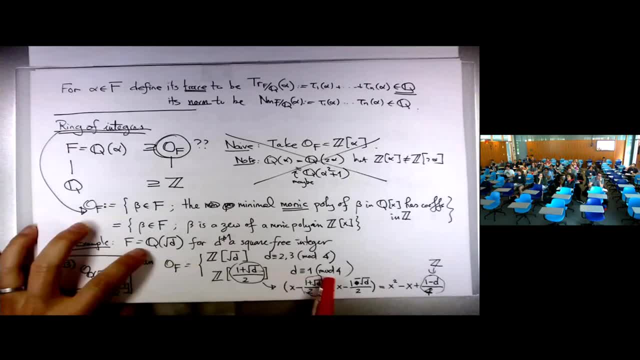 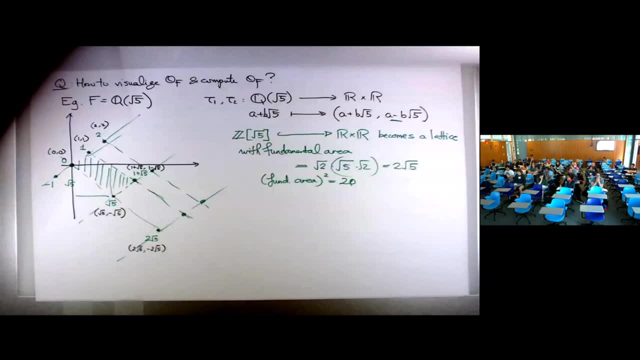 Just a reminder that remember that over here if D is common to one, log four, the, the ring of integers, you have this one plus root of D over two. So what I should be doing, should have been doing, is like: 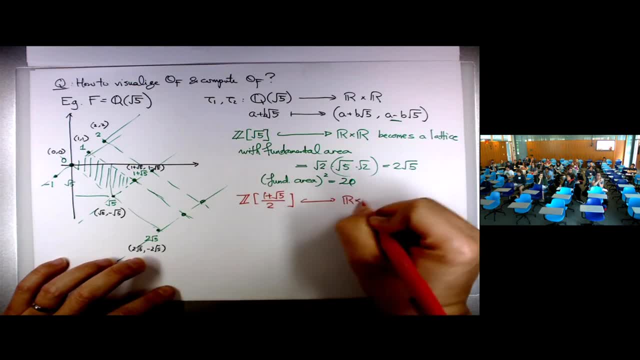 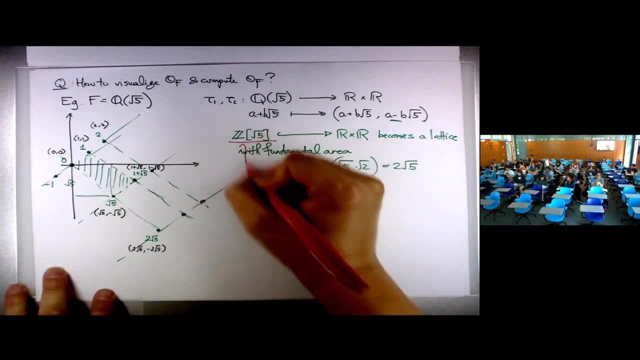 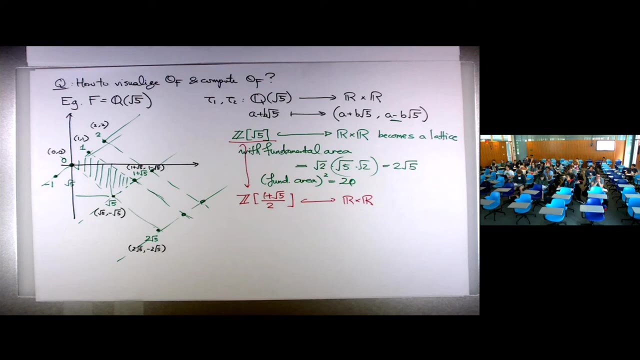 looking at this one. OK, So what so? of course, this Z to the root of five is contained in here. So all the, all the green points are already in this, already drawn here, But we have just one, you know. 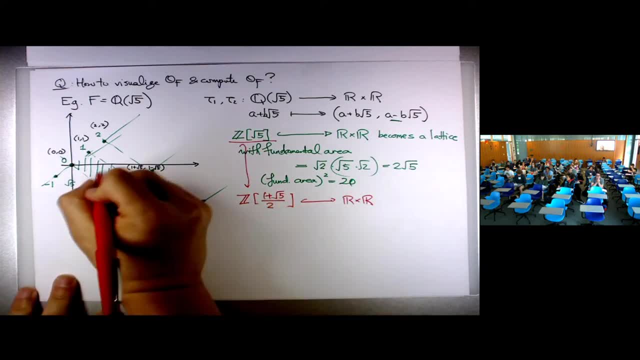 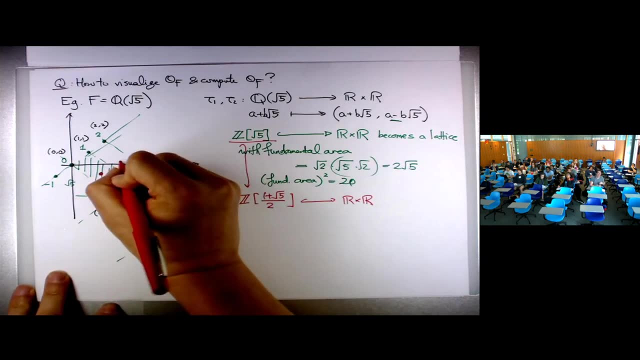 additional, additional points, For example, one point of five over two. So that's precisely the center of this. And also here, like you can add one, so it means add one here. So this is what is this plus one. 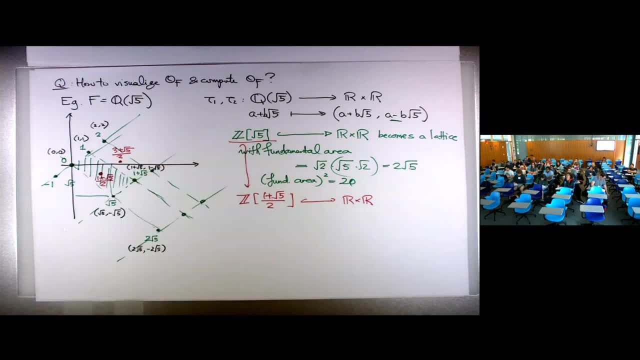 So three plus one. So it's going to be a five plus one plus one. So this is the final lattice, then this Z: I draw a root of five. You should add more points Basically in each of, in the center of each of the box here. 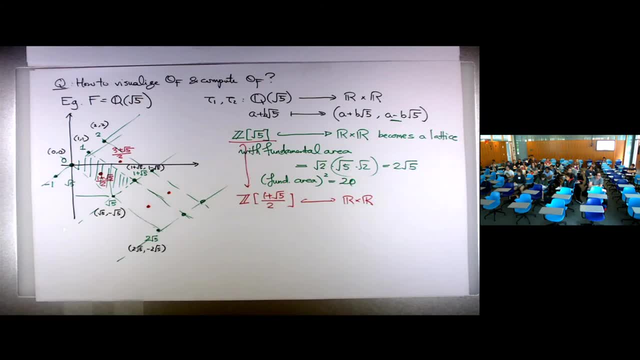 right in the center, you put a point. It's going to be a final lattice And I can also ask: the fundamental area of this final lattice, which is going to be this one, Or you can, you could, you could draw a different one. 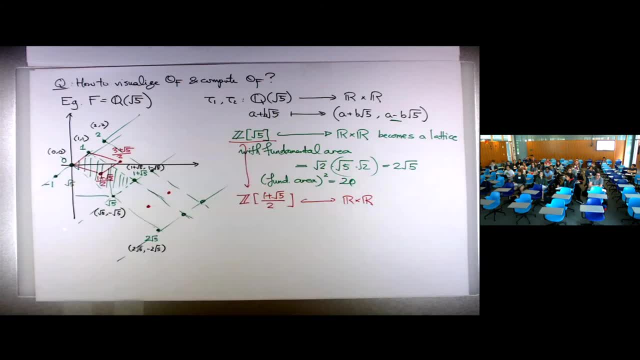 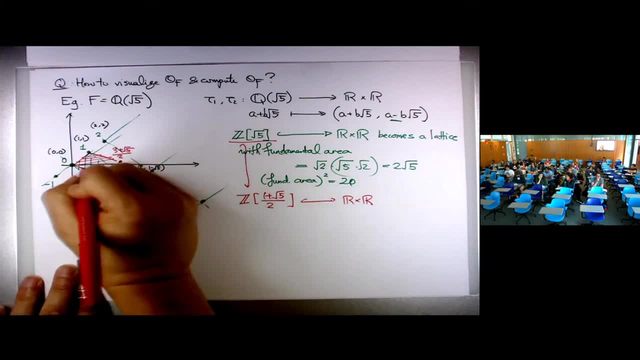 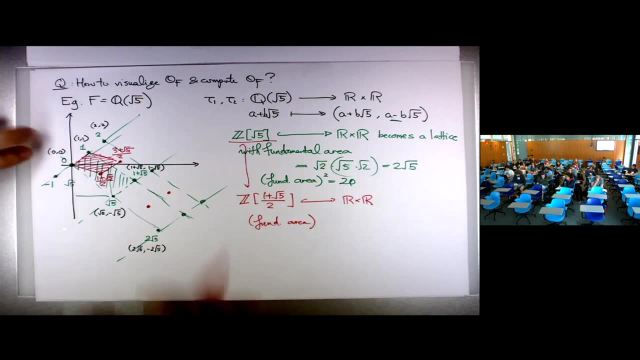 this is going to be, this is going to be. So, this fundamental area, Well, you know, you can somehow parallel move it. It's like half the area of the red region is half of the area of the green region, But your square, of course, is going to be fourth of that. 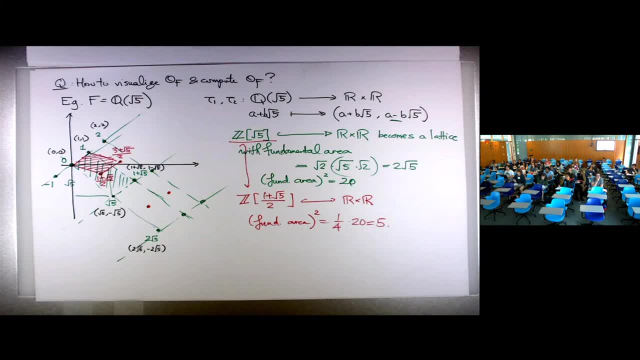 This case five. So this way, in some sense, we gave a way to actually kind of see what the range of integers are, See them using the embedding as some sort of lattice, in this case two-dimensional space, But later on we can kind of do something similar. 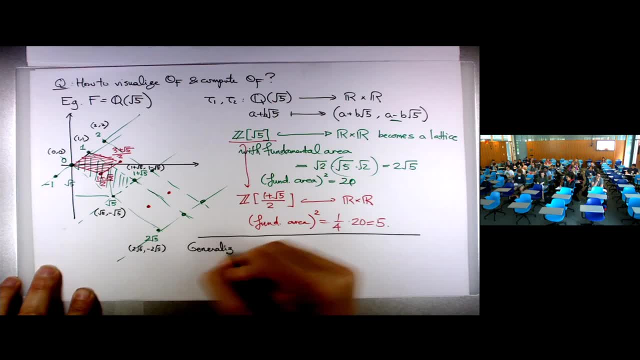 a generalization Is that when I have a number field, I want to consider all these embeddings. There's a small subtlety here that this f doesn't always go to R. In my case it's just like f embedding to the reals. 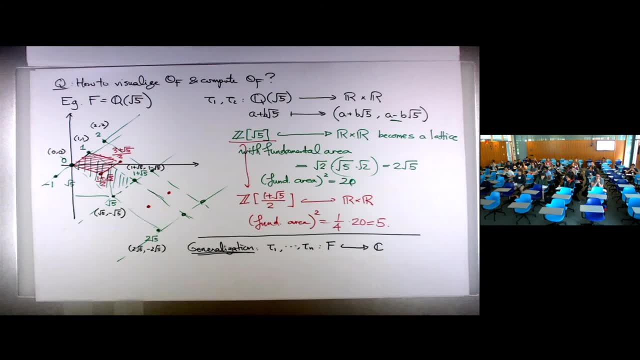 In general, it may not be real embedding. It's a couple of embeddings For the moment. let's forget about this here. Just pretend that these are all real embeddings. In an exercise you're going to work through something that's somehow two. 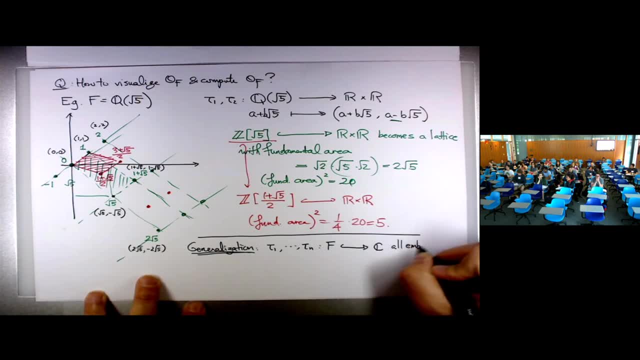 So solve, Solve this issue. This is all embeddings And so supposedly, this OX, the range of integers, is going to create a lattice inside this n-dimensional space. This is our n-dimensional space, And I want to know the fundamental area of that. 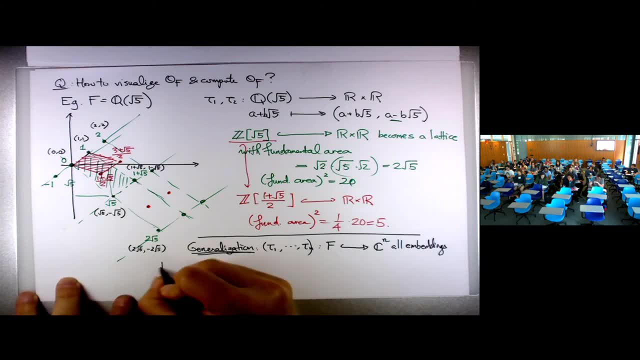 in some sense, or fundamental volume of that. So I want to define something called a discriminant of. so just give me a second For alpha 1, for alpha n, you can define it over f, For all the elements in f, you can define the discriminant. 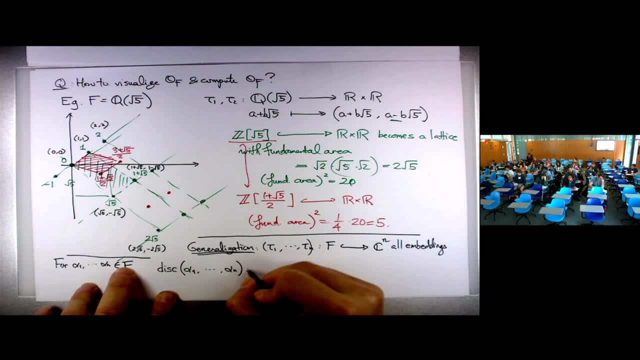 of them. This is defined to be the determinant. It's a little bit. I'll explain in a minute. It's kind of a big matrix. So why is this? Why do we define things like this? Well, I'm not sure if you learned this in linear algebra. 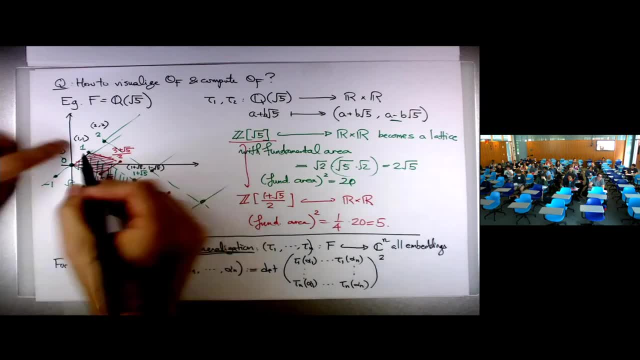 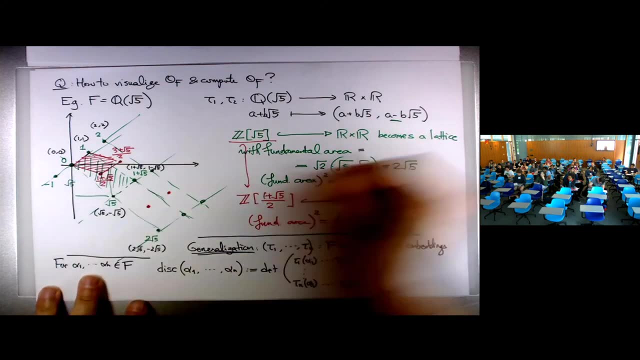 If you want to compute the area or the volume of some sort of parallel. one of the ways you do that is you do what I did here, But another way. for example, in this case, what you can do is that you can do the determinant. 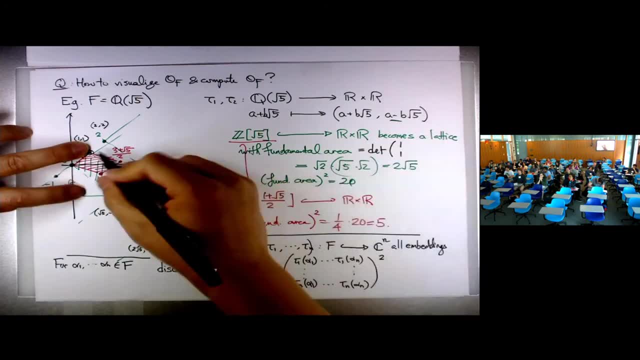 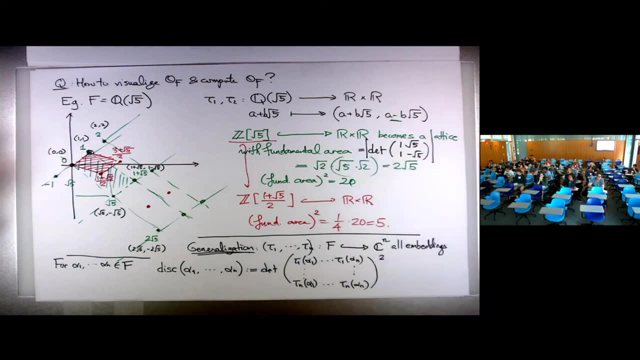 of this coordinate 1, 1.. And then the determinant of the other coordinate, root of 5, negative root of 5.. And then take absolute value. That's some sort of formula I'm not sure if you have seen before. 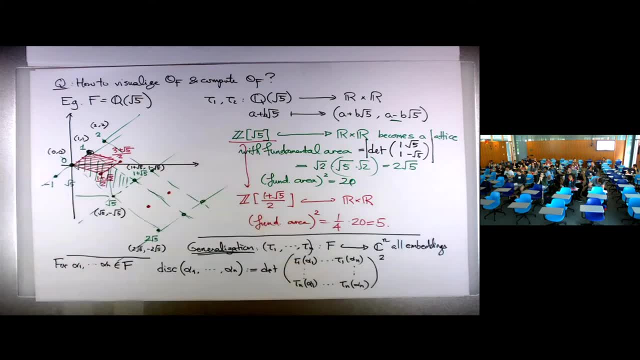 This is some sort of general linear algebra. If you want to know the volume of a parallel pivot, you take the determinant of the vertices. So this is the see the tau 1 through alpha 1, through tau n alpha 1.. Those are the first column here. 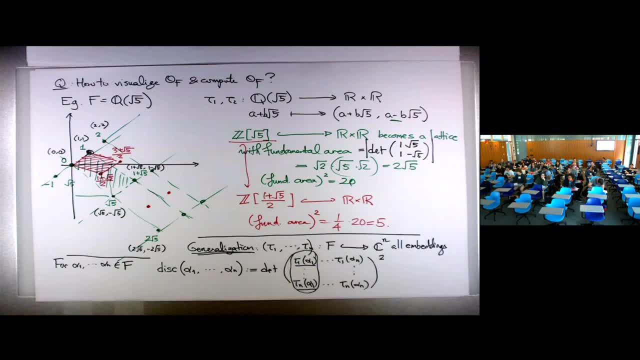 This is the point. Corresponding vertices correspond to alpha 1. And the next column here is going to be the vertices corresponding to the image of alpha 2, and so on. You take the determinant of the whole thing. Suppose you take absolute value of the fundamental area. 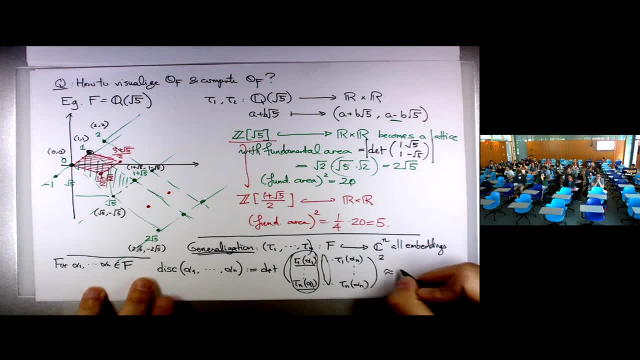 So this is roughly somehow the fundamental area squared. because I put a square here. Well, it would be literally true if it's not complex image, It's real image. Because of the complex embeddings it turns out, this determinant actually could be a negative. 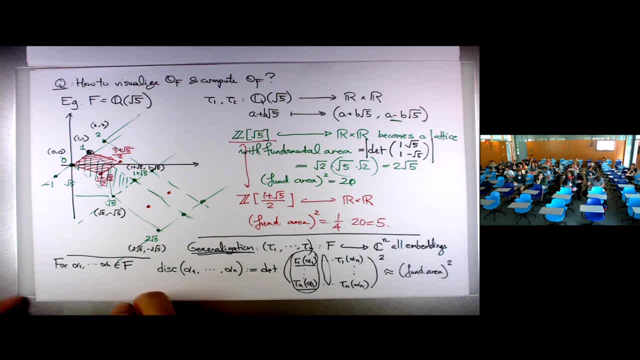 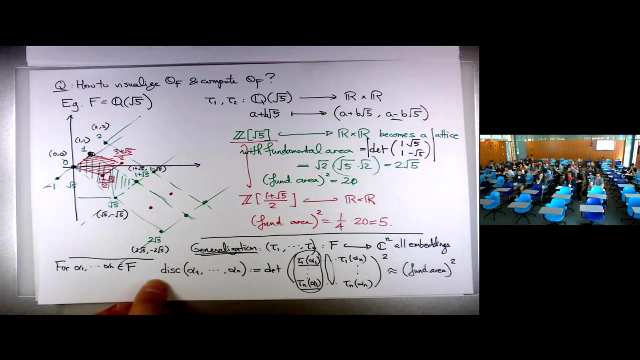 number. This is some sort of subtle things in an exercise that I won't have time to do this, But I think it's a good way to keep in mind that it's roughly the same as the fundamental area. Any questions? I know this is somehow the difficult point of the first lecture. 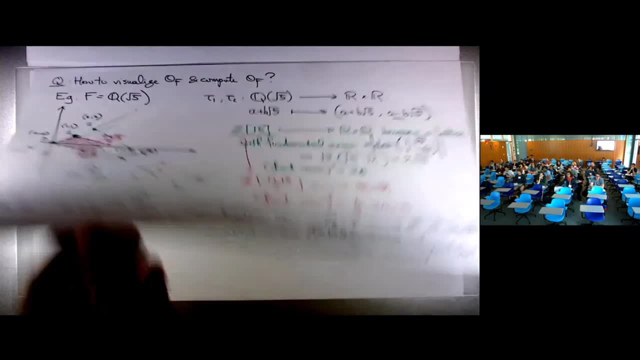 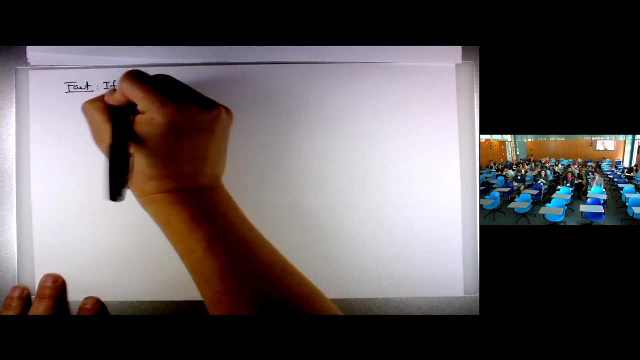 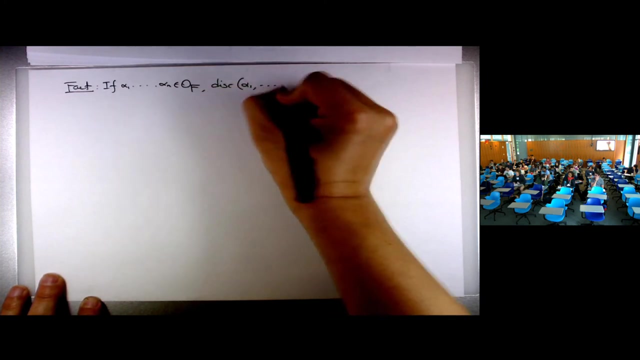 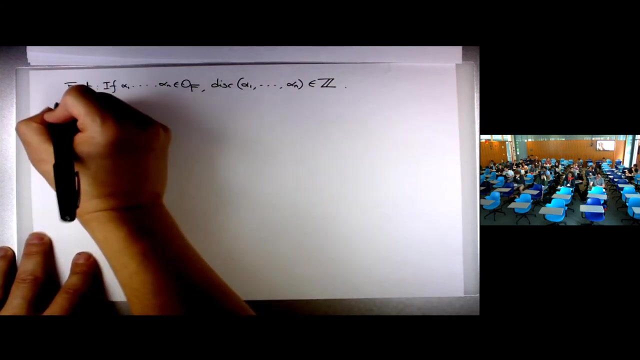 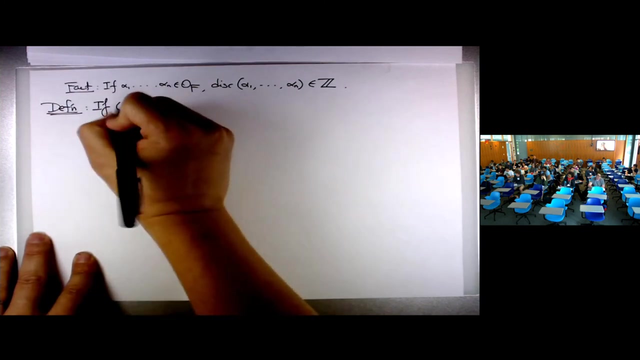 OK, Good, Very nice, Thank you, Thank you, Thank you. So now here's a fact: If alpha 1 through alpha n are actually in the ring of integers, then this discriminant defined is actually an integer. So definition, if I just give my alpha 1 through alpha n just precisely the basis of the ring, 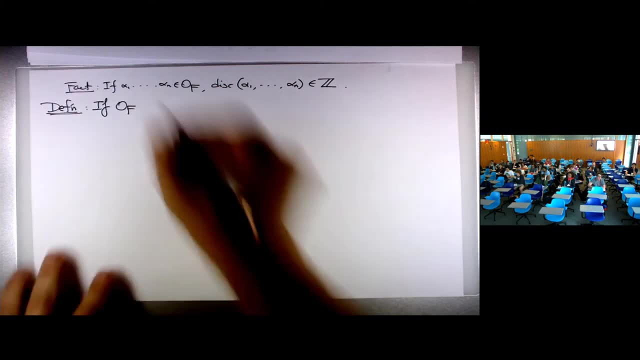 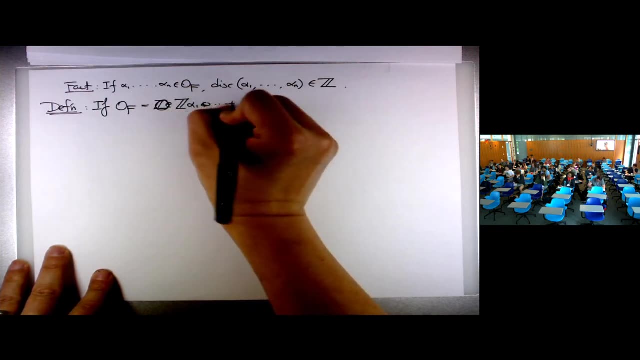 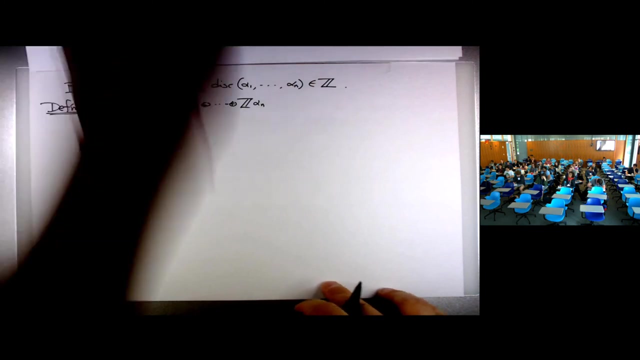 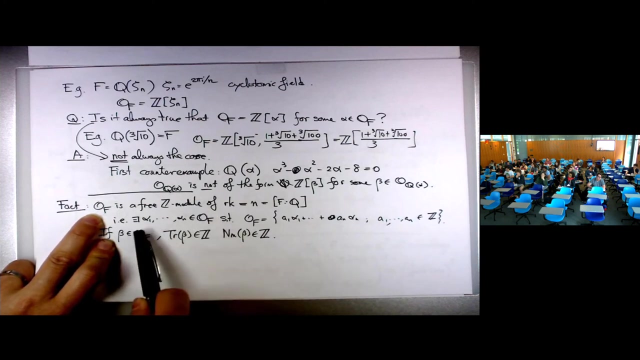 of integers, I can compute this discriminant. So if this is just precise, the alpha 1, the alpha n. So if this alpha 1 through alpha n are precise to the basis, namely where is this There? If we know that of is the free module, free Z module, then I can find alpha 1 through 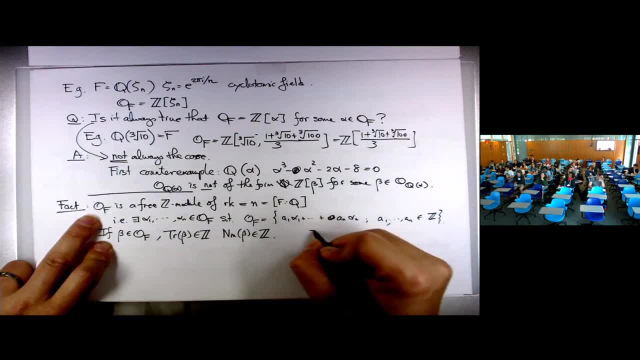 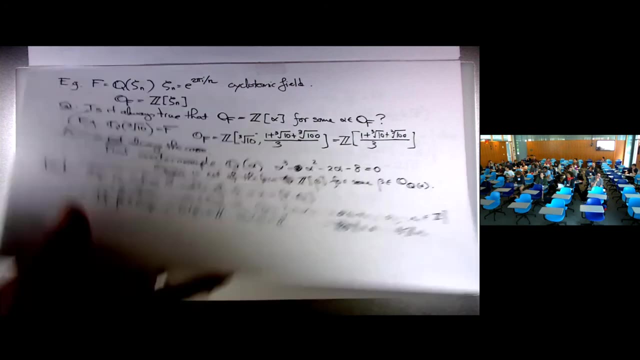 alpha n such that of looks like this In a fancy way. this All right, Thank you z excuse me. z alpha 1, z alpha n. So these alpha 1 through alpha n are the z faces of O. 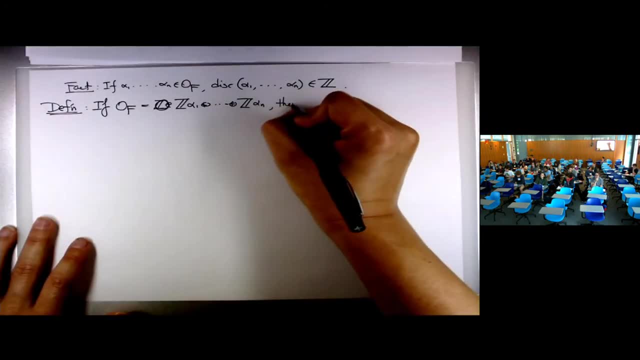 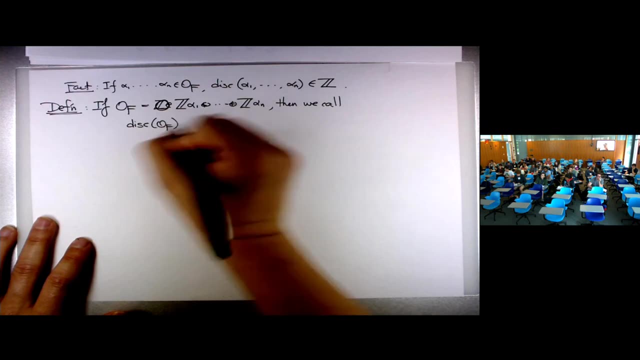 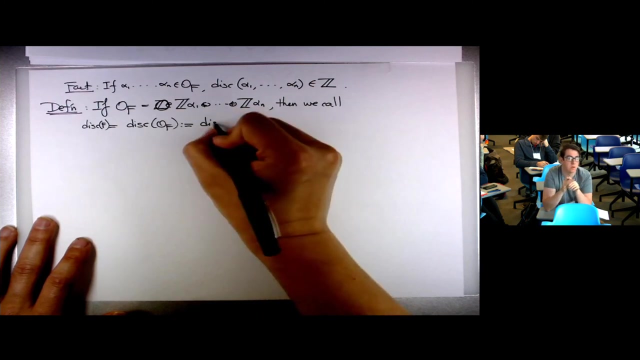 Now, if I do have this, then we call. I'm going to write discriminant of O or sometimes you write discriminant of F. This is defined to be the discriminant of alpha 1 through alpha n, as defined in the previous page. 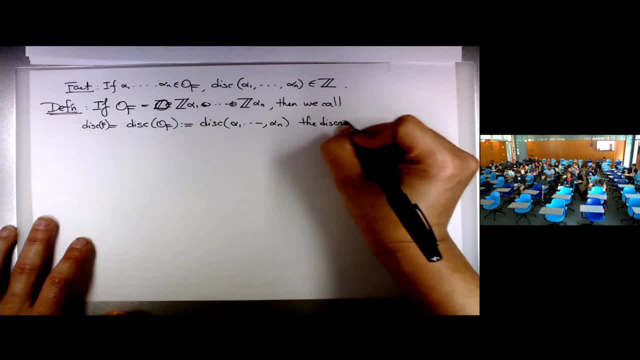 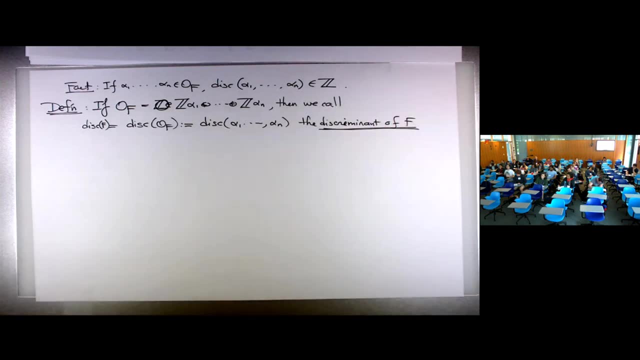 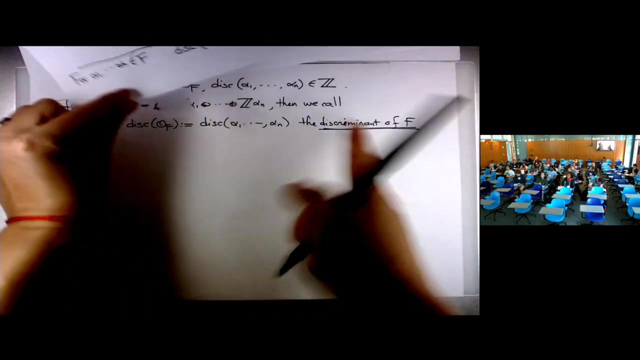 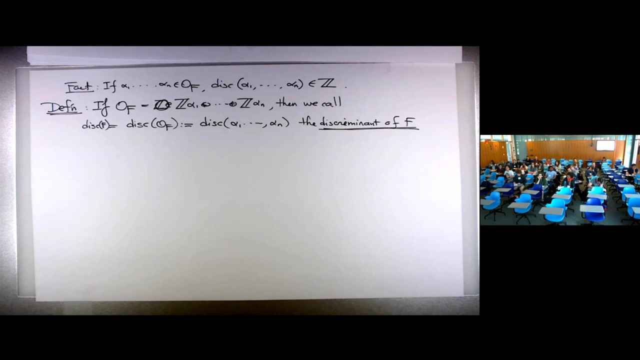 the discriminant. So this is a I think. I hope it gives you some sense of what this means. In terms of picture we had earlier, this means that you embed O into. this is sort of the n-dimensional space, the fundamental volume of that lattice. 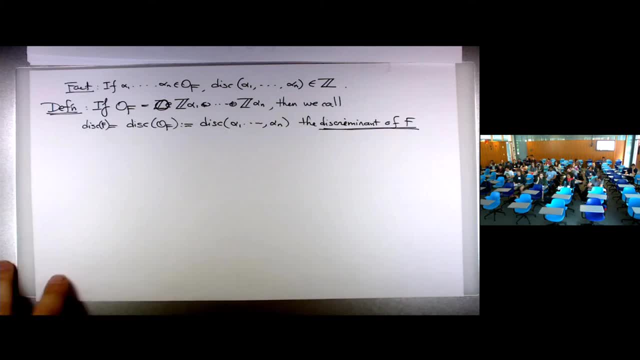 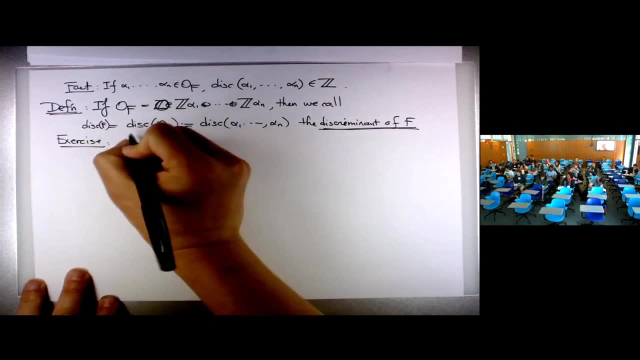 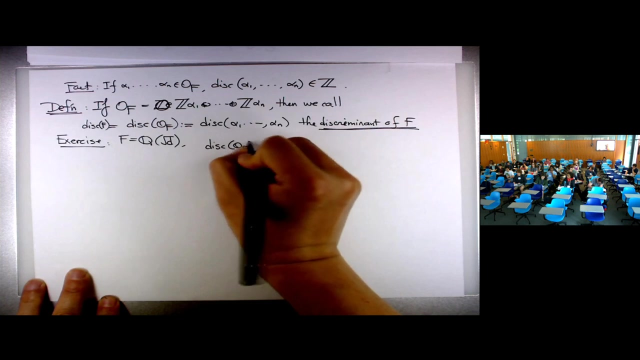 That's roughly what discriminant is. Just giving you some. this will be an exercise later. If you have F equals Q, a joint root of D, then the discriminant of O or the F is either D, if D is counted as 2, or 3 mod 4.. 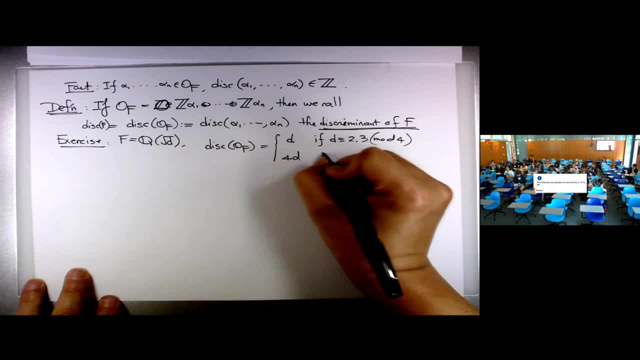 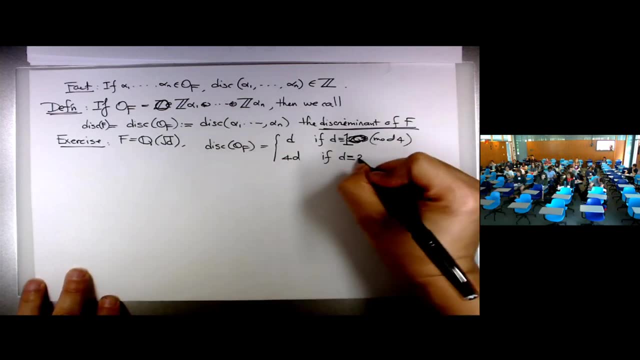 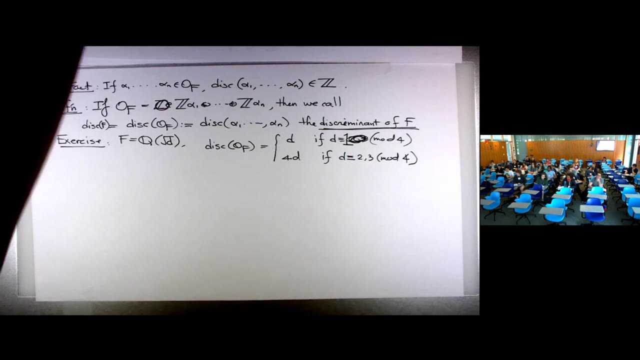 It could be also 4D if D is. oh sorry, If D is counted as 1 mod 4, it's D, Otherwise it's 4D, Sorry. Let me give you an example. So here, Q, a joint root of 5.. 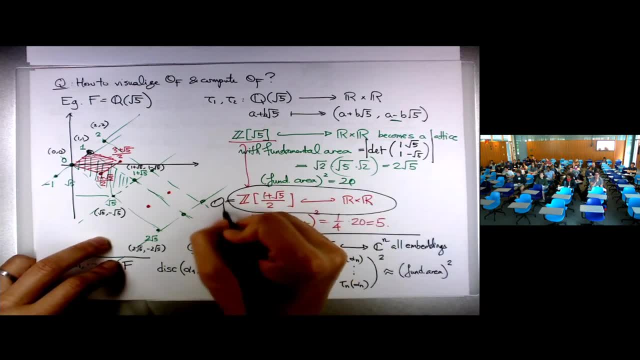 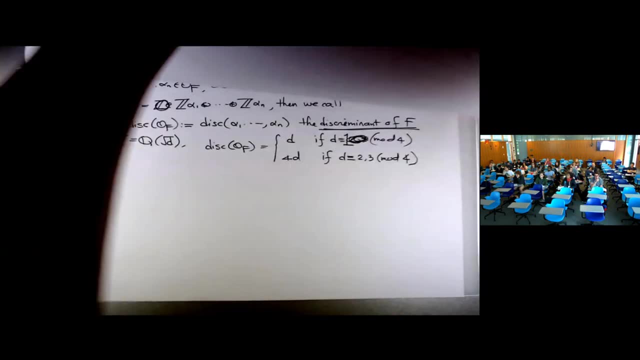 I compute the manual. This is really the O here, Then the square root. Put it on the table, Put it on: the area is 5, which is this: 5 here, root of 5.. That's somehow the first example we have here. 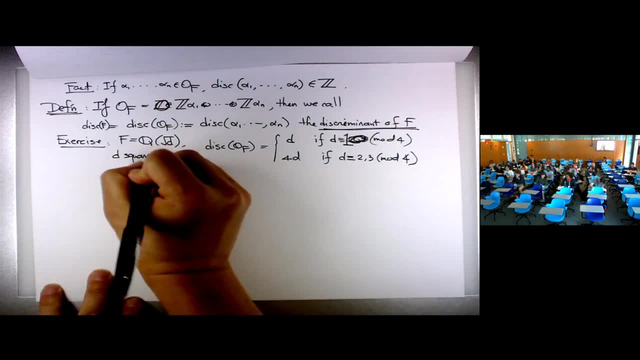 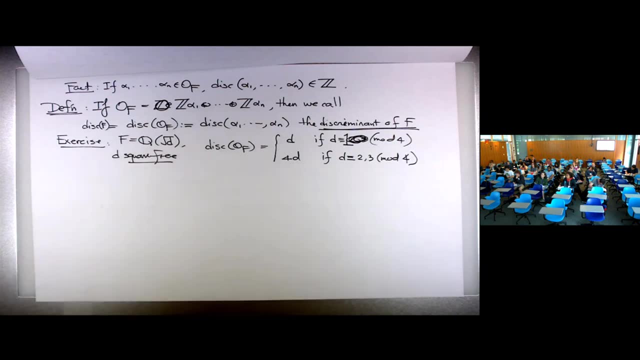 Oh sorry, I mean O is D squared of 3.. Whenever I read this, I mean D squared of 3.. OK, So I want to say that. the next thing is, I want to say: how is this discriminant? 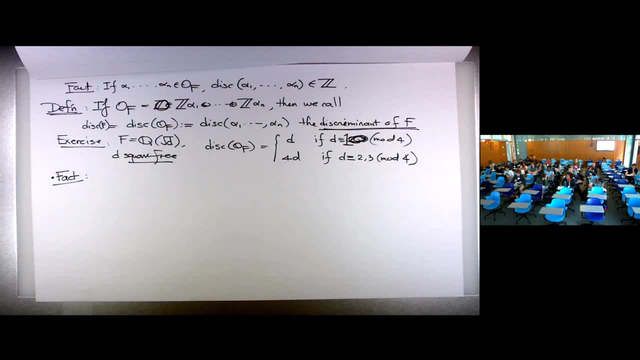 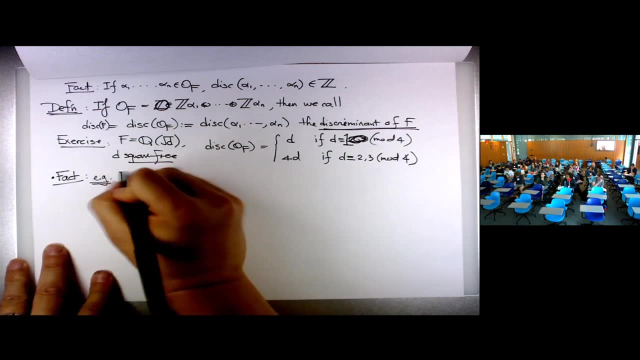 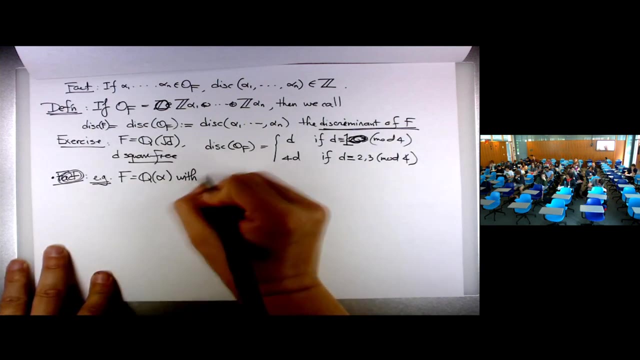 This construction can help us to determine what OF is. Here's maybe an example. Let me start with an example actually. So I start with F, Not fact. just an example F of joint Q alpha Where alpha specifies as x. alpha cubed equals alpha plus 1.. 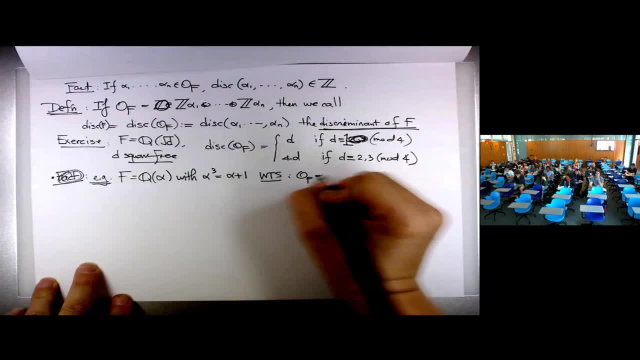 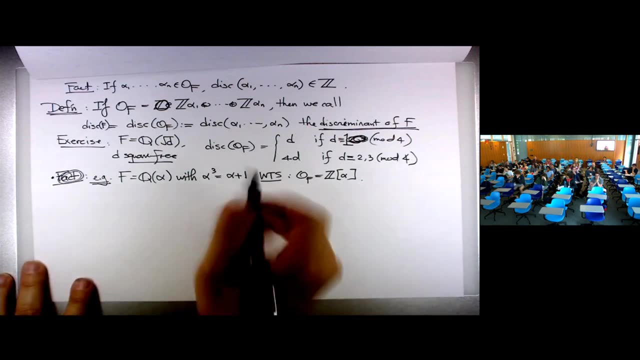 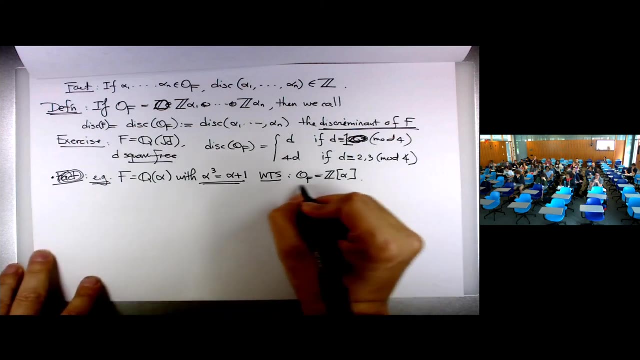 I want to show that OF is just z alpha. Of course alpha sets by this integral coefficient polynomials. Therefore it's in the random integers, But then I'm pretty sure there's nothing else, right? So here's what you do. 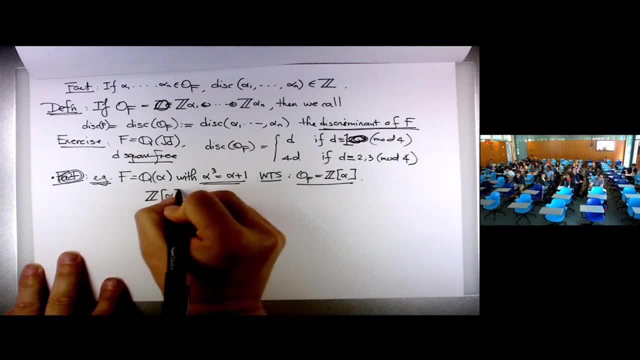 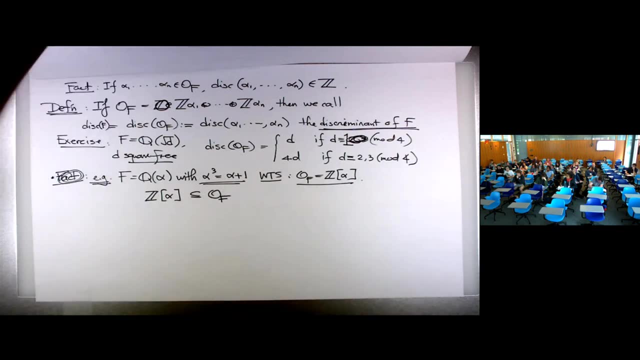 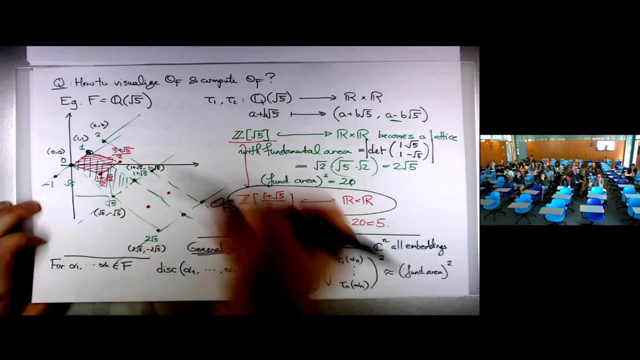 So you know that your z alpha is going to generate a sublattice of OF. OK, In the sense that you should kind of look at the picture here, Your OF is going to be the finer lattice here Your z alpha could potentially be the green one. 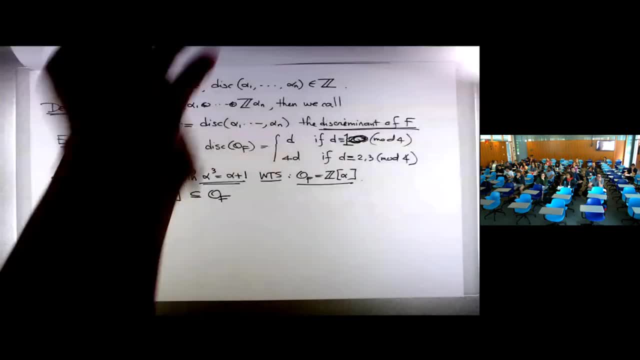 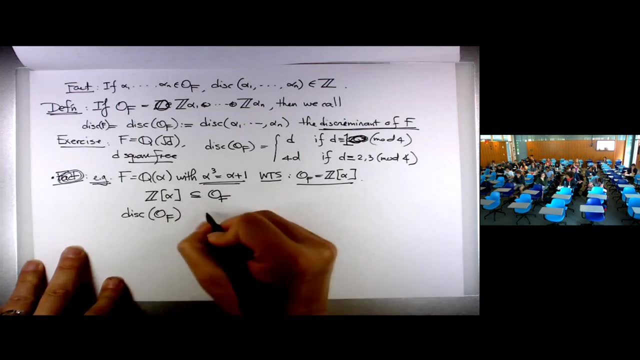 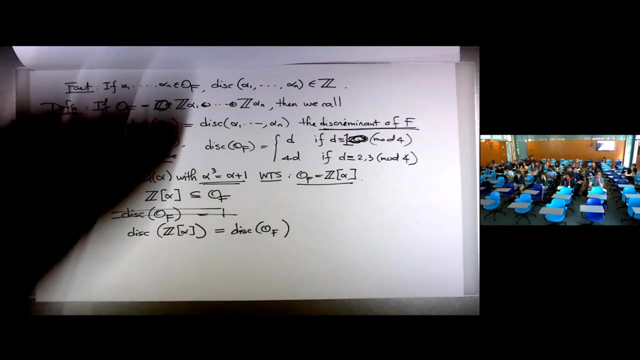 but missing some points. Right. And now, if you look at the discriminant of the difference of the two, if you look at the discriminant of the larger lattice versus the discriminant of the smaller lattice, if you see in this paper, in this calculation here, 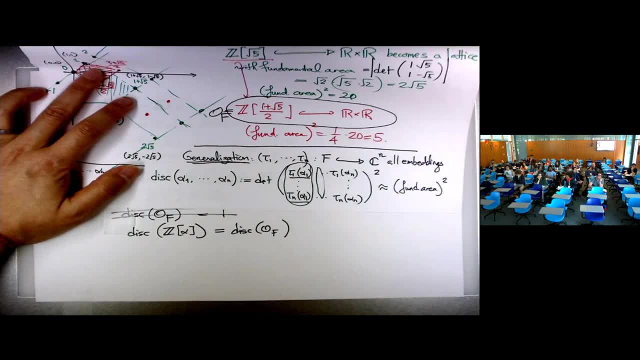 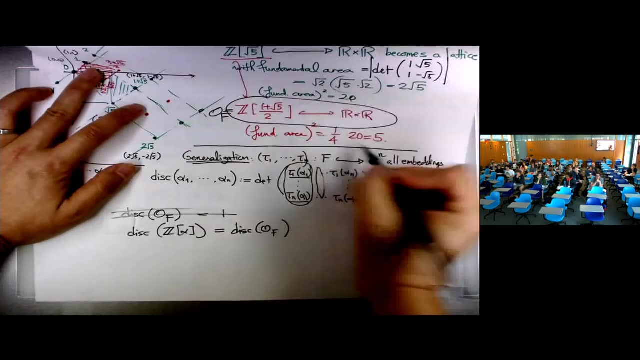 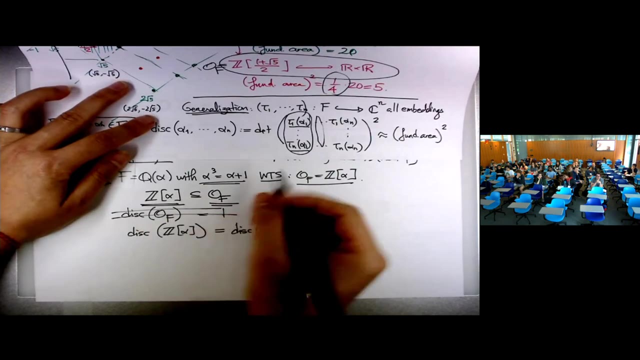 see, because the discriminant is really to think this is a square fundamental area. If the difference here in this case is 2, then the fundamental area squared will opt by a factor of 4.. So in your case z alpha is going to be a sublattice of OF. 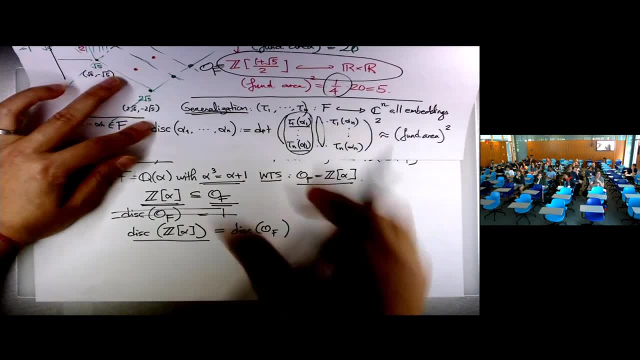 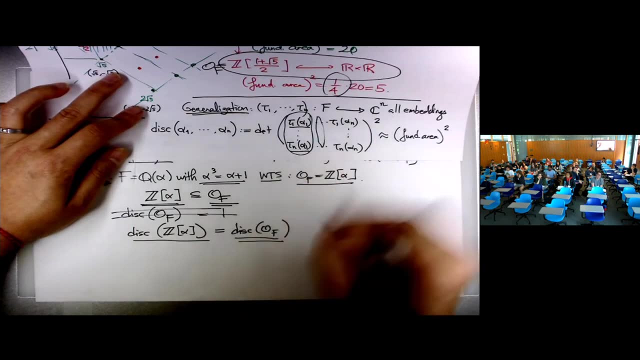 So in the sense that the green one, the discriminant, the fo- OK, So the green, the square of the green fundamental area should be the square of the red fundamental area. times some sort of the difference, but squared, Because our fundamental area is squared. 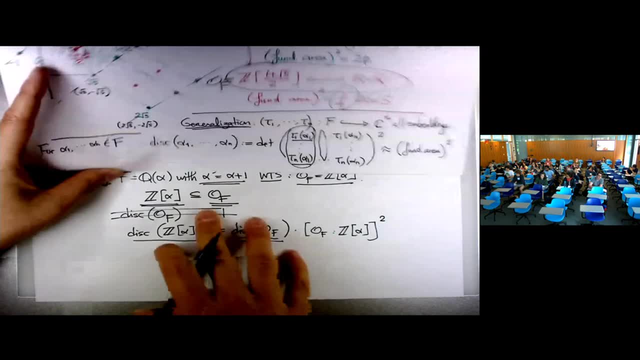 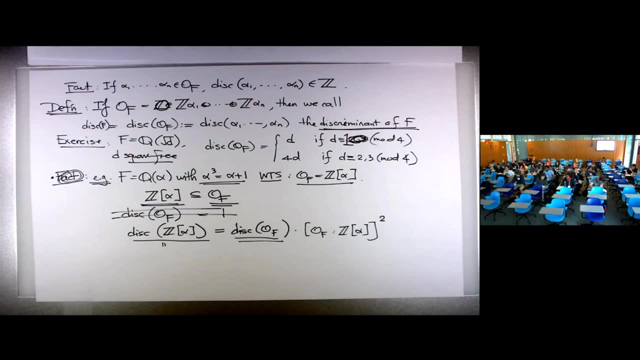 OK, And you can check that this one. this is some sort of a OK, Well straightforward calculation, but I'm not going to perform this, You just do. you have the standard basis, 1 ARP and ARPA score. 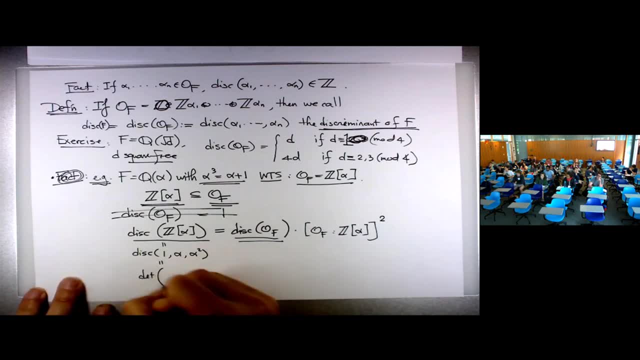 And you just really compute the determinant of all the embeddings: 1, 1, 1,. tell 1- ARPA. tell 2 ARPA. tell 3- ARPA. There's a better way to do this. I don't have time to do it now, but I'm just saying. 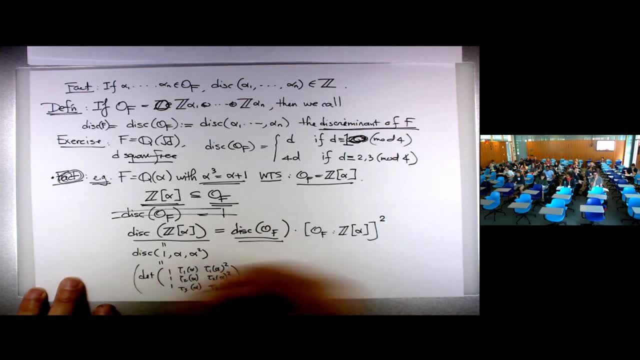 This is something you can compute. After a bunch of computation, you, you could, you could show that this is actually negative 23, if I got it right myself. OK, It's not that difficult, It's not that difficult. But now you're in this peculiar situation. 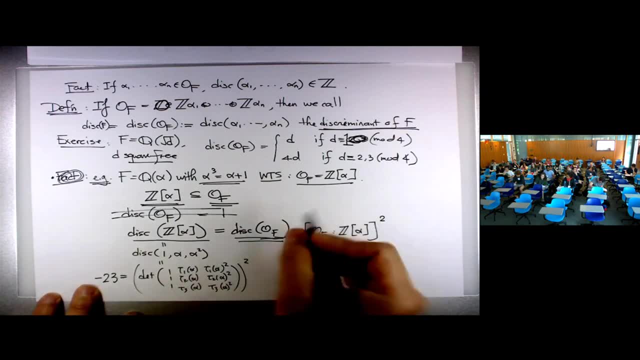 that the left side is negative transition prime. But we know that this discriminant O F is an integer And they're off by a square factor. But there's no square factor in this 23 here. So therefore this will force O F to equal to ZR. 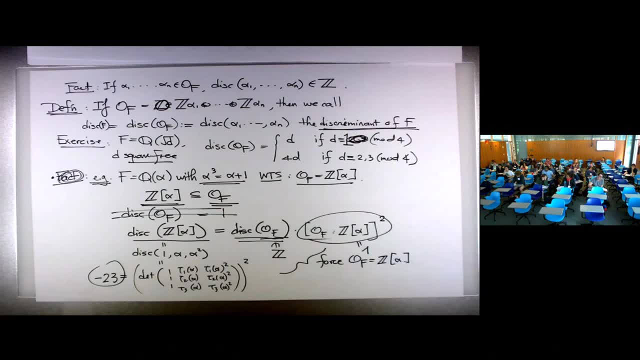 So force this factor to be 1. Because there's no square here. So that's how you use discriminant to help you to determine what O F is, in the sense that you first kind of approximate O F as possible, Like in this case. you would guess that somehow. 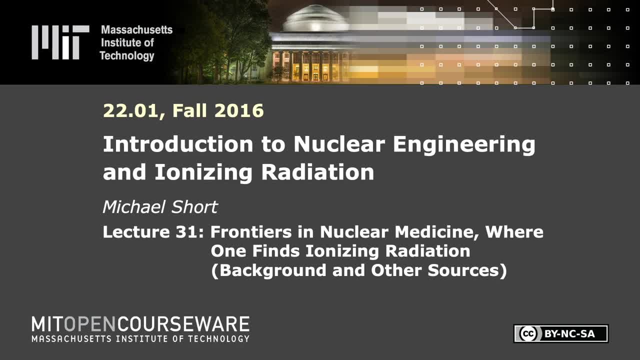 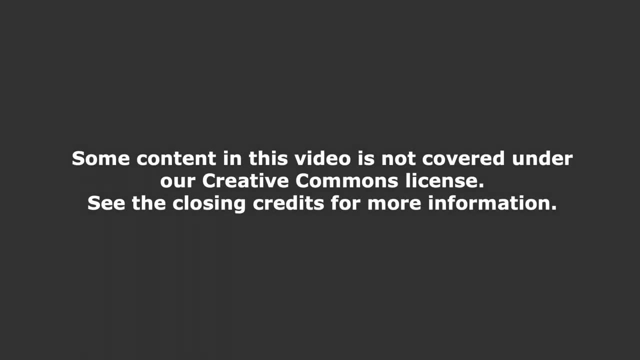 The following content is provided under a Creative Commons license. Your support will help MIT OpenCourseWare continue to offer high-quality educational resources for free. To make a donation or to view additional materials from hundreds of MIT courses, visit MIT OpenCourseWare at ocwmitedu. 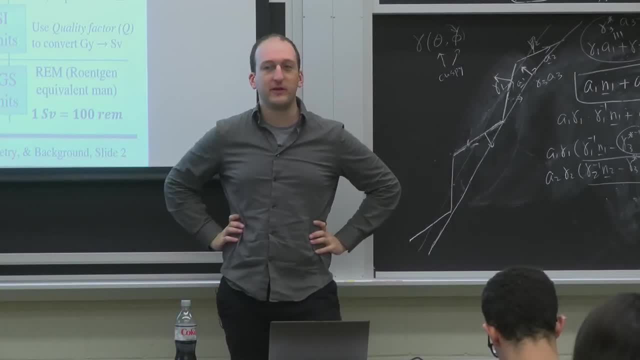 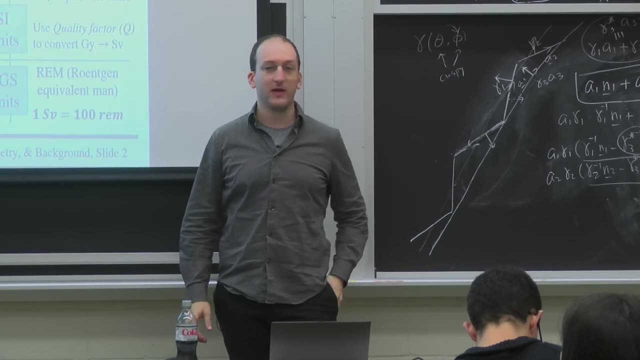 Hey guys, So quick announcement: We're not doing nuclear activation analysis today because the valve that shoots the rabbits into the reactor broke and needs to be repaired. So we'll likely just do this next Friday And instead we'll have the whole recitation. 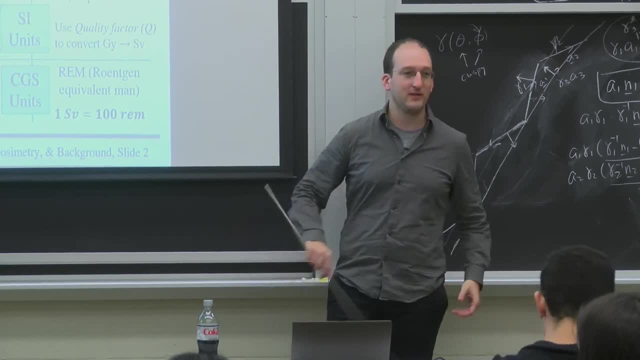 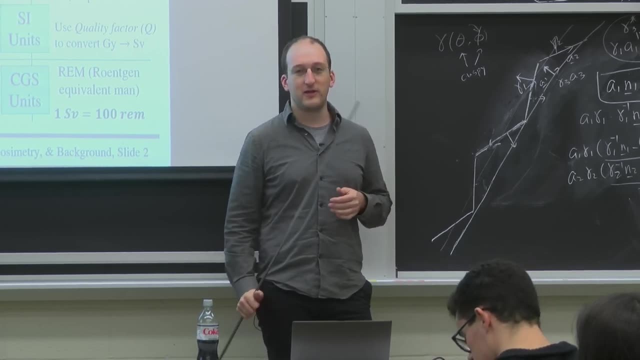 for exam review, like I think we originally originally planned. I also want to say thanks to whoever said: please write lecture notes for this class. It's something I think needs to be done, And I just now biked back from meeting with a publisher.